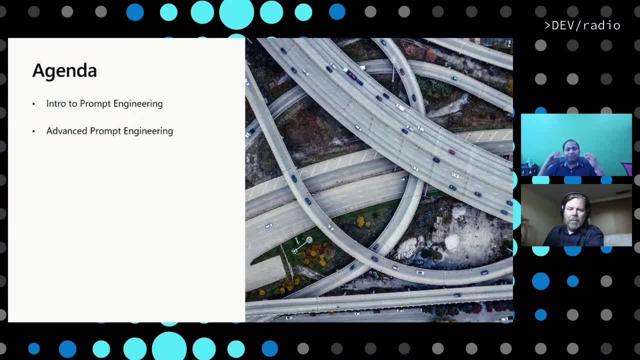 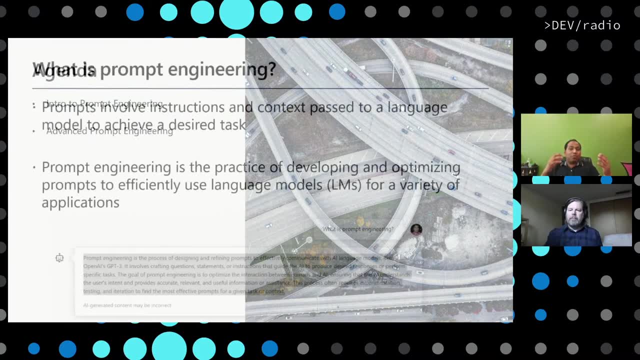 The intro of the prompt engineering and then we're going to dive deeper on the different tips and techniques of the advanced prompt engineering. Now, first of all, you know, first thing first, what is prompt engineering. So the prompt engineering, it's a very next. 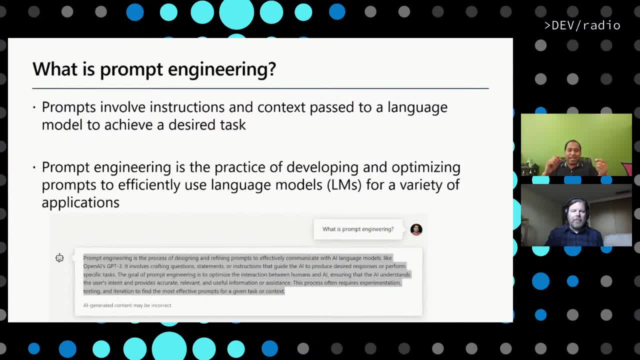 skill nowadays right And one of the hottest programming language nowadays is English right. If you know English better, you can write a prompt And the prompt engineering- basically the large language models, what instruction you are passing to the models and what output you want to. 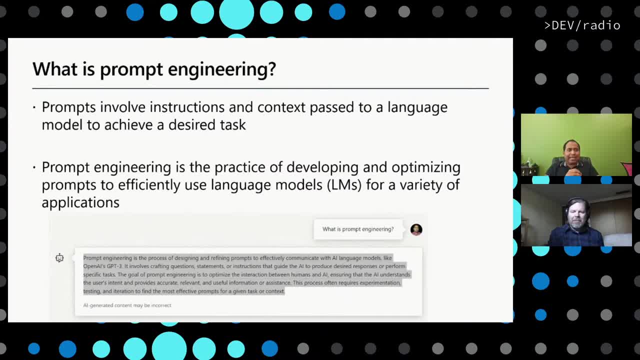 get out of the model. these are the two things right, and in fact, before i join this call, i just write my azure openai. what is prompt engine right? and this is the response i get- is that prompt engineering is the process of designing and refining from and effectively communicate with. 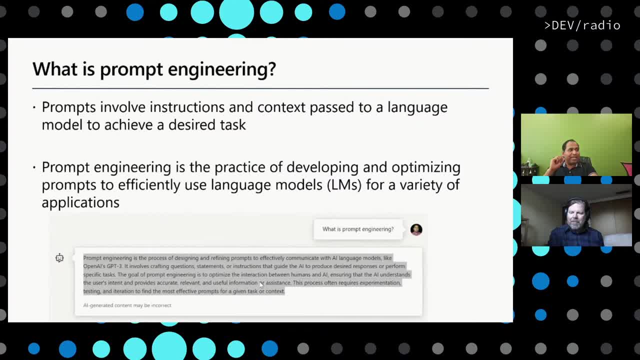 ai language models, so see that how it's like it effectively communicate with ai language. that's the reason i said english is the new programming language, so, like azure, openai, in fact, as you open ai, the gpd3 and other models, right, so involves creating questions, statements, instruction and 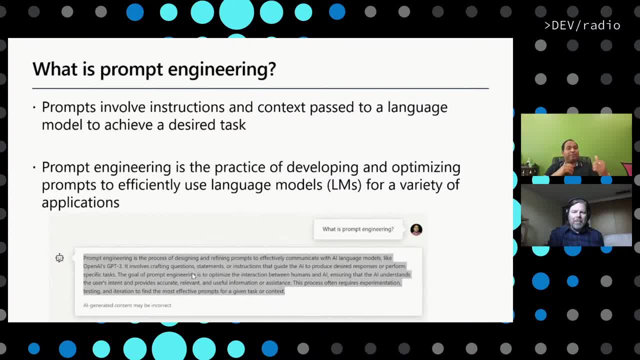 guide the ai to produce desired response and perform a specific task. the goal of prompting to optimize the interactions between human and ai, ensuring that i understand the user intent and provides accurate, relevant and useful information for assistance right. and this process often requires experimental testing, iterations and find the most effective. 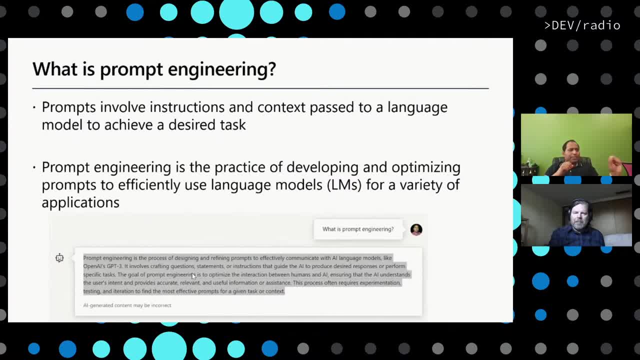 prompts for a given task or content. so just just put in a focus on the last statement. this process often requires experimentations, testing and iterations to find the most effective prompts for a given task or content. what does it mean? prompt engine? last words, it means prompt entry. 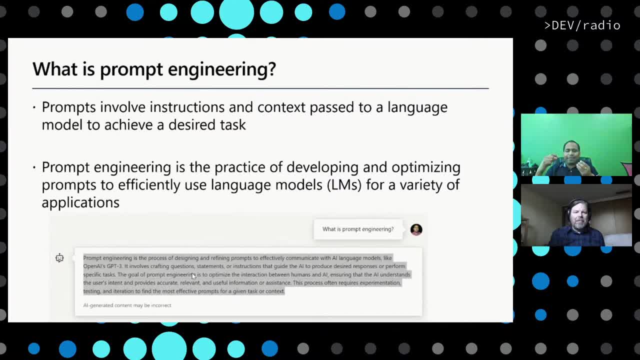 one, two, three. cool is note to see how come, when we have some functionsért, that's complete. remember, just before we apply some functions. worse, this is seed and mp. and the answer to this is: hey, oh, write. you should write once on the Harley own, once it. it's an iterative process. nobody can say that this is the best prompt. 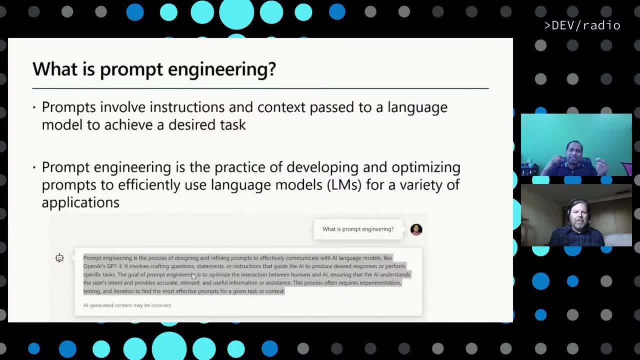 ijk ちら and secondary, what it helps us to give this to the model. no, the prompt you write. a prompt means that instruction given to the model. you get back the response, response and you see that how the response is coming up from the prompt and you may try to a little bit change the prompt and see what's the. 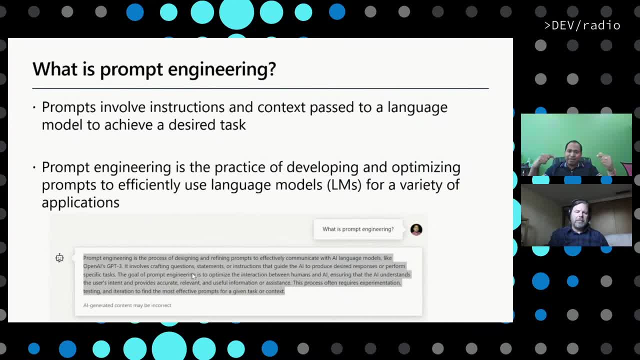 response part. so it's an iterative process. keep on continuing doing it to give you better and better and better results. right, and there is no certain point i can say that, hey, this is the, this is the point you should write the prompt and this is the response you should get. no, it's all depends what, where you feel that. 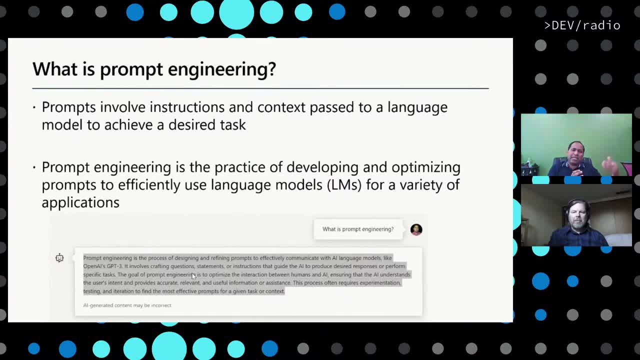 this is the best output you are getting and that's where you can stop it and you can keep it ready to give more and more better right. that's need to be remembered. so, in short, the prompting is a pro. it's kind of a process- eternity process. you have to keep on writing. 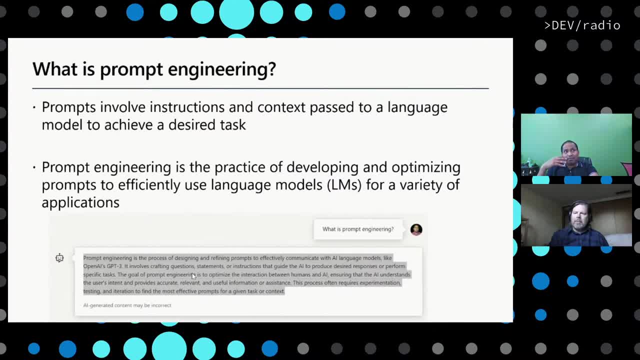 giving you the better response, and that's in fact i'm. i'm seeing the future. the prompting will be one of the very next skills in the coming era of generative ai, which people has to adhere as part of their other skills and without that skill, i think the scope of your application to giving 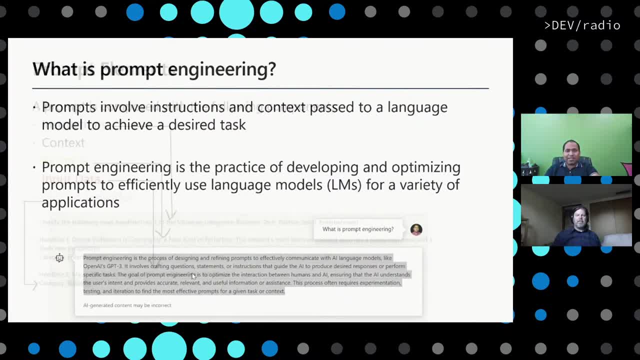 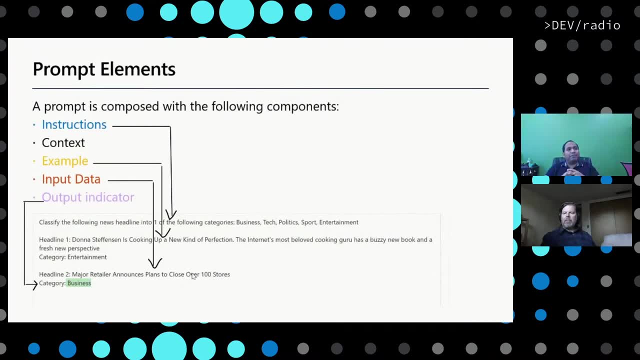 sophisticated, will be much, much, much more hard. okay, now we're going to go to the next slide. we're going to talk about some basic things before you go to the advanced type of the prompting. first of all, what are the different elements of props? right, so i in the town, i have provided 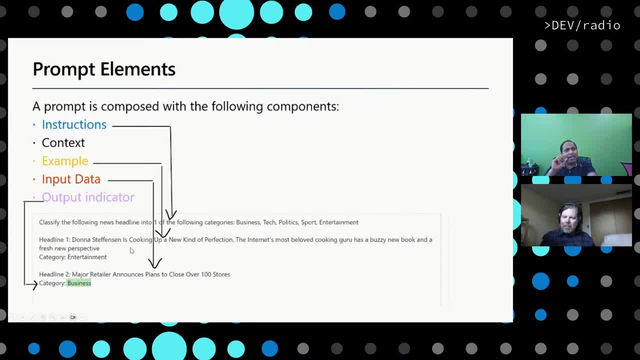 uh, examples of a particular prompt. so typically a prompt has um around four to five and the reason i said four to five, some some prompts, you'll see that four, some problem could be five uh elements are there. one first thing is instruction. means that this, if you see the example that i classify, 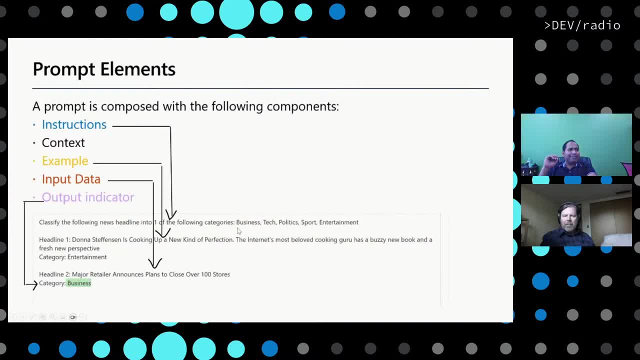 the prompt, you will see that the prompt has four elements and the prompt has five elements. so if you look at the following new news headline into one of the following categories: business, tech, politics, sports and treatment, this is the call instruction. so you are telling the model what. 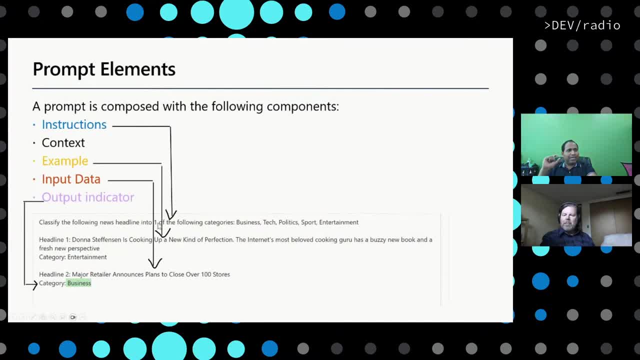 the model has to perform. that's called instruction right, and then i'm going to come to context later. but then we are giving some examples. for example we are giving here- don't ask to come- is cooking up a new kind of perfection. the internet most um beloved cooking guru. the internet most um beloved cooking guru. the internet most beloved cooking guru. 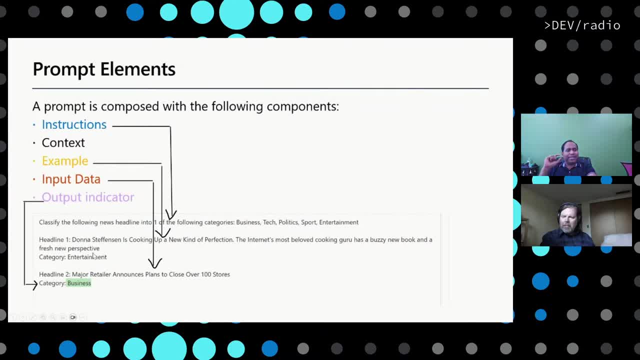 as a buzz new book and a fresh new perspective. and the category you did it's doesn't that by the model? you did say it's an entertainment. so this is an example. you are feeding to the model along with the instruction- right, that simple example. and then you provide your new input. data means now that is. 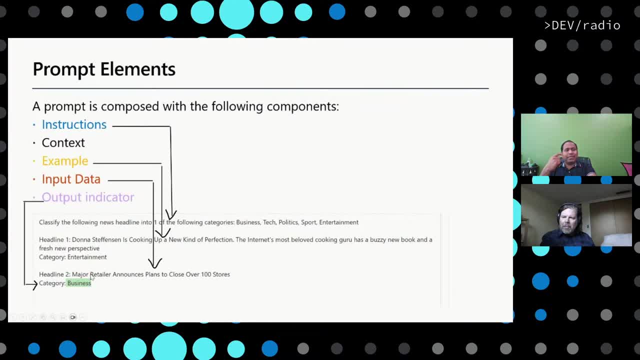 the kind of a question you are asking, to model, to predict what would be the category for this particular particular statement. right, that's called input data. and then we have an output indicator which is just a category, not the green part, just the, the, the, this particular the black letters category. 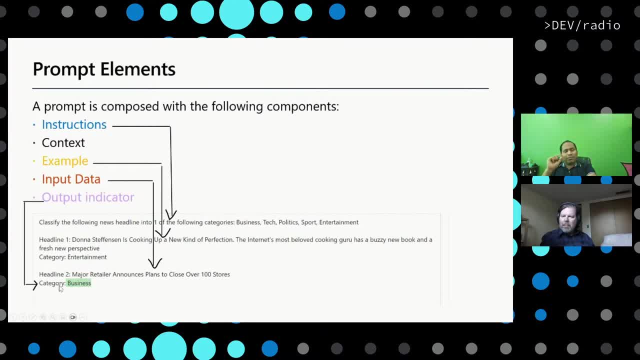 that's an indicator. you are telling the model. okay, you want to. model has to predict the actual category of this above statement and come up the results in the category tab right and model predict it. it's a business which just seems to be correct, right? so instruction, you are telling. 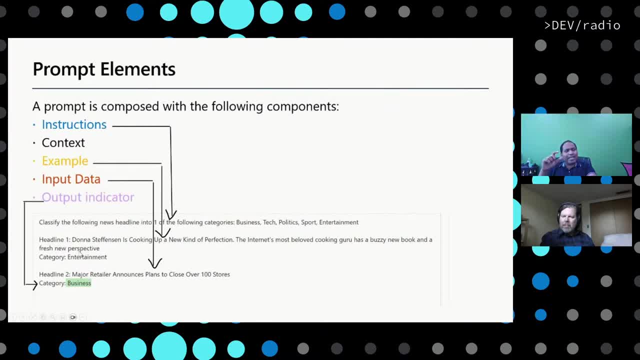 model about you to perform examples. you are giving some examples to the model so that model can steer towards particular uh examples and give you the actual result for your actual input data and input output indicator. now we'll go later about some other techniques, about you know detail but this: 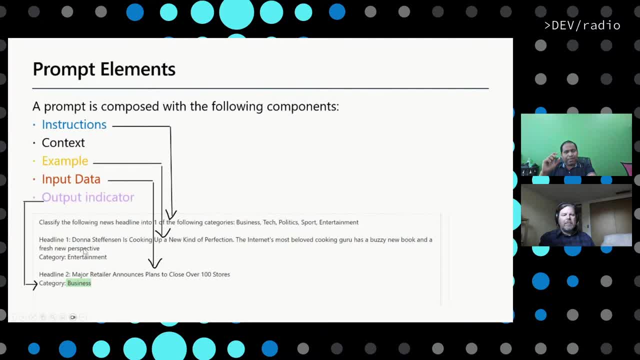 examples is not necessary you have to give. every time is very good to have, for sure, but even if you don't provide that example, that's okay. um, it can produce you the results. will not judge about the quality right now, uh, but it is possible without having an example right now. I haven't touched about the context part. the context. 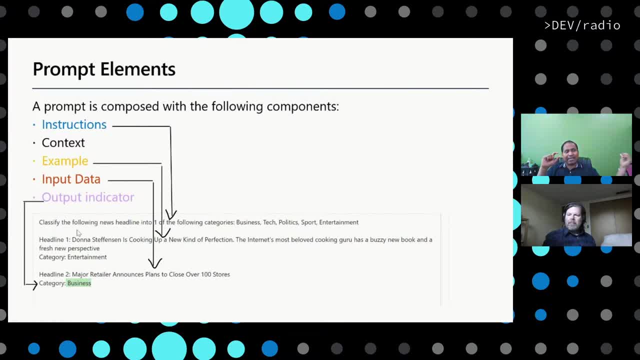 is also important in some cases. we're going to go more deeper on that time. we're going to talk about the context piece. but the context, think about, you are producing a question answer for your given text, right? and then your, the given text is become a context, right? so you said for. 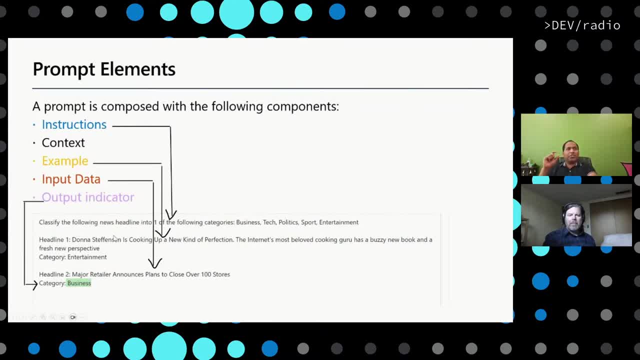 example, you tell the model that, okay, your job is to find the right answer from a given questions by the user for the given text. right, and then you provide the text and then you embed the whole texture. right, that text become the context at that point. right, we're going to go to the example and 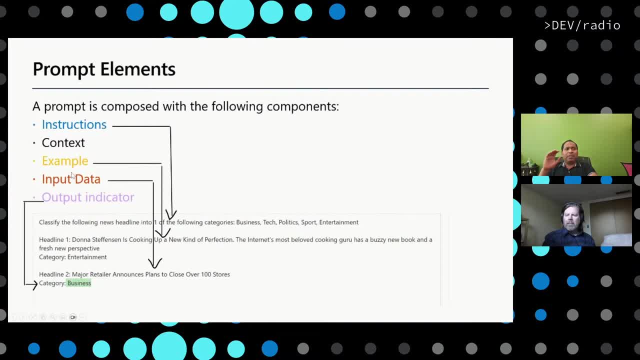 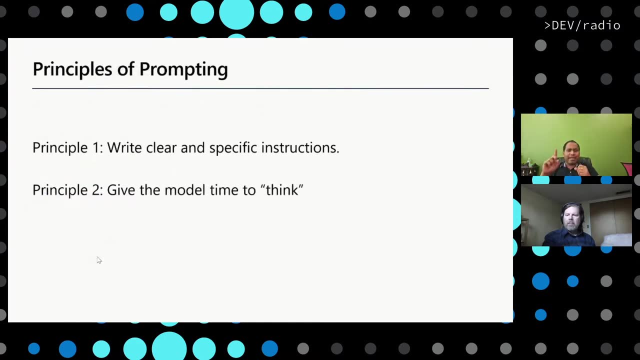 it will be much more clear. but typically instruction context example: input data and output data- these are the element to define a particular problem. now let's go. different principles of uh the prompting. the principle number one: you always write clear and specific instruction. principle number two: give the model time to think. same goes. 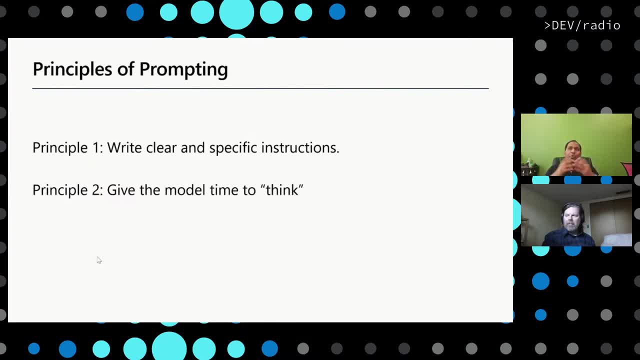 by the human. if I ask you to do something and if I don't give you a specific instruction, I will not get the desired output from you. right, it's a pretty human and at the same time I have to time to the person to think before the answer. right, it's pretty. 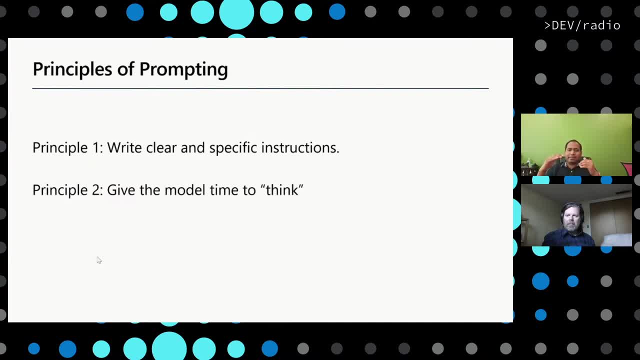 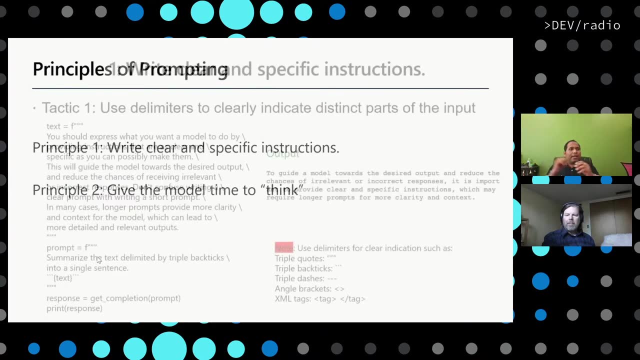 simple thing: I need to tell you what needs to be done and then I also need to give you time to think before you response back to me. these are the two principles. applies for prompting for a large language model. pretty easy. now principle number one: we said: write clear and 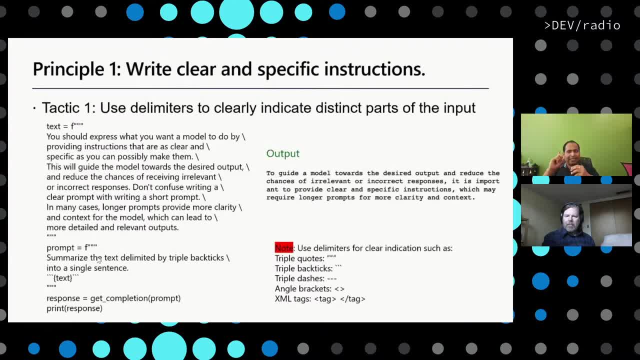 specific instruction. now, what are the different tactics? for that? tactic number one: use delimiters to clearly indicate distinct part of the input, right. so here you see that I have a given text and I have in the f string. I have provided the text and then I have telling the actual. 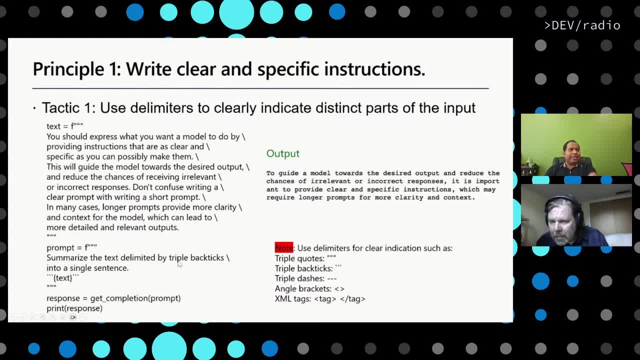 uh, which is an instruction: summarize the text delimited by the triple backticks into a single sentence. right, it's a pretty clear in the uh and specific instruction what white is clear because I said summarize the text delimited by triple back. so a very clear what need to be need. 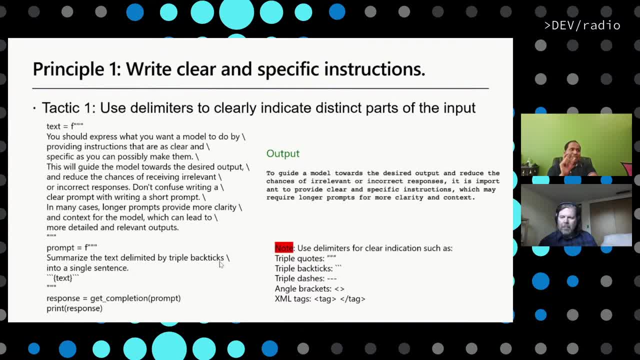 to be, uh, used to to, to summarize that statement right. and then I'm saying into a single sentence: that's a very precise instruction, very clear and specialized instruction now in the text- and, by the way, I'm just sometimes fishing in that screen and doesn't mean that I'm doing something different- 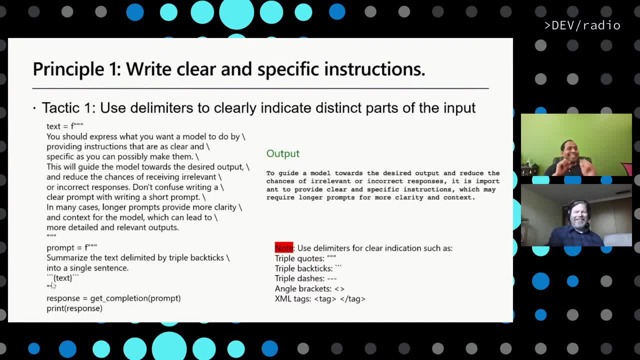 because I would do it anyway. look at that here. so here in a, in the text that is kind of a variable and in the backtricks which I put it here, that text is basically: this goes here, right, and then I'm asking to summarize in a single sentence, and then I'm getting the response and 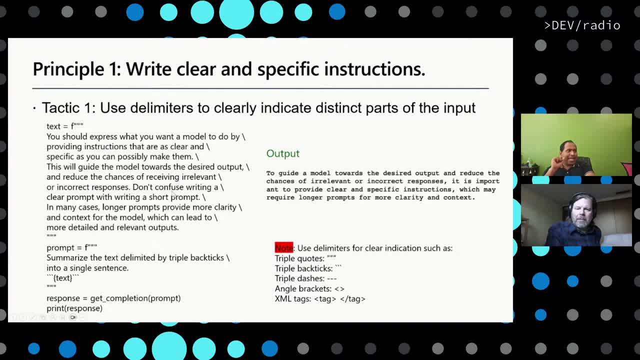 response and the output comes based on this particular text, the guide to a model to us, to a desired output, and reduce the chance of iterations or incorrect responses. it is important to provide clear and specific instruction, which may require longer prompts or more clarity and context. right now, people sometimes think that, hey, is it a back to side, always need to put or there. 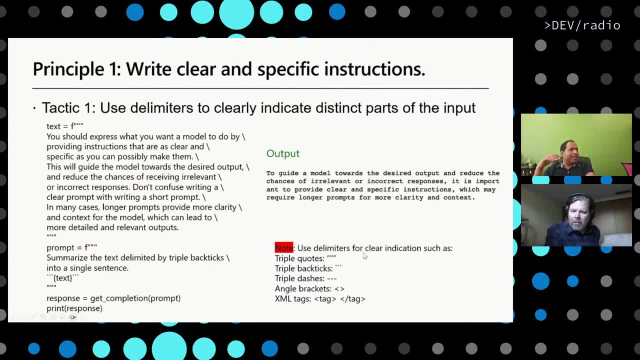 is some other technique. no, it's not back to us. it could anything and there are some examples. i have put it. it could be a triple quotes, could be a batteries, could be a dashes, could be an angle bracket, could be an xml tag, could be anything right which can't. 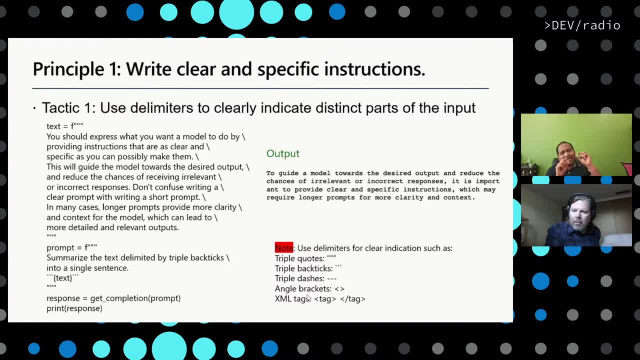 separate this out, which can understand for the model what is where exactly the test goes. that's why you need to separate it out and you give a very specific, clear instruction what need to be done. so i hope it's clear. the tactic number one. now we'll go to the next act. tactic number two. 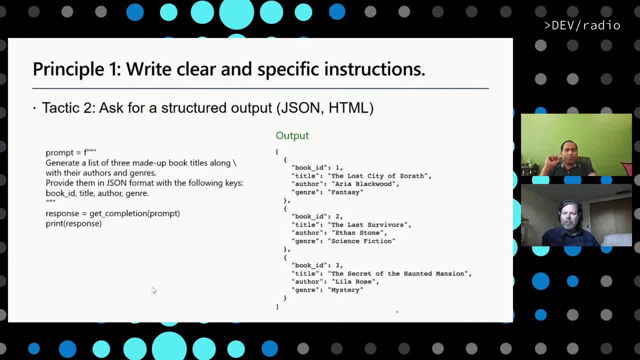 always ask the model to produce a structured output. right? if i ask you a question and if i tell you that at the same time to answer, you need to response back to be a bulleted list, that means you're gonna not gonna read a paragraph to me, you're gonna read me a bulleted list, same. 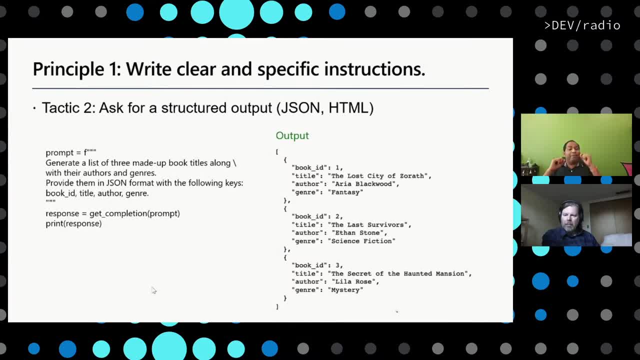 thing goes to the model. if i ask the questions to the model and if i want the model to response me better, i'm going to ask the question to the model and if i ask the question to the model, back to some structured output could be a bulleted list, could be a json, could be an html. 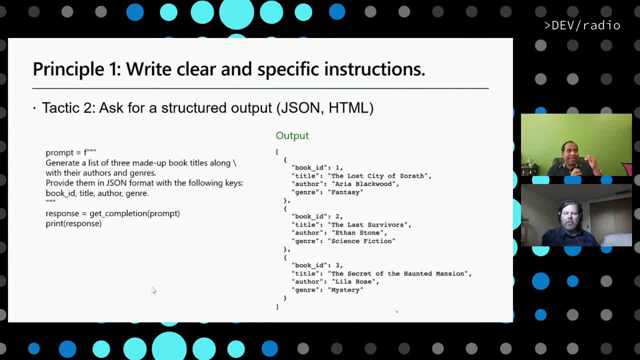 could be anything right that has to be clearly mentioned in the instruction. so always you need to make sure you have a structured output, and see this example in the prompt i said: generate a list of three made up book, title, song with their authors and genes. provide them in json format. 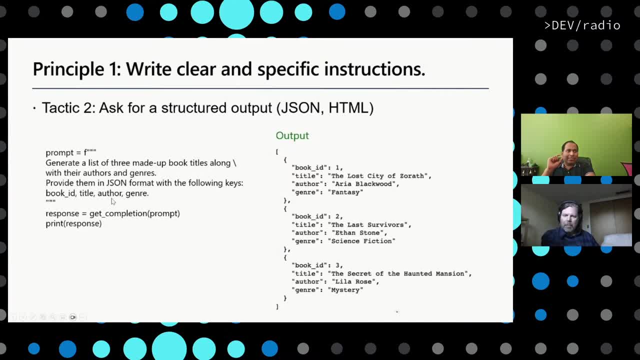 with following keys: book id title: author: jenny, see how clear that not only the instruction, but i'm also telling the output has to be a json tag right. and these are the keys of the json and if i run that one i get a json output right. and 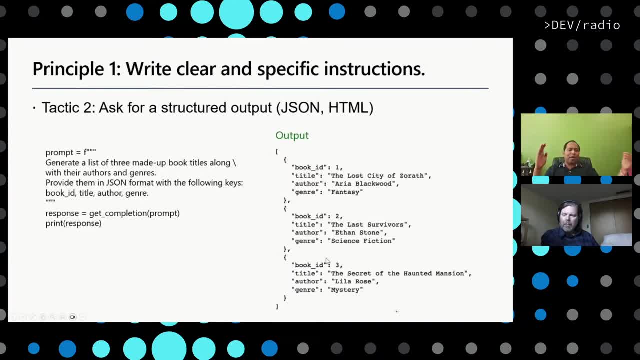 this json things. you can take it, and you know, post process for your downstream applications, which could be much more benefited, rather, if it, let's say, responds back to kind of an in a one sentence right, which sometimes again you have to post process with some other techniques, but it doesn't. 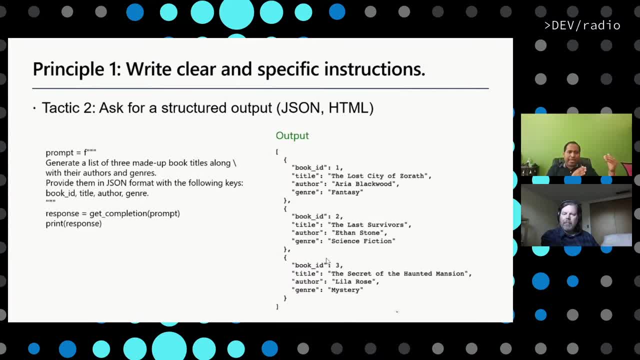 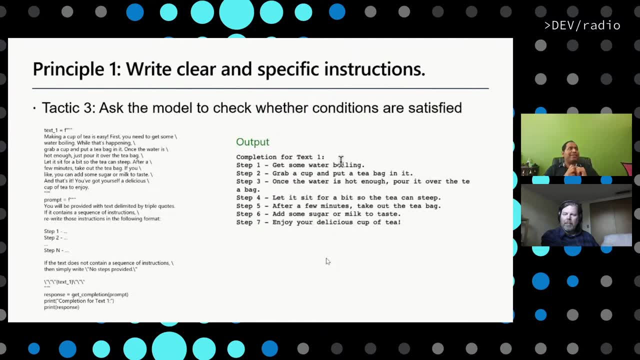 seems to be good right. so always you need to have a structured output in your prompt instruction. third, ask model to check whether conditions are satisfied. very important tactics. you need to remember. this is very important and we're going to dive deep more in the subsequent slide. why this? 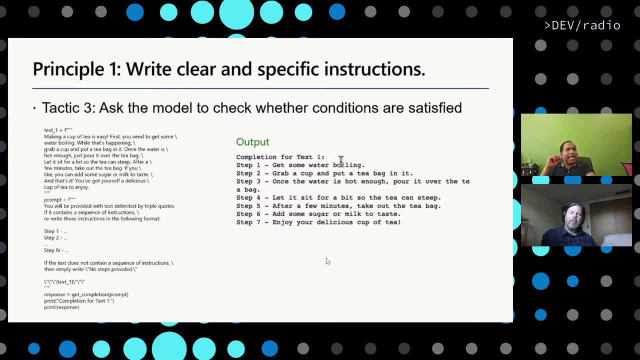 is important, right, but this tactics is helps you to give you the right answer. same goes to a human: if i ask you a question and i want you to give me the right answer, then you can give me the right answer. so only you need to submit it. Emiler, we going to ask you to get the questions correct. 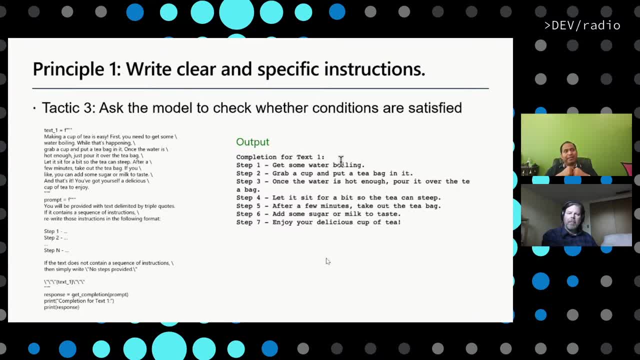 once again, you need to validate the fantasy. some of you probably don't want to accept this because you are not a human, you are just an attacker. before you answer that question, make sure you validate all the conditions are satisfied before you respond back to the to me same thing here. 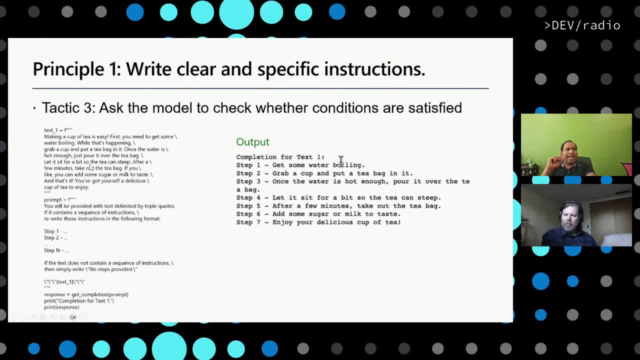 i'm making a prompt here. i'm telling that making a cup of tea is easy. first you need to get some water. warm tea for tea: Hillsaze, Review the chat. for example, if you are having a hot coffee while you might want to photor an ad in your tea bag, now just prone it over to the tea bag for a normal magic contract. before you answer the questions, make sure you validate all the conditions are satisfied. status: child. before you respond back to the to me simple thing here, making a prompt is easy. first you need to get some water- water boiling while that's. 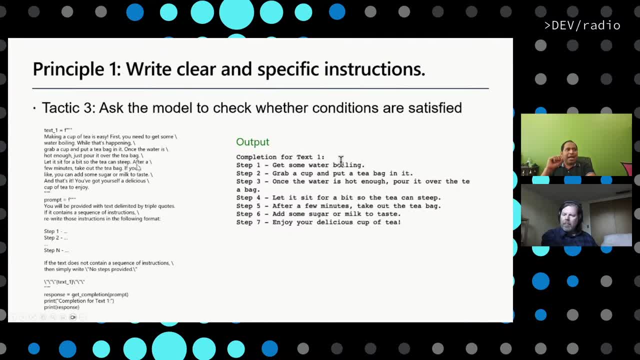 and then take a step after a few minutes, take out a tea bag. if you like, you can add some sugar or milk for test, and that's it. you can go to yourself to a delicious cup of tea and to enjoy. in fact, you know, after reading this one, I wish I could have a cup of tea, or coffee anyway. um, yeah, so and see. 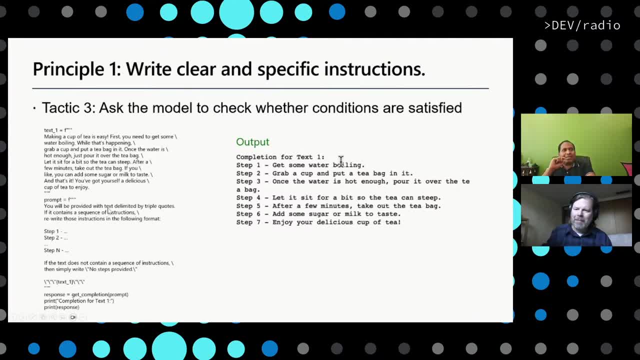 this is my text, right, and in the front I'm saying that you will provide you the text with the recommended by backtricks codes, right, if? if it contains a sequence of instructions, rewrite those instructions in the following format: step one, step two, step three, step four. go to the step. 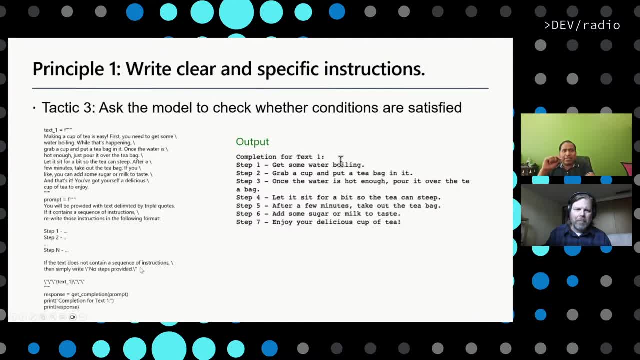 end, and if the text does not contain a sequence of instructions, then simply write: no steps provided. see, then I'm putting within the back is the text and then asking the output. right, and here is the output. so this output, step number one. step three was the water is hot enough pour it over the tea bag. step four: let's set it for a bit. 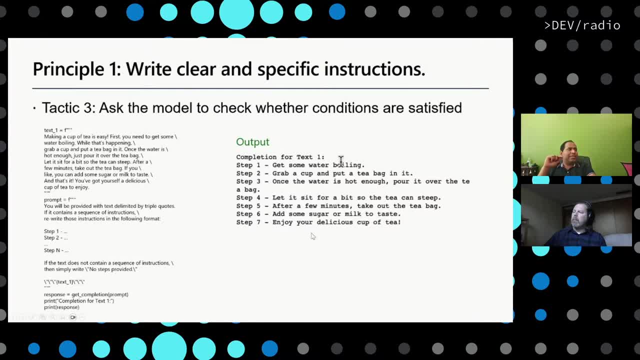 the tea can strip. step five after a few minutes. take out the back. step six: add some sugar or milk for test. step seven: enjoy the delicious cup of tea, correct? so this very sequential steps how it came up, because we tell the instruction, the prompt, that you need to rewrite that instruction in the following format: 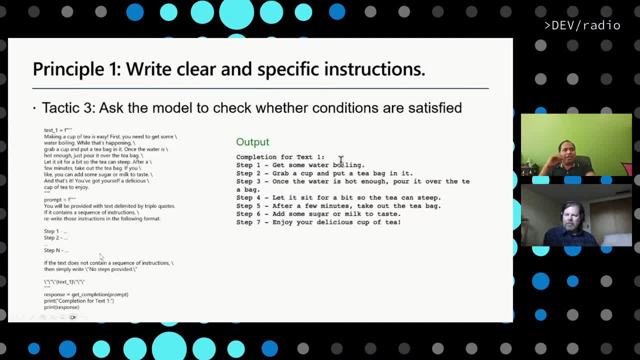 right. and if this test does not have any sequence, there's a no steps provided. so before it affects the actual output, the model itself goes and make sure all the steps are validated as satisfied. and because you see there is there is no no steps provided no steps, I mean there is no such step. 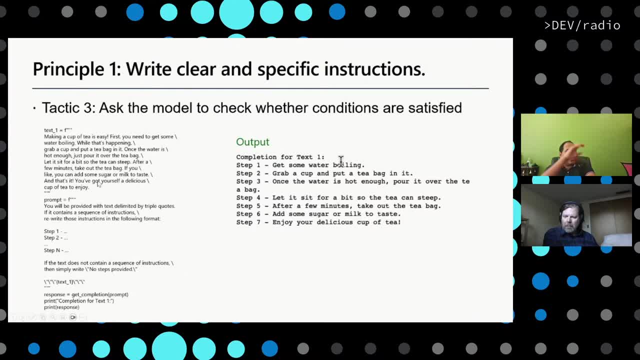 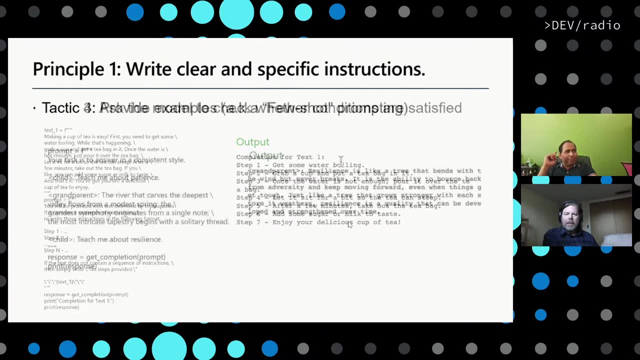 eight or something like that: says no, no steps provided, because it's validated and it makes sure to make a tea, whatever is required. the steps is all is there and that's interesting. I hope it makes sense. yeah, yeah, let's go to the tactic number four: provide example. that's what I said beginning. 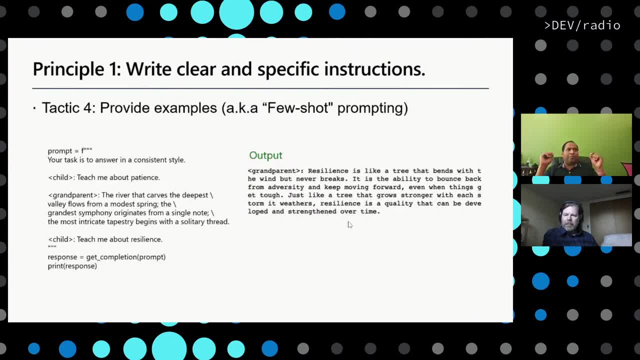 right example is very important. it's also known as few shot prompting, right. let's take the same human analogy: if I ask you a question, right, and if I do not provide you the examples, you can give me the output for sure, but if I give you an examples, right, hey, this is my question. these are my examples. 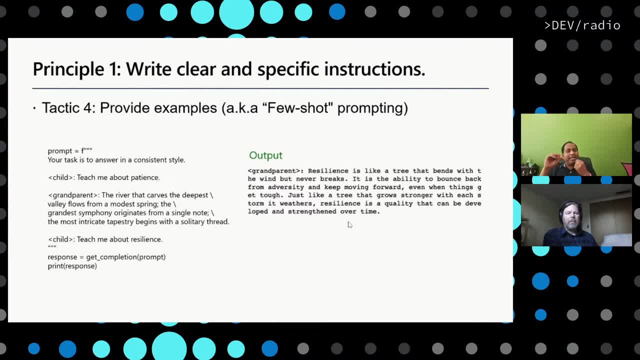 then it's for you it's very easy to understand, very easy and fast way you can compute in your mind what exactly I am looking and you will give me the results right. same goes by the large language. you have a prompt. you provide some examples. for example, here your task is to answer in a consistent 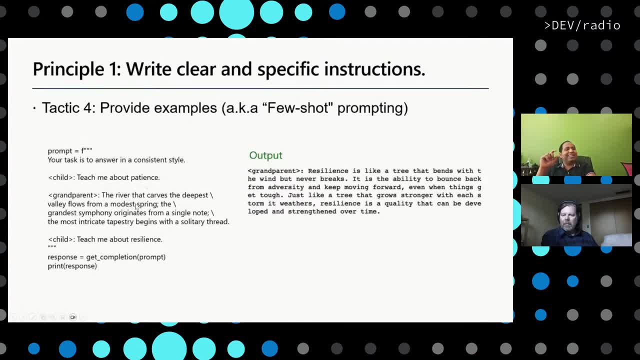 style child is asking: teach me about patients right. and the grandfather is responding: the river that creates the deepest Valley flows from a modest spring. the trend is simply Origins from a single note. the most intricate transparency begins with the solitary threat. these are the examples that father is given. 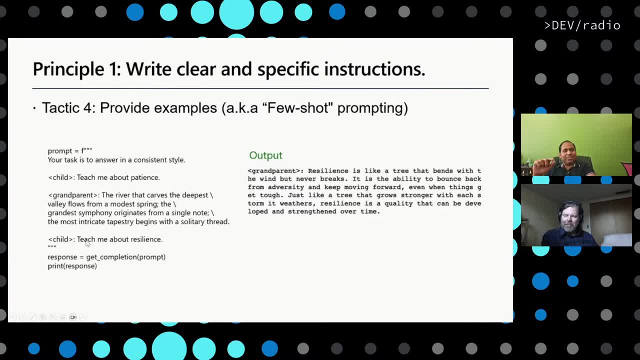 teach about the patients. now the child ask another question: teach me about Resilience. right and see how the grandfather's respond. bridges is like a tree that bends with the wind but never breaks. it is the ability to bounce back from the adversity and keep moving forward even when things 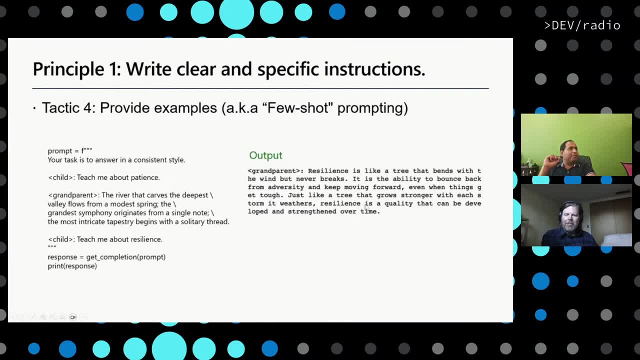 um, things get tough, just like a tree that grows stronger with the each strong it withers. Resilience is quality that can be uh developed and strengthened over time, so this uh kind of a Shakespeare oriented literature is coming out of here. right, it's pretty much matches the way I have given this example, so it's important. 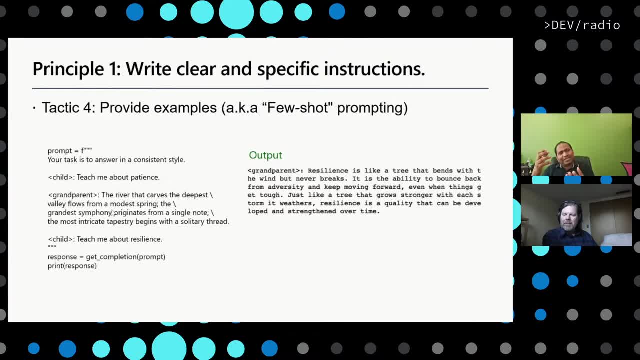 the tone which I'm expecting I provide the same tone in the problem. so it is important, uh, to give you the right response in the right tone, which is called future prompt, and if you don't provide the examples, you will get definitely what is Resilience means, but may not be the same tone. right, if you? 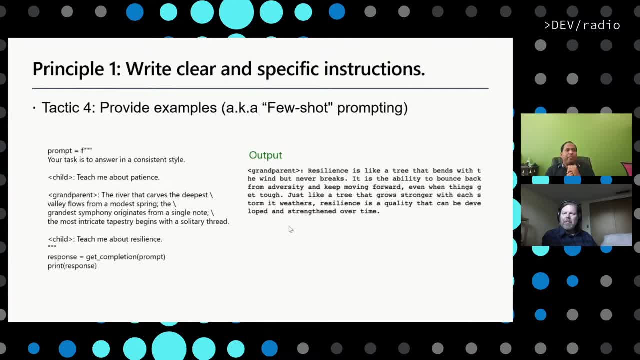 will get the answer right. that's called zero shot. prompting means that you do not provide any examples, but you still get an answer which could be satisfactory for you. and uh, that's, you know, that's okay. I'll not say the best, but that's okay. some applications, but not the best for the getting. 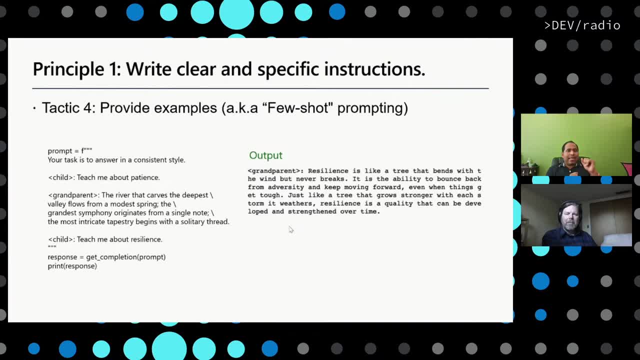 the best. you need to provide some examples. always do that, um, and now I'm gonna, and again, uh, these are four tactics I listed. it's not the all right. that could be many, many tactics like that. these are the very common tactics you can employ into your applications. 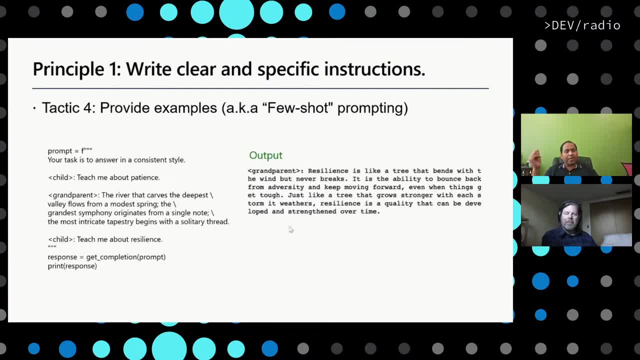 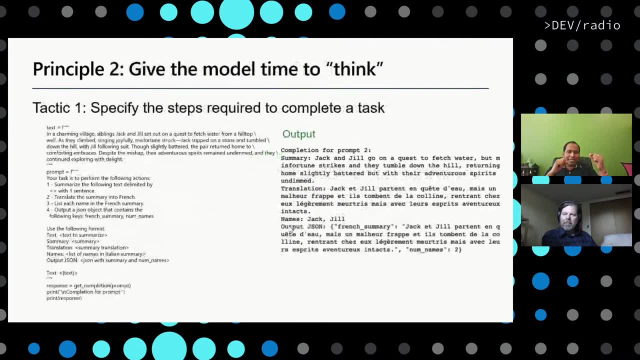 to give up a better output or do a better prompting GD. now I'm going to switch gear and talk about the principle number two, which we tell that give the model time to think. if I ask you a question, I need to give a time to your thing, right? 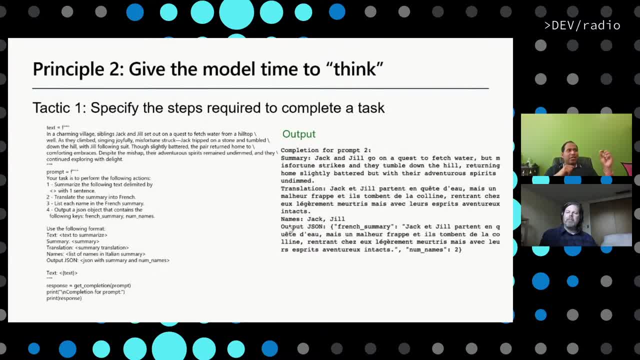 now for this tactic: specify the steps required to complete a task, right, and I'll go a little bit deeper on the technical aspect of it. but let me first tell, in a very high level, what does it mean. so I provided a text and in the instruction I say that your task is to: 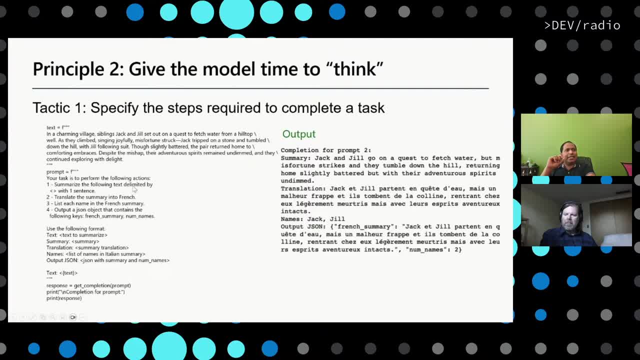 perform the volume accent. first, summarize the following text, delimited by triple and the, the, the triple angle, within one sentence. that's a clear and specific instruction. second step: translate the summary into French. third step: list each name in French summary. fourth step: output adjacent object that contains the following key friend summary and the number of names: right, and then I use the actual text. 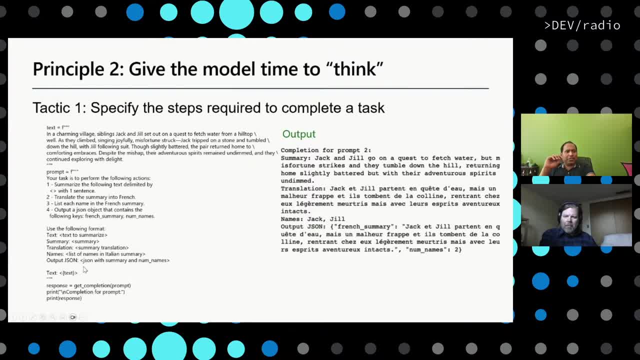 the summary translation name and the outputation, and then I provide the text in the in this particular, uh, triple back angle. and I'm asking now see that when I provide that, I get completions from um two, which is um summary. is this one translation? because this is the, this is. 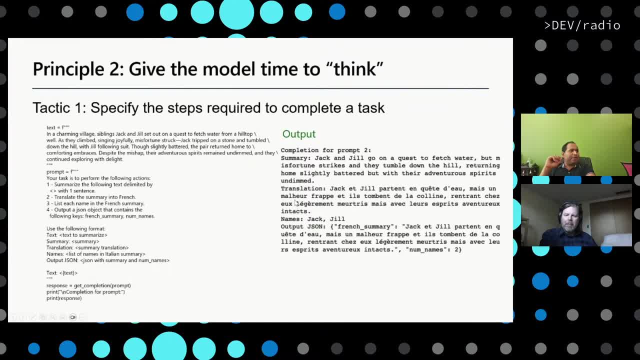 the following way: I ask: right, that summary, and then the sum, uh, uh, the translation, right. then I ask the names, then I ask the outputation. now you might be thinking: where is the? where time to think, concept, concept, time to think concept comes in because we are providing more and more and more. 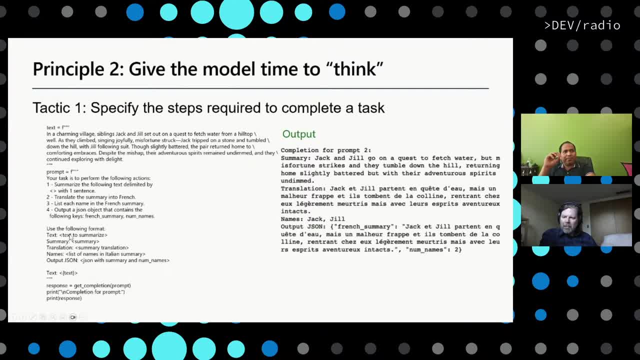 detailed instructions in the prompt right. so model has to think: okay, first I have to summarize, then I have to translate the summary to a different language- French. third, I have to list, uh, the name in French summary and then the output in addition. so I'm providing more detailed instruction so that model can think: okay, first thing, I need to do this and this and 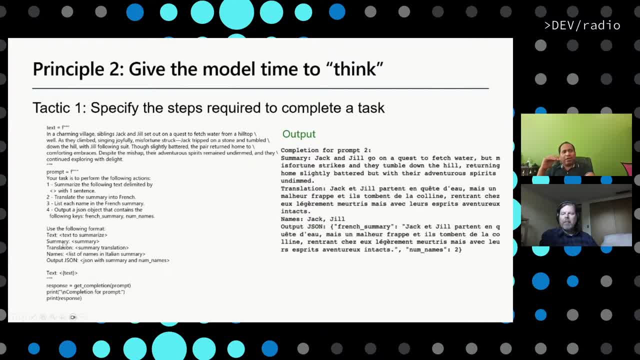 this and this right. and then I'm also telling the format, which, the format or the sequence of format. I'm looking, expecting the output. so that's, that's I'm saying you have to provide model, time to think. now I'll go a little bit deeper and on the technical side of the story, why this is uh. 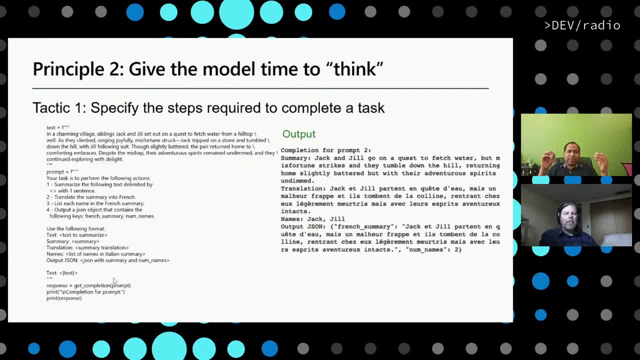 time to think. in a large language models, to think is means give more compute, right? if I provide a more time to you and ask you a question and to answer me back? in your brain you are parsing and you are trying to. you know, um, translate yourself, okay, what needs to be done. you are doing some computations in your mind because the more 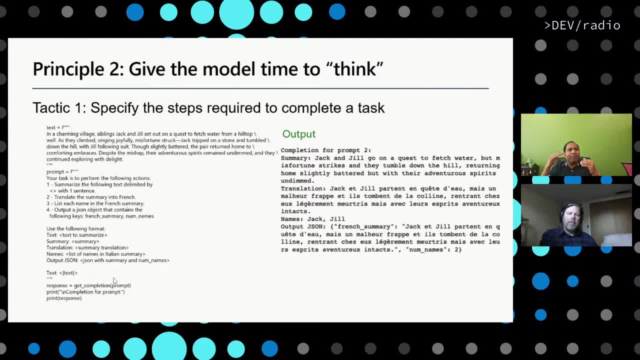 time I give you will get more time to think about. so in large language models we're providing a detailed instruction means we are telling: okay, these are the things and they can get more time to compute, but how the computer works through tokens means each um tokens is it's kind of a concept that it's not necessarily each word is that tokens. 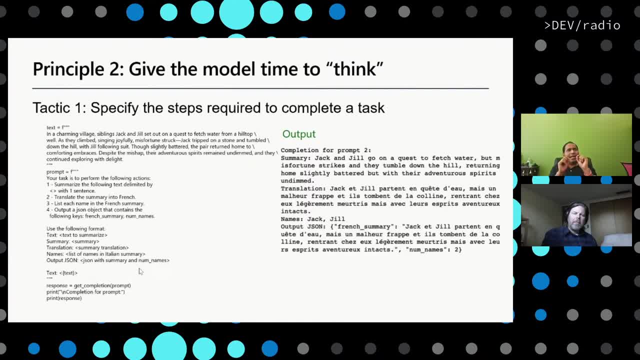 tokens. it's just a numeric number, by the way, from a given word, and one word could be just one token or just more than one token, could be two, three, four tokens, right, and in fact, if you go to the open AI, um, uh, you can see that tokenizer and you can pass a text and give you the exact token. 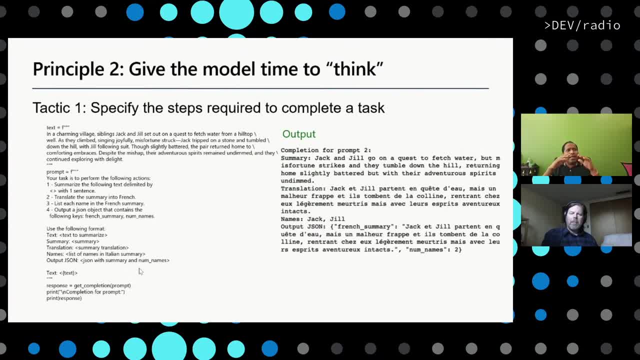 counts from them. I'll not go that part yet, but the more text you provide in a prompt, the more tokens you are consuming. the more token you are consuming means that large language models has a more tokens in his context and it can get more time to think. and token is equivalent a compute in in the large language. that's the reason. 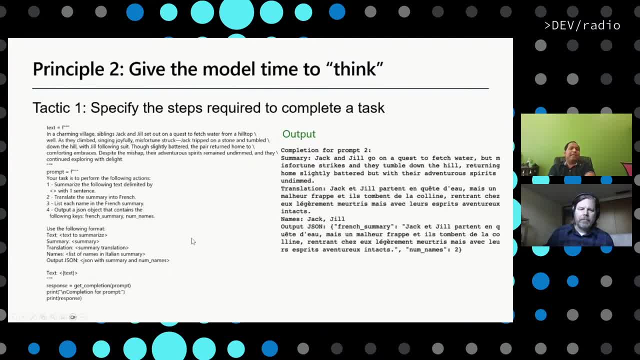 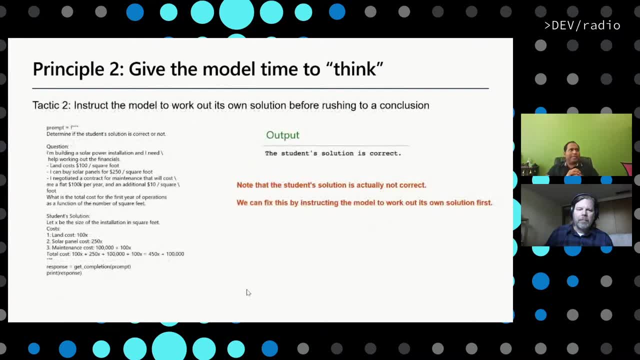 I said, the more you give or the provide, it's giving more time to think for the large language model. second tactic, on the principle, to instruct the model to work out in its own solutions before rushing to a conclusions, right? um, it's very important and it basically goes more on the 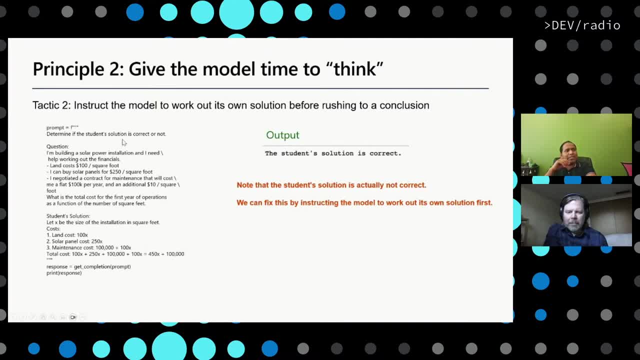 reasoning kind of a concept, for example here. if you see that determine if a student solutions is correct or not. the question: I'm building a solar power installation and I need a hug working out for the financials. plan cost 100 per square feet. I can buy solar panels for 250 per square feet and negotiated a. 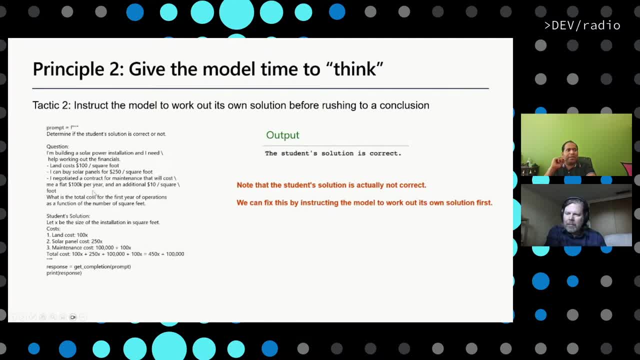 contractor and maintenance. that will cost me a flat 100 per year and additional 10 per square feet. right, so that's a negotiation. see, that's the how, how, the getting complex. now what is the total cost for first year of operations as a function of the number of square feet? now here I'm telling. 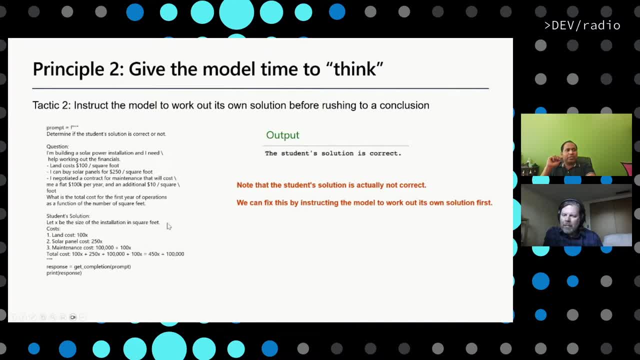 that the students answer: let's X be the size of the installation of the square feet, right? that, by the way, this is not students is producing. I am giving the models. uh, you know to to think and also you know, try that same reasoning and the math behind the scene with that kind of 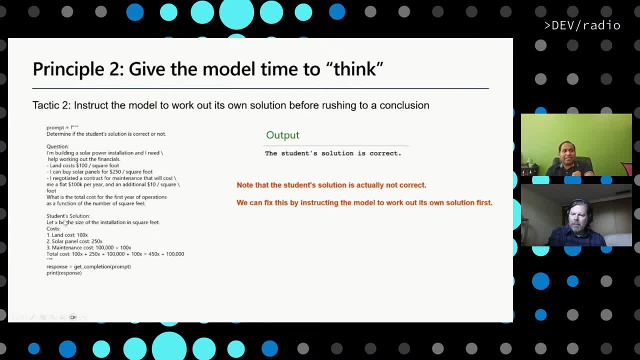 an explanations or the reasoning, so that I can get the proper answer. so I said: X, the land causes 100 X. solar panel cost 250 X, then maintenance cost 100, 000 plus you know um 100 X. that's this one, and then total cost is this: 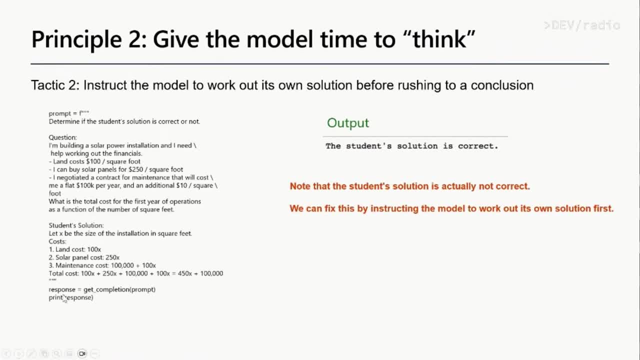 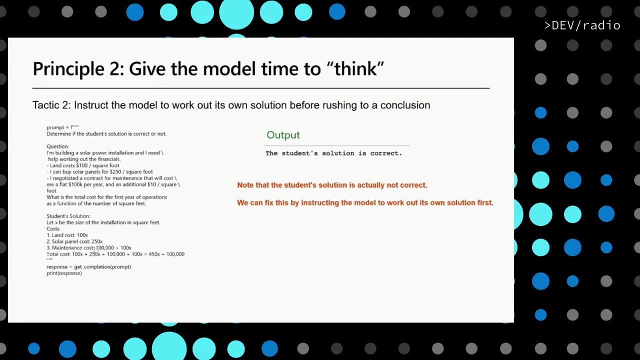 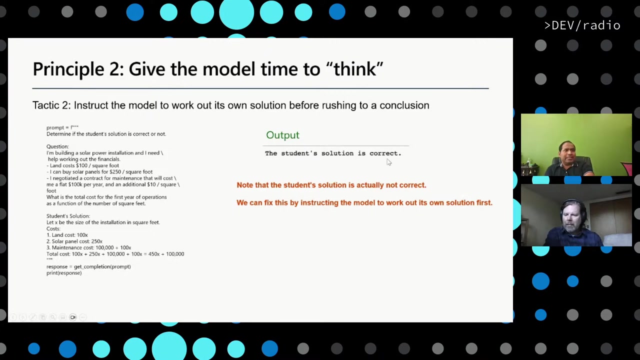 right now. then I'm asking that um, um, get the actual output right here. I am providing this one, but I did not, uh, say that, hey, this is the students solutions, by the way, the actual skills provided, and I'm asking model to verify and model saying this is correct. but 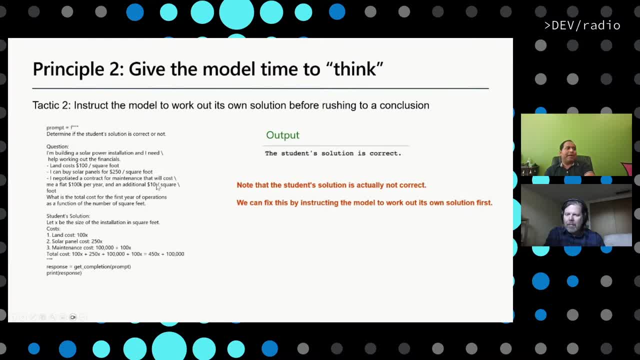 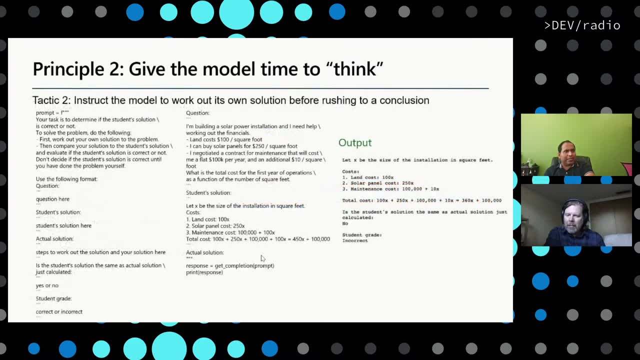 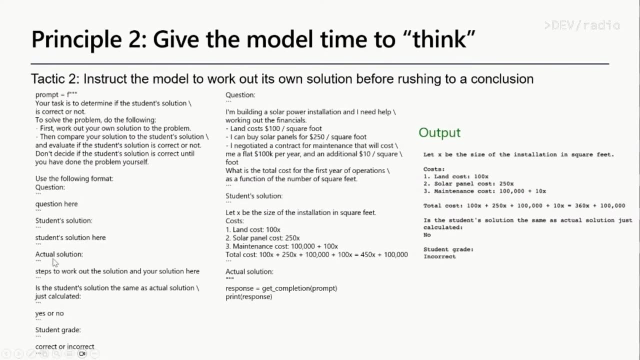 you know this is wrong because they did not fact get the negotiations part here right. but how i can fix it? this one with the same principles like this: i said, okay, this is the question, your questions here, your actual student solutions here right. and then your- i mean models, actual solutions and steps to work through the solutions. it goes here, then students. 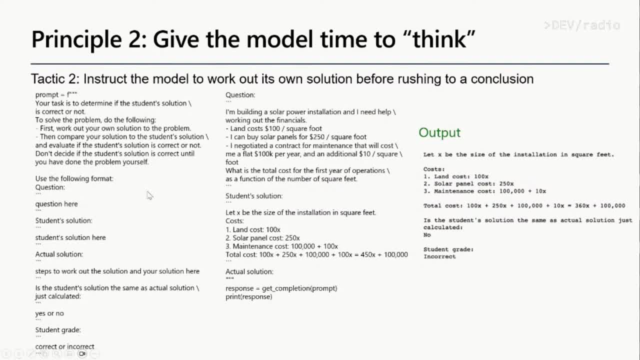 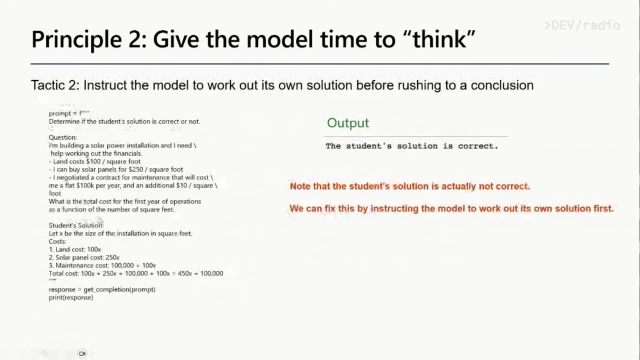 grade right, and then we provide here the actual question, the student solution, then the actual answer. but in this prompt, compared to the last one, last one, i do not have anything. i have actual prompt and the student solution, right, what the students have provided, and then asking: but here 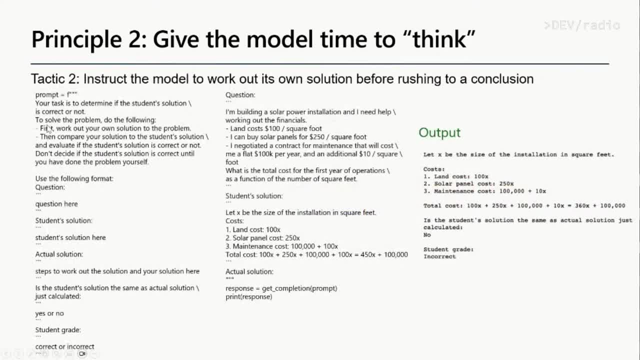 i am telling model your task to determine if the student solution is correct or not to solve the problem. do the following: first, work out your own solutions to the problem. then compare your solutions to the student solution and evaluate if the student solution is correct or not. you. 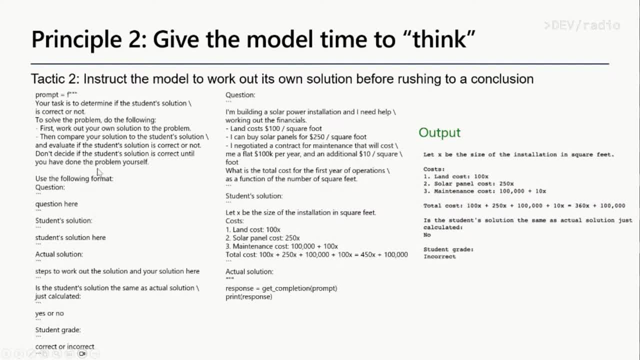 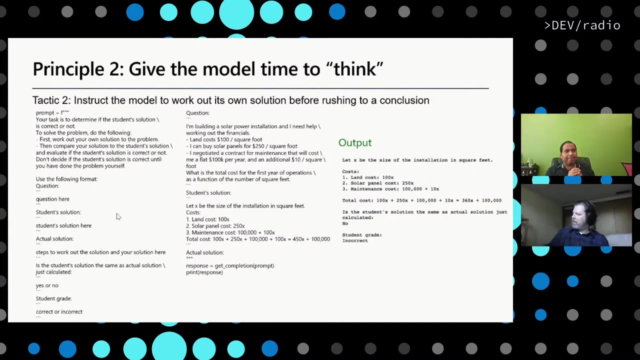 don't decide if the student solution is correct until you have done your problem yourself. same thing: if i ask your math and if i ask you the answer back to me, what do you do? you first try your math by your own and see if the answer is correct. then you response back right same thing. 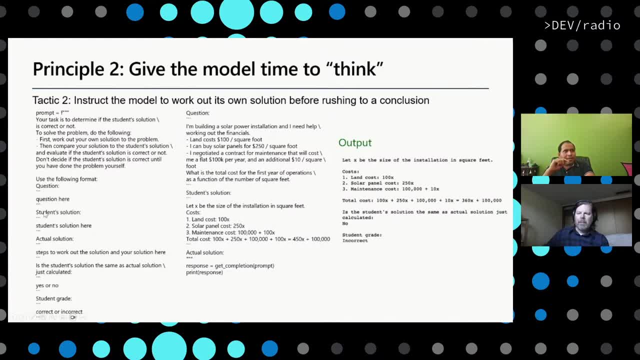 here your question, which is this one. then student solutions, which is this one. and, uh, student instructions here. means that what solutions actually come out the? the answer is correct, right, the actual solutions, where the model is providing the actual solution and steps to come up to the actual solution. then you are judging your actual solution with the student's grade. 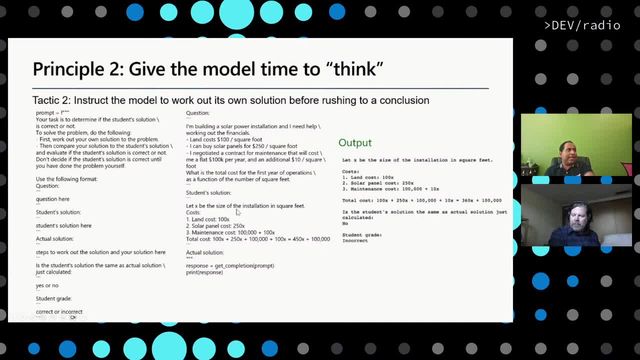 uh whether the student is correct or not, and then you are providing the query, and then you are asking the output and in this case, say: i did the same thing. let's uh the output. if you print this one, you'll get the output like this: let's x be the size of the instruction of the square feet. 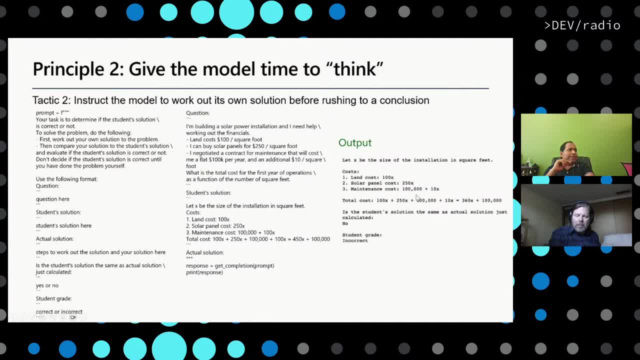 lag was 100x. solar fan: on this one, matrix was 100x. and then you are asking the output and in this case say: i did the same thing, let's uh the output. if you print this one, you'll get the output like this one. and this one matrix was 100, 100k plus 100x. total cost um is 10 250k, this one plus 10, 10x. so 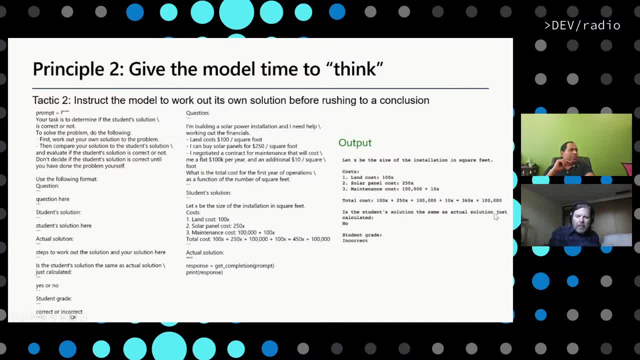 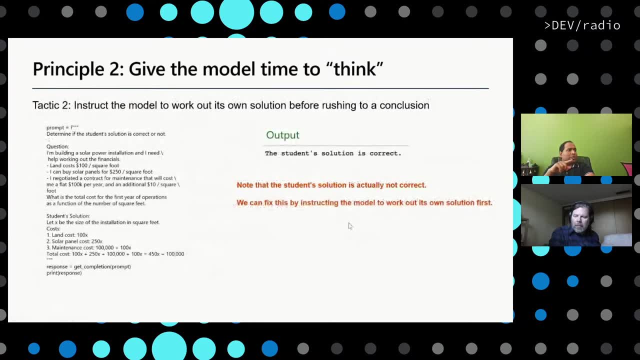 300x plus 100k. the student social has the same solution, just just calculated. no, it's not that because they have not calculated the same thing right. they're saying the flow service is correct because here the student solutions is 450x plus 100k. in fact i know to switch. in fact i'm saying 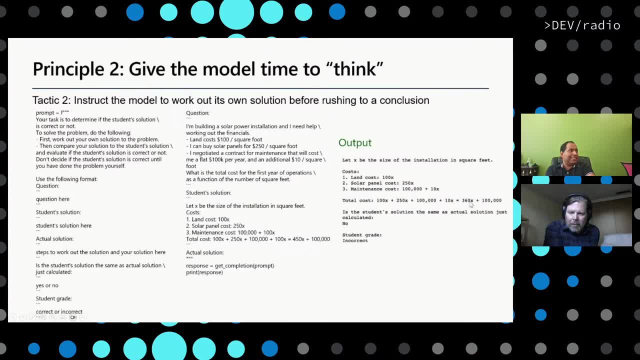 here. it's right. that's why i'm showing you here, right, that's why i'm showing you here: right, that's actual solution. but the actual solutions is 360x plus 100k, not 450, right, and that's the reason the student service is incorrect. so this kind of things comes up. you need to always instruct the model. 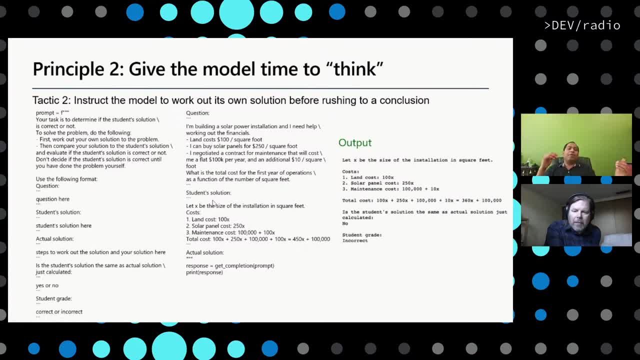 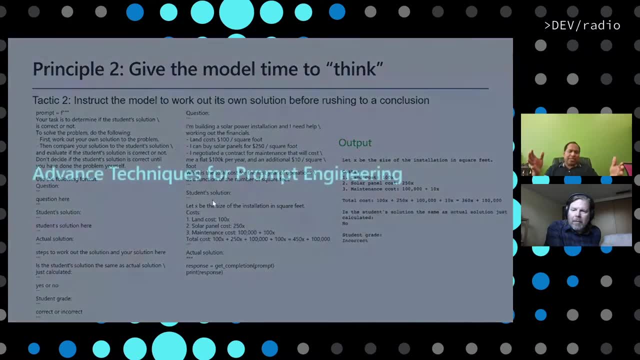 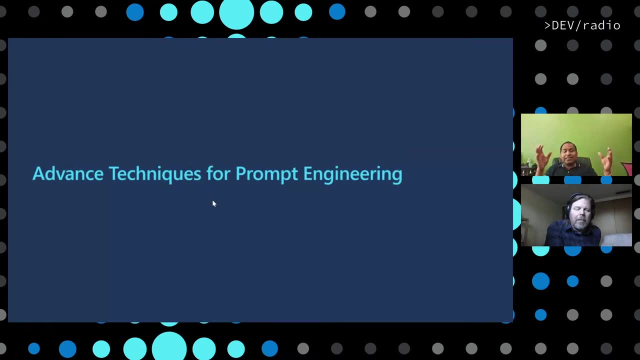 to work out first in their own solution and then compare with the actual solution and come up to a conclusion. right now, that's kind of a couple of techniques. i taught you that. what are the different techniques you can use to write a better prompting? again, these are not all. there are many, many techniques. but now i'm gonna tell you that what 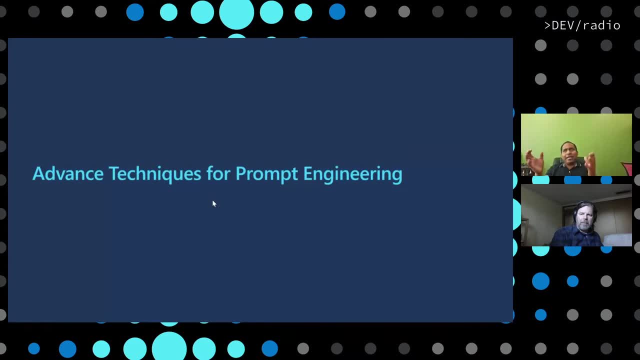 are the different techniques for advanced, prompt engineering and in fact, once you go to that subsequent, then you will understand that before i talked about the few short learning, uh, the reasoning over that, you'll understand where this comes from, how the tactic, the techniques or the tactics has been developed. it is not just something you know arbitrarily coming out of, you know some. 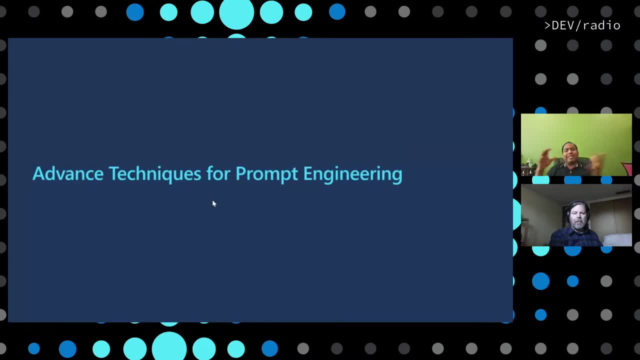 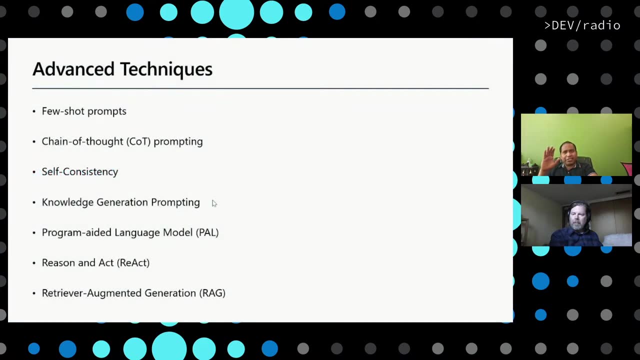 it is based on the science and research paper. those techniques has been proven. now we'll go to deeper on that. first of all, these are the techniques i'm going to teach you. uh, in this particular topics, which is few shot, prompt, chain of thought, self-consistency, knowledge generation. 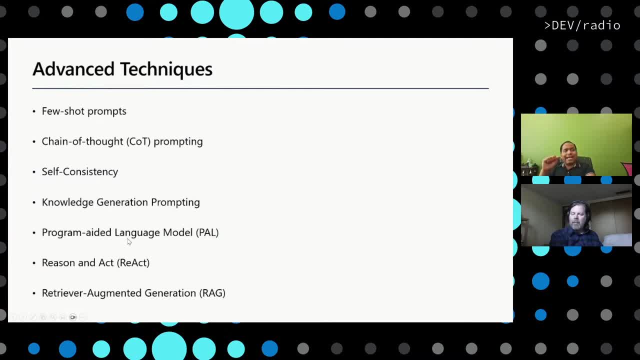 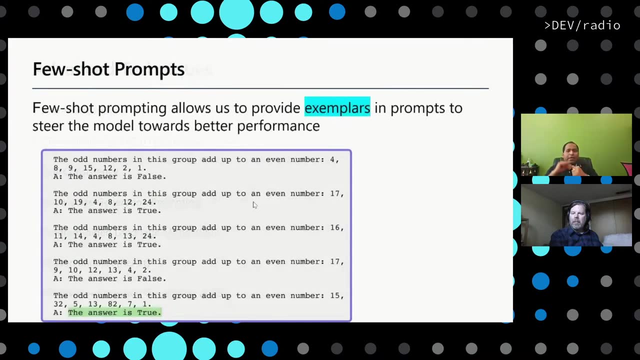 prompting, programmated language, model, spell, and then reason and act, which is called react, and the last but not, which is very important rack, which is called retriever, augmented generation. right? so let's start with few shot prompt, right? so the few shot prompt, in fact, in our first, i think first, second or third, 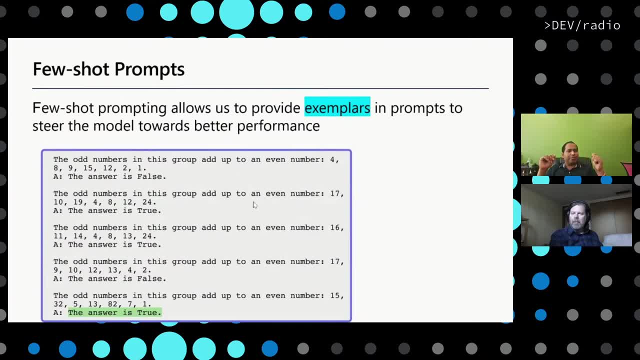 slide. we talked about some examples right, which is called few shot prompting, and few shot prompting allows uh the models to provide some uh allowed. basically, we provide some examples to the models and model can steered towards those examples to give you the better output or the better. 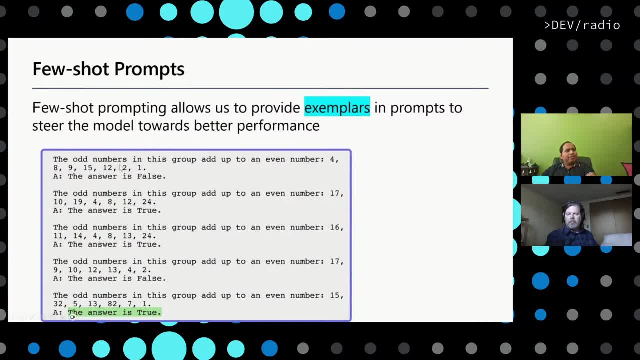 performance in a given token, right? so here i'm saying that these are the um input, sorry, the examples i've provided say that the odd numbers in this group add up to the even number is, uh, four, and sorry, the four, eight, nine, fifteen, all these things and answer is: the answer is false, right? second example: i'm giving two, third. 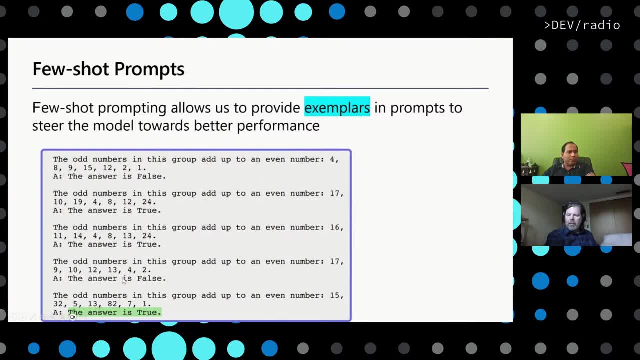 example i'm giving, i'm saying the answer is true and like that. so i'm giving almost four examples. then i'm asking a question. the odd numbers in this group add up to an even number and i'm giving this numbers: fifteen thirty two, thirteen, eighteen, eighty two, seven and one, and model said that 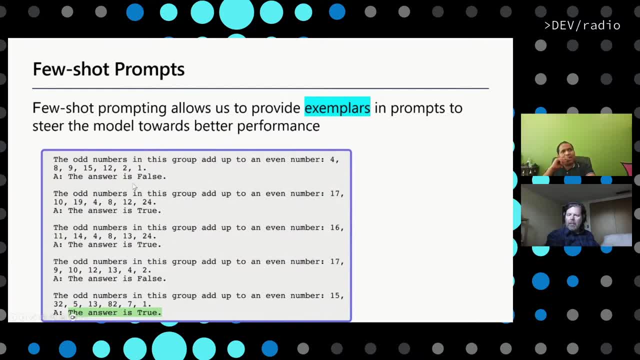 okay, the answer is true. behind the scene it says that: okay, i have provided these examples. it understand that. okay, these are adding up. it's doing the calculations. that's how i'm giving the answers, true or false. well, this given on the question, into the calculations behind the scene. 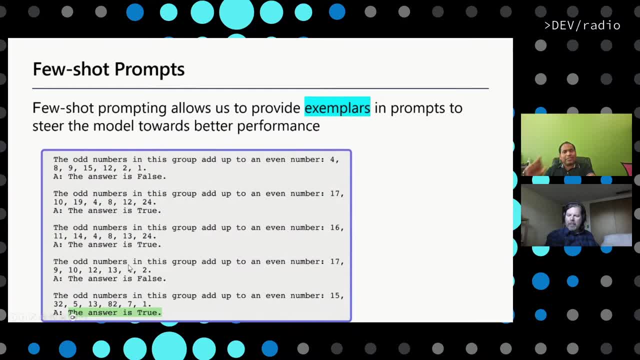 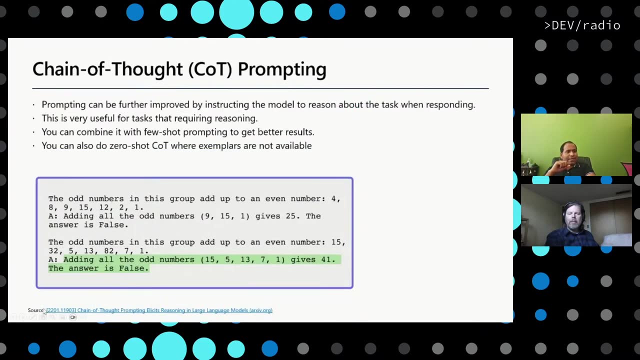 and give you the actual answer. so having an example is always good in your prompt. show that you can steer to it and get the actual results. it's very important. and second is a chain of thoughts which are cot prompting right and in fact this. i've provided a 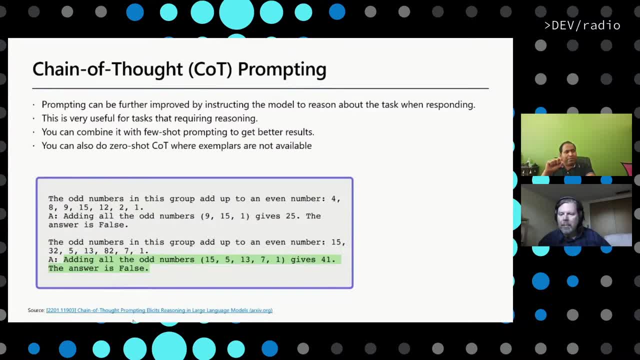 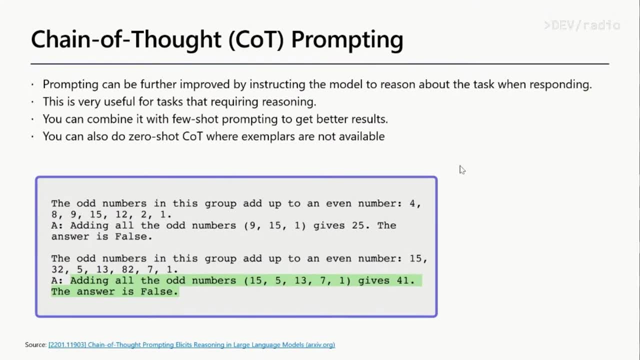 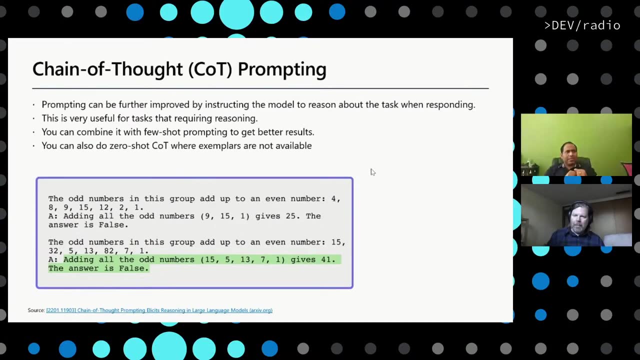 source here at the chain of thought. it is came out of a research paper which you can go and search, search later. but what is the crux of it is that, uh, you are telling the model to think step by step, with some reasoning, and then response back right, which is called um chain of thought, and you can 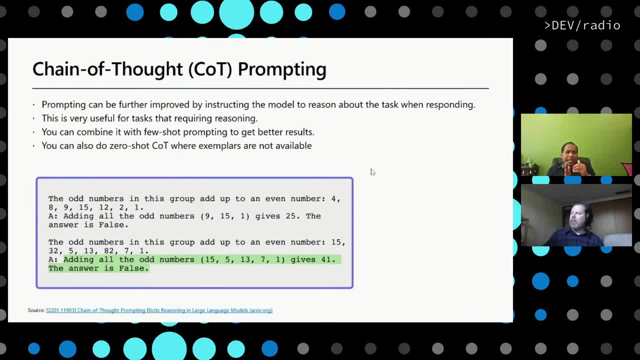 combine that um, um in a few sort prompt as well with the chain of thought and chain of that also right now in the last couple of months this came out of a research people called zero short chain of thought. i mean so in a chain of thought you can provide example so that model can understand what is the. 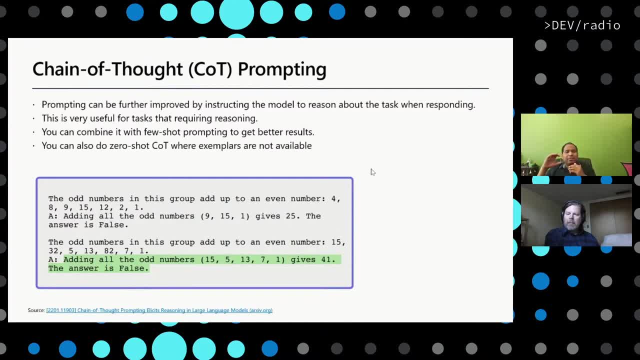 different thought process has been involved with that example, or you do not provide an example but you can write a single statement which will go later on that i'll tell you that was that in a next slide and that will understand. before it output it, it has to go through some sort of thinking process. 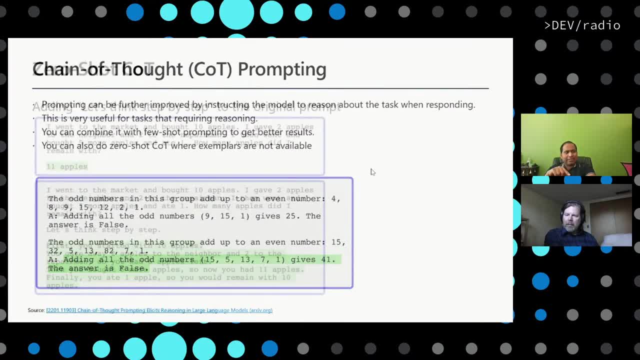 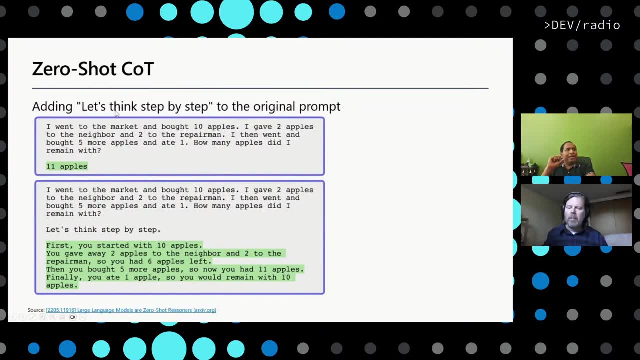 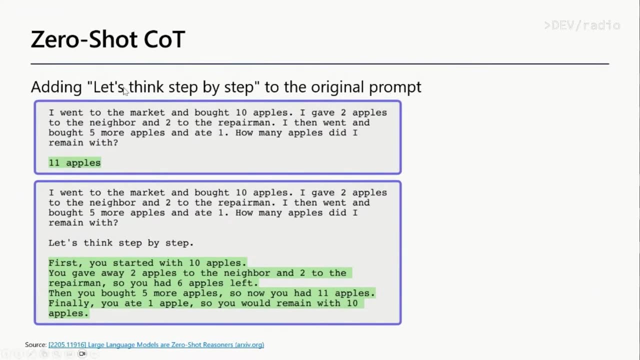 behind the scene. So zero-sort, and again, this is a research paper I listed here. just say this particular sentence in your prompt. let's think step by step. So we are not providing any examples, rather we are providing a line in your prompt, right? 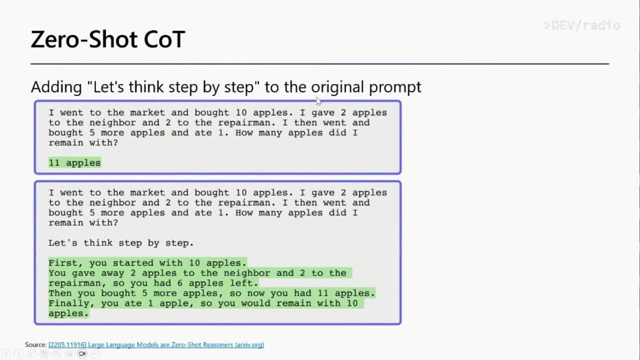 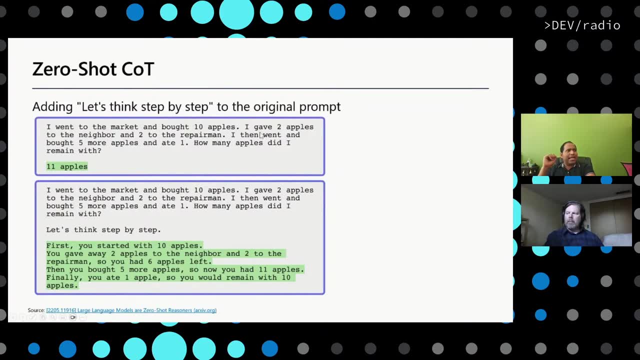 And, by the way, when you go to some demos, you're going to show that. So here, the original prompt was like this: I went to a market and bought 10 apples. I gave two apples to the neighbor and two for the rich man. 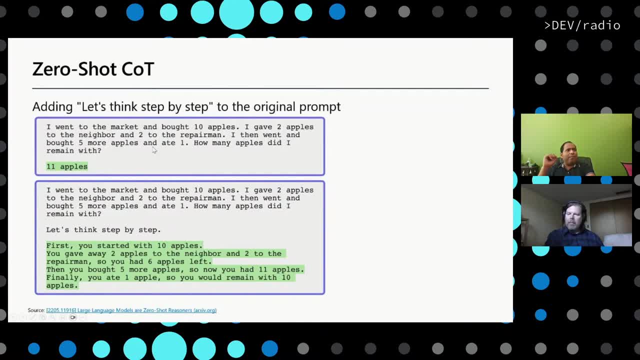 and I then went and bought five more apples and I ate one. How many apples did I remain with? Then it just say that 11 apples right, Which is not right. But if I say, on the same question, let's one more line, if I add: 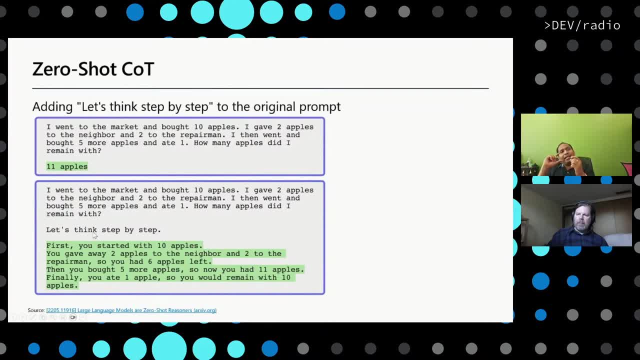 let's think step by step, then model gives what? More time to think. As I said, the principle you need to give more time to think. When you say that let's think step by step means you are telling model time to think. 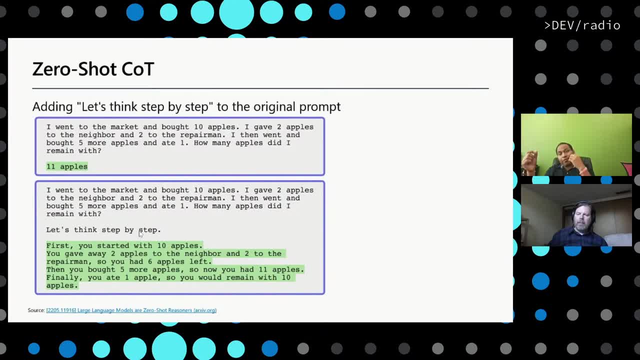 And at the same time, time to think means putting lot of, basically tokens has to be consumed and which give the compute to thinking of the model. Now here, first step: you started with 10 apples, Then you gave two apples to the neighbor. 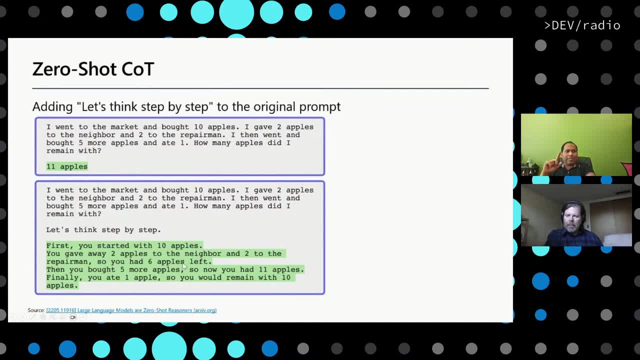 and two to the rich man. So you had four apples left. Then you bought five more apples, So now you have 11 apples. Finally, you ate one apple. then it remained 10 apples. But if you don't put that line, 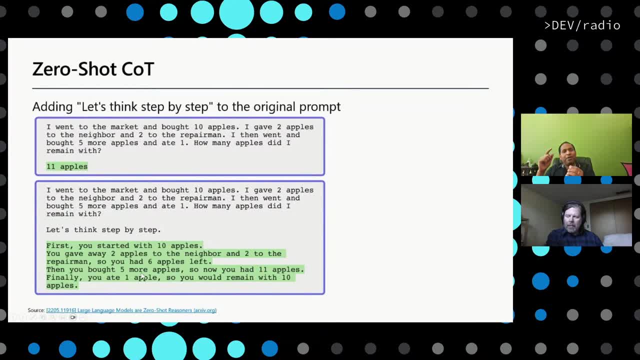 your answer is 11 apples, which is wrong. So think about how powerful just adding one line in your prompt get the right answer. So that's called zero-shot chain of thought. Now, why it is zero-shot? Because we are just adding a line. 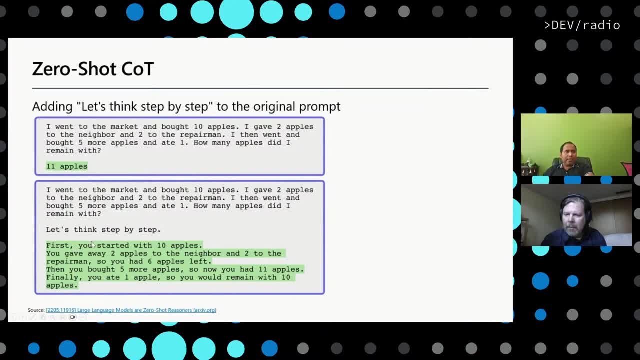 but we are not giving any example steps in the prompt. If you think about the regular chain of thought, which is not a zero-shot, then typically what you do, you just add a couple of examples like instruction or steps. that goes through that thought process. 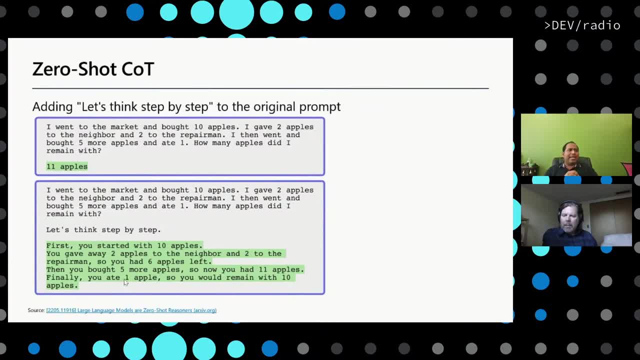 and then give you the right answer, You'll get same thing. but then now you'll be asking that, hey, whether should I use zero-shot or whether should I use regular COT? just giving an example What I said before. the principle: 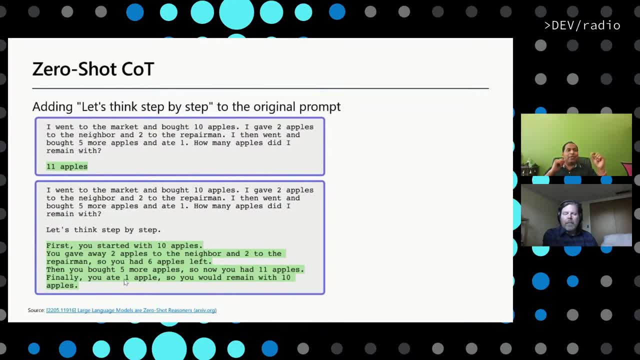 it's an iterative process. I cannot tell you that only zero-shot gonna work or the exemplar's chain of thought gonna work best for the application. You need to try it out. you need to test it out. It's an iterative, prompt development process. 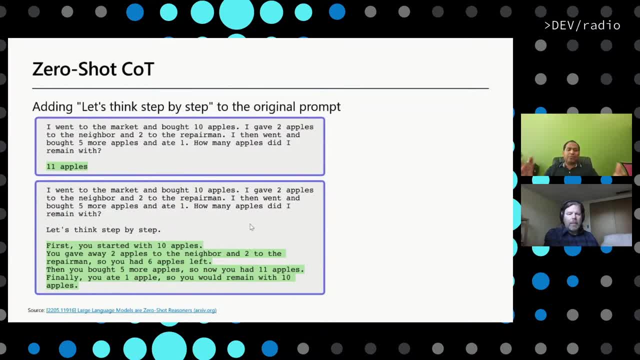 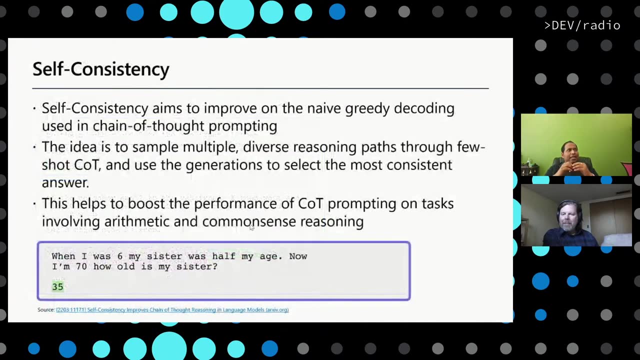 and see which one you are getting the right answer. That's what you need to decide. I hope it makes sense. so far right, Yeah, no problem, so far Awesome. Now other technique is a self-consistency. What is self-consistency? 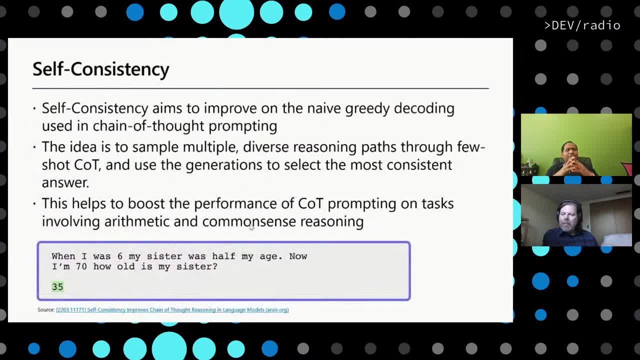 So self-consistency is basically kind of what: you provide: a sample, multiple diverse reasoning part with a few shot of kind of a COT approach, and then you ask to generate some sort of consistent- I don't know- a few shot of kind of a COT approach. 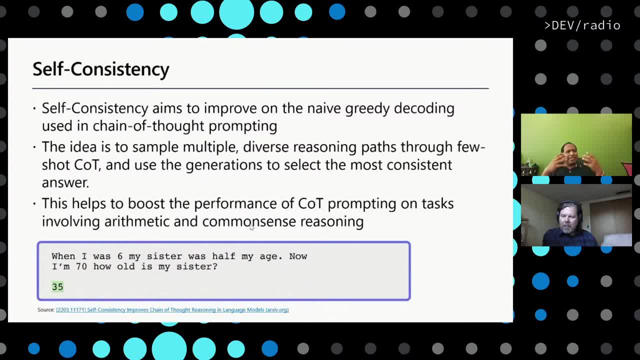 and then you ask to generate some sort of consistent answer from there, And from that consistent answer you are telling model which is the most voted, kind of a thing, which is the most weighted answer. you pick that one. That's called self-consistency. 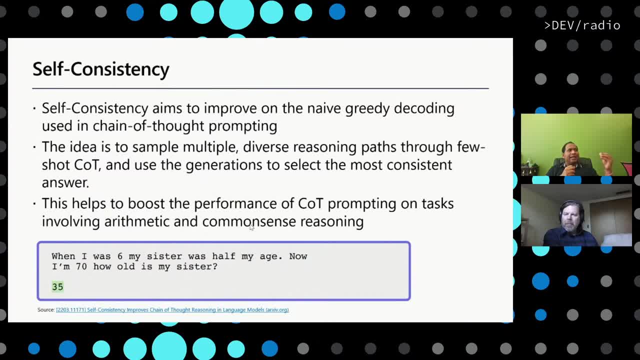 Why is it designed? It's designed to basically improve the naive greedy decoding in your chain of thought, prompting Now what is naive? you know, greedy is a mouthful word, I know, but the naive greedy decoding, think about. 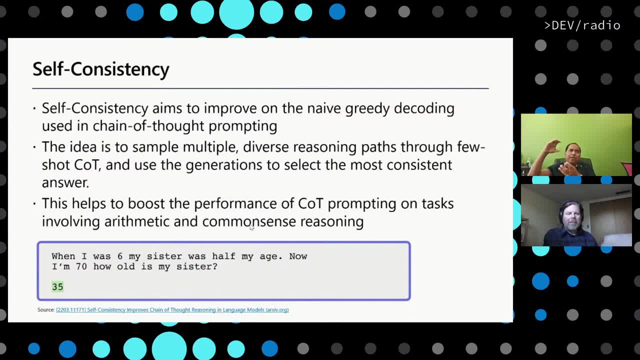 nlp kind of a concept, right, where you have an input and you get a probabilistic, uh, output, up all the proper next sequence: uh, the word you'll get an output. right, that i mean not an output, the next possible probabilistic word in your, in your statement. right, uh, now and then what it does. 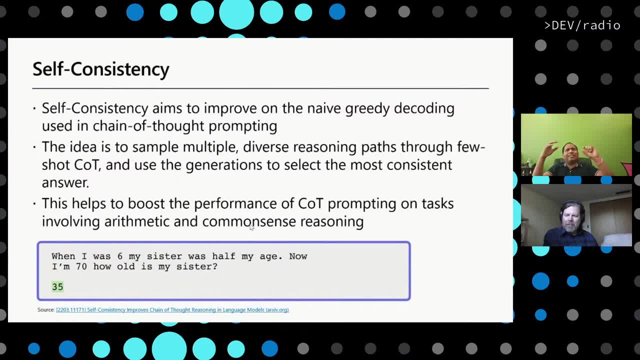 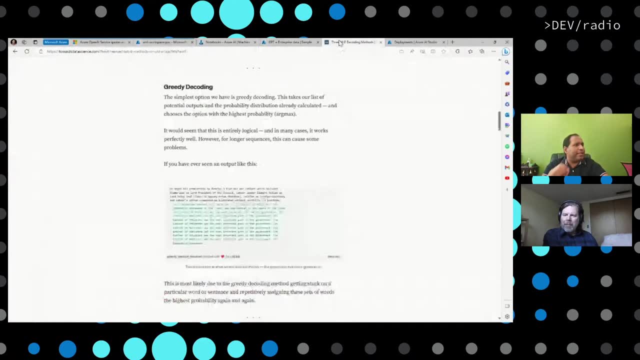 is basically whatever the most weighted you know probabilistic, uh, the sequence, you pick, that one that's for night, night decoding, but it's not not always the right things, uh, to use the knife graded decoding, and in fact, let me, let me share you with this one right, for example, this knife. 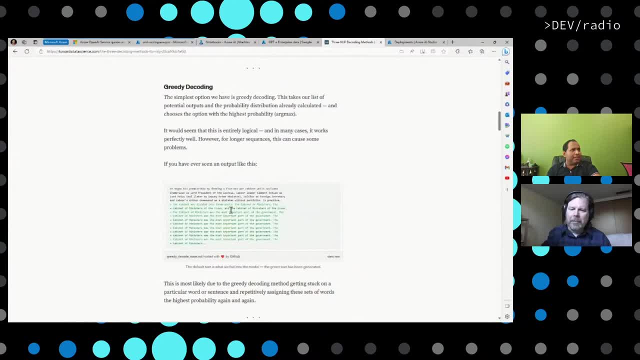 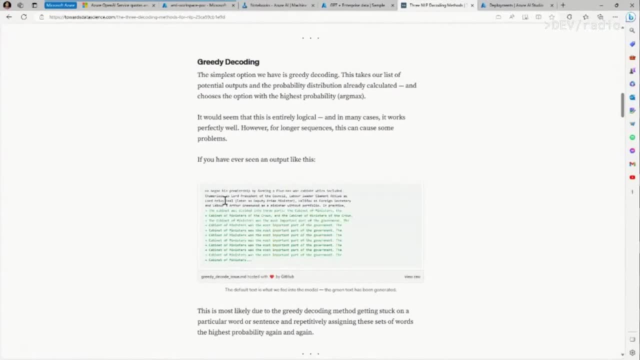 decoding. i just pick it from this. you know, this article, that here you see that it begins with the um, the partners who are forming a five-man war cabinet, which is included, uh, uh, you know, chairman, and the lord, president of the council, labor leader, cabinet athlete lord, will also very 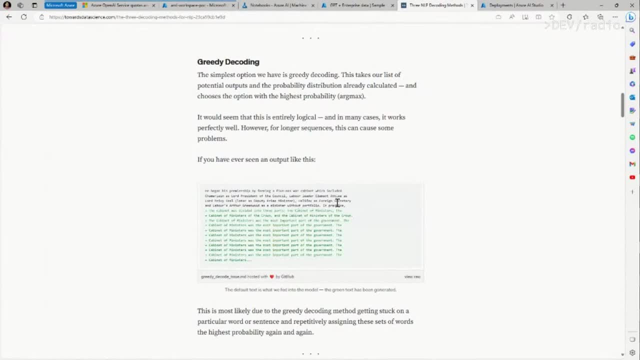 tough. what, by the way? the late deputy prime minister halifax and foreign ministry and liver author, mr blah blah blah. and then it says that in practice, the cabinet was divided into three parts: the cabinet of ministry, the cabinet of ministers of the crown, the cabinet mr of the crown, and then 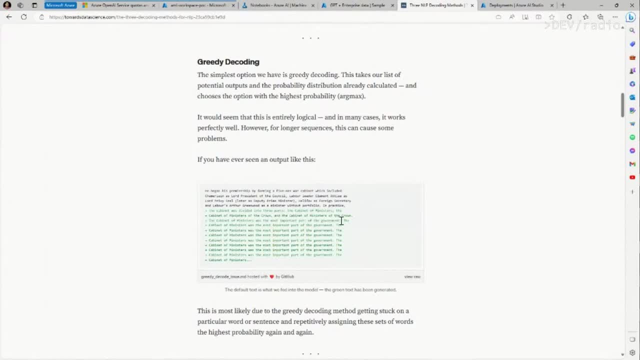 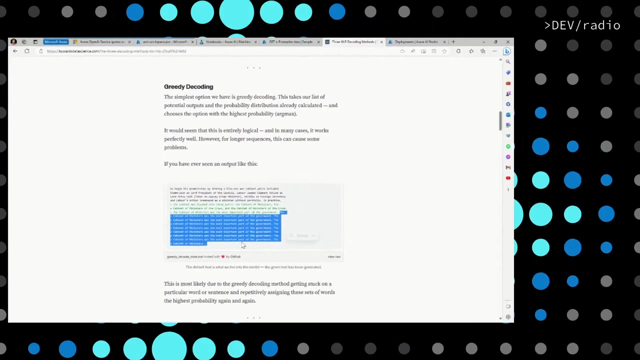 the cabinet of the minister was most important part of the government. and then this piece is getting higher weighting and keep on repeating the same word. right, that's called naive decode and gradient decoding. it's understand the next possible probabilistic distributions, which has been already calculated, and try to choose that option with the highest probability, because that's. 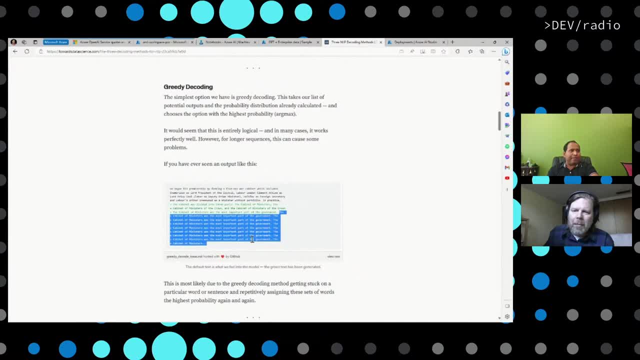 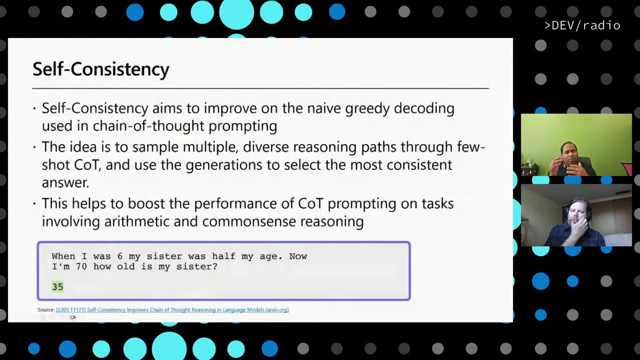 go to the highest poverty, which is not always right, right, which just makes sense in most of the cases, but not always right. and to solve that purpose, the self-consistency um actually comes into the picture. so means that you provide some examples and the questions and then you come up and answer. 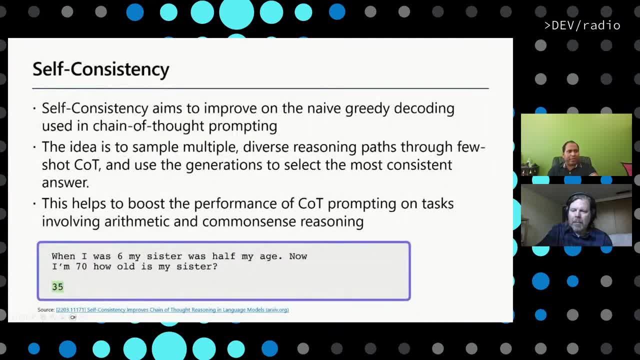 and try to see which one most voted, and then you go from there. for example, in this one right, if i ask, when i was six, my sister was half of my age. now i am 70. how old is my sister? it's a 35, which is not quite correct. 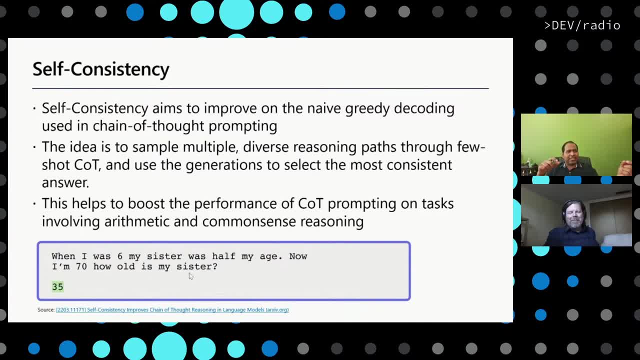 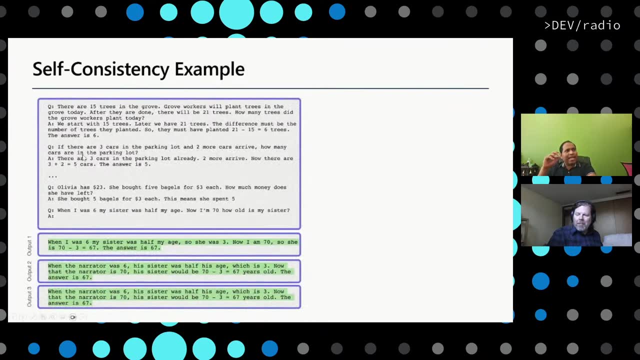 right and i'll say how you can solve that problem with a self-conscious example. and, by the way, self-consistency is nothing. something came out of community, it is, an research paper has been published and that's what has been produced. now, in that self-consistency, you see this how they have said. this is the questions right, and 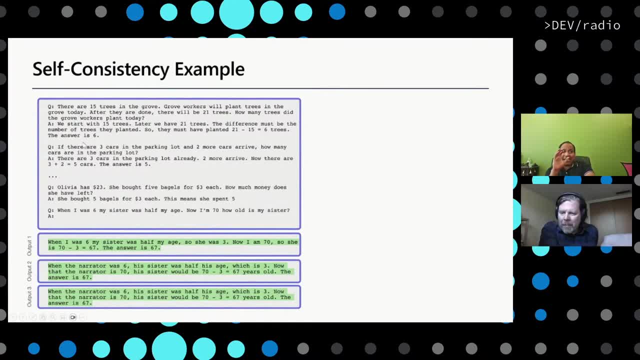 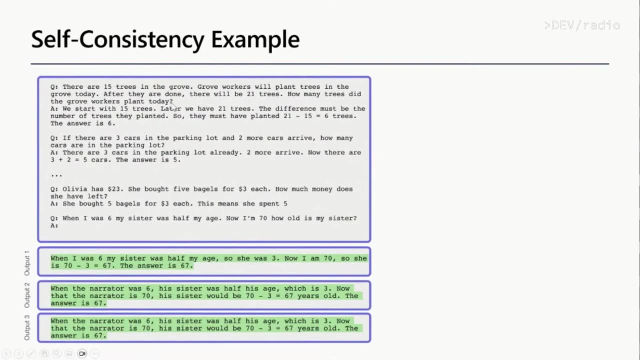 in that question. um, this is, by the way, the exemplar question, not the actual answer of the question. so there are 15 trees in the grove. grove workers will plant trees in the grove today. after they are done, there will be 21 trees. how many trees did the group workers plant today? then i am providing. 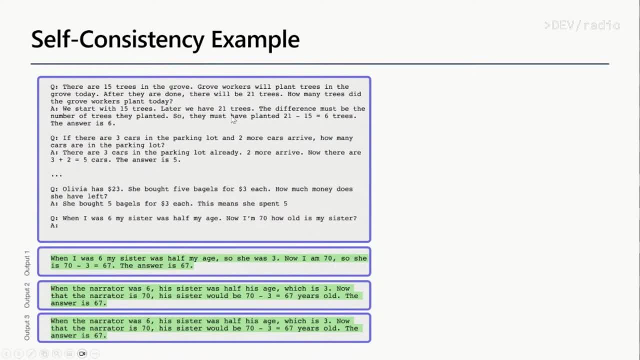 some answer for that question. we start with 15 trees. later we have 21 trees. the difference must be number of trees they planted. so they must have planted 21 minus 15, 6 trees. answer is 6, right, and then i give the another example. then i give another example, then i ask the question. 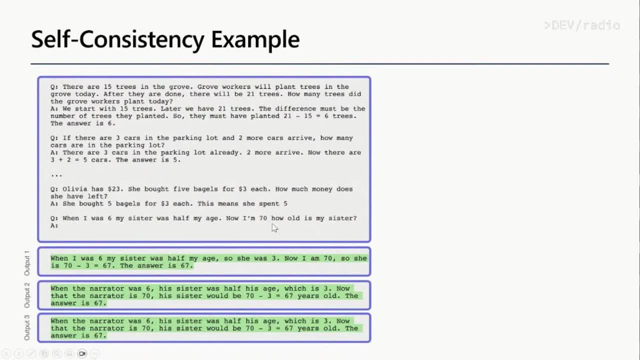 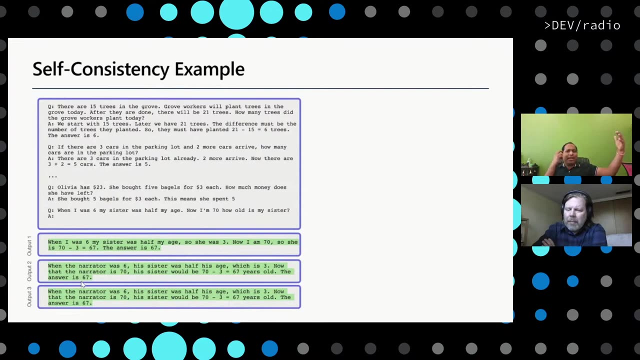 when i was six of my sister was half of my age. when i'm 70, how was the system then? it outputs a different outputs means it try to basically try to solve the problem with the answer to the question problem in a different ways. right, if i say, okay, i want to get five, five can be done by: 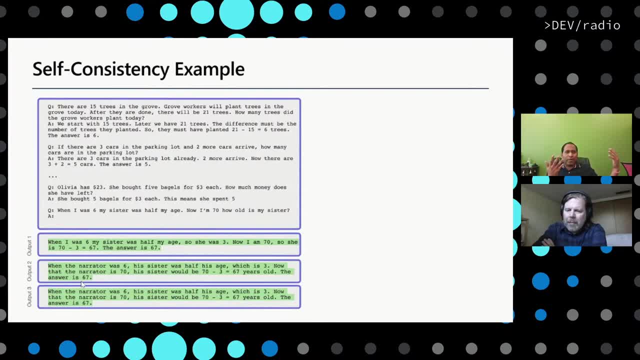 two plus three: right, that's the one way. or i can say four plus one, or i can say zero plus five. all are correct. so means that to get to five, i not only have just one answer or one way: two plus three. i can provide multiple ways to come to the conclusions: five, right. 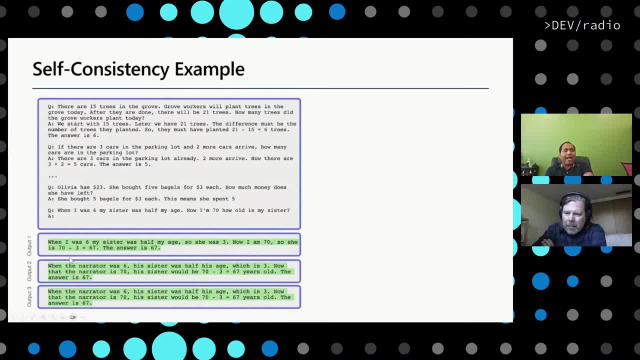 same thing. so here what it does. i provide the question. it try to solve the question in a multiple way. first output is when i was six years old. i mean six. my sister was half of my age, so she was three. now i'm seventy, so she should be seventy minus three, which. 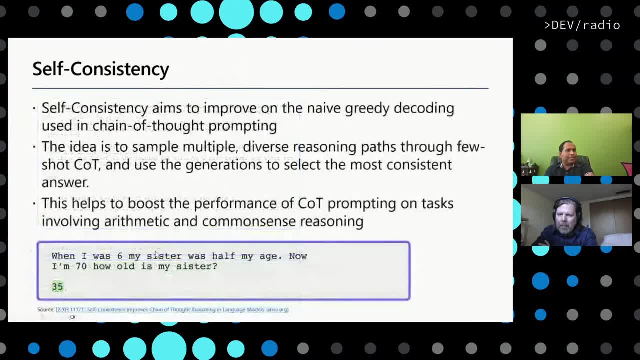 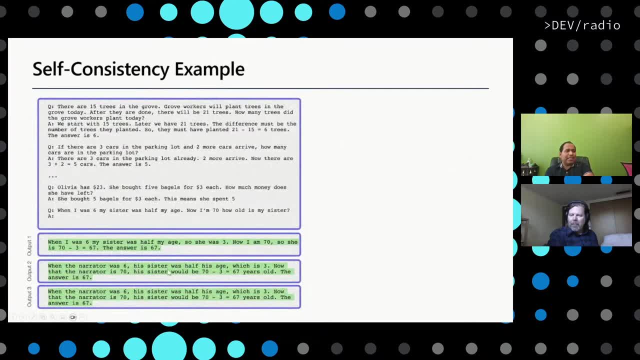 is sixty seven. the answer is sixty seven and previously, you know, uh, he said the thirty five, which is not right. right, so now he gets first output sixty seven. now, other way to get that, when the narrator was six is sixty, was half of his age, which is three, now that. 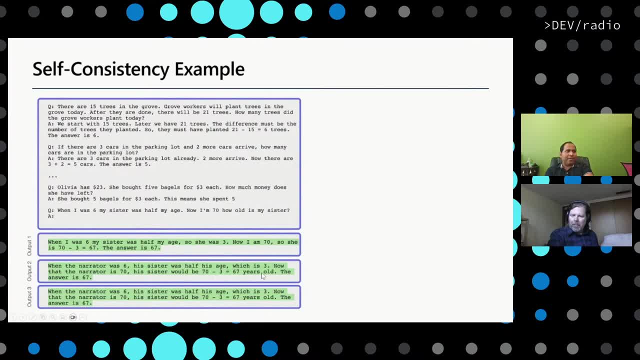 narrator is seventy, history is seventy minus three, which is sixty seven right. and then other example: the nature was six, sister is half of the age three. now that was negative seventy. so it's trying to come up to a different way the examples i have provided here, because here i provided. 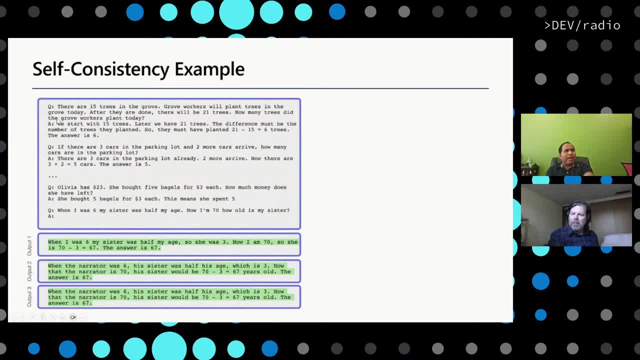 a tree. but, um, i'm, i'm not, i'm asking about the age, but i'm providing an example of tree, example, parking lot, another example of the buying something from a dollar. so different examples i'm providing to come up the right. uh, you know, uh, answer same thing is: try to. 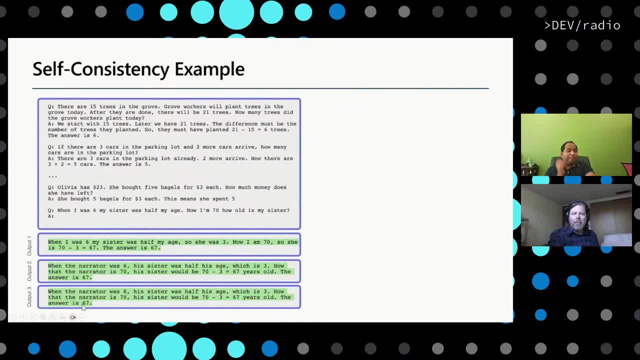 do them the most. one and maybe, maybe fourth output could be just. for example, it could just be 35, but while it give you the answer, it will not take to the fourth output because the majority voting is 67. that's how you get, so it will take from that and that will give. 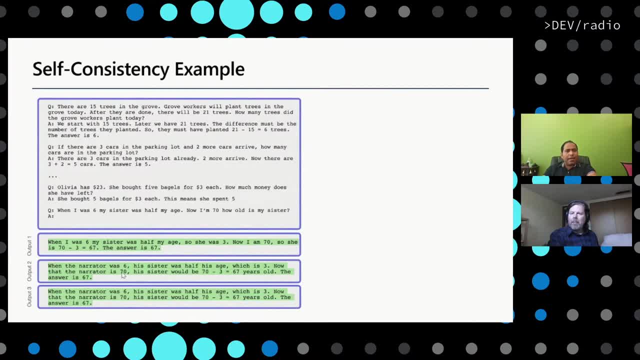 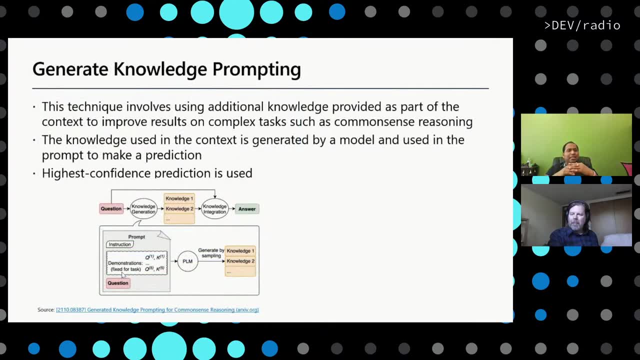 you that that's called a self-conceit. now we're going to go to the next one. it's called the quedar. uh. so these techniques is um, involve additional knowledge provided as part of the context to improve the complex tasks such as common reasoning. right, um and uh, it is very it is. 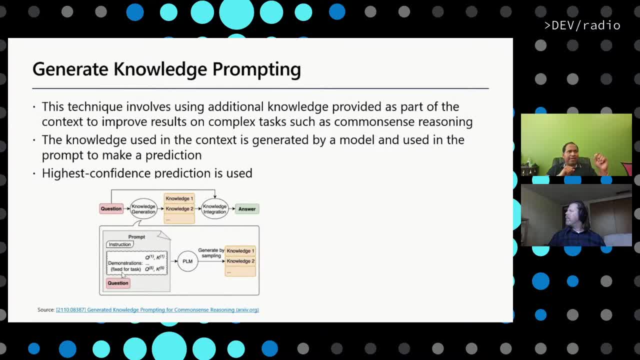 very similar to- uh, we're going to talk about the rag approach in the later. it's very kind of a very similar, but it gives you the high confidence. prediction is used in the in the knowledge right, so in the in the in the next slide, sure, sorry? 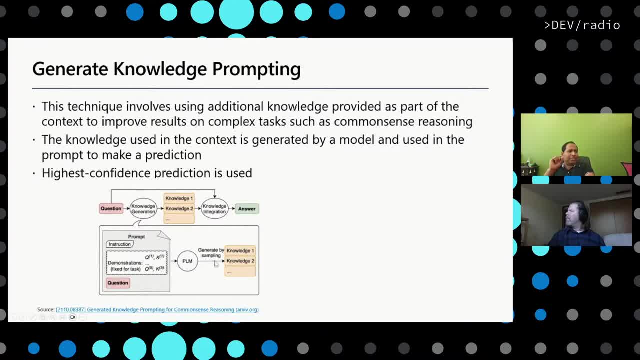 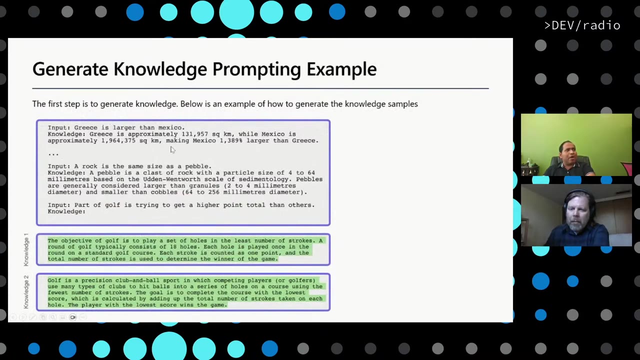 okay, in fact, this particular screenshot i've taken from the research paper itself. so you have a prompt, you generate uh questions from that knowledge prompt and then those questions feed into the knowledge integration and then you get the actual answer. so how that practically works is that. so generate knowledge prompting is the first step, is to generate knowledge, and below is the example. 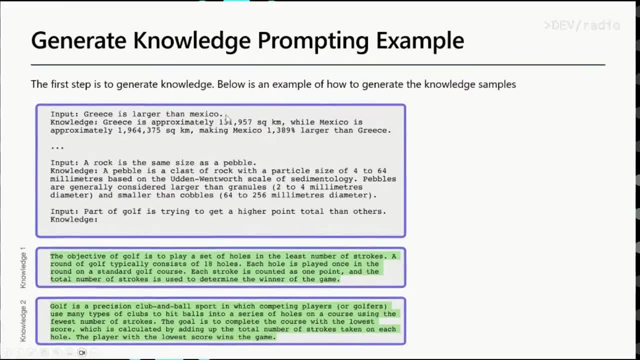 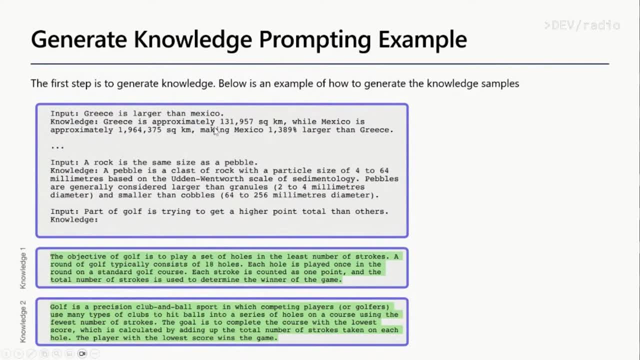 how you can generate money. so input is greece. is the larger than mexico. the knowledge which i provided. i'm not telling in this time yes or no. what i'm telling is: greece is approximately this much of square feet as a square kilometer, while mexico is approximately this one making. 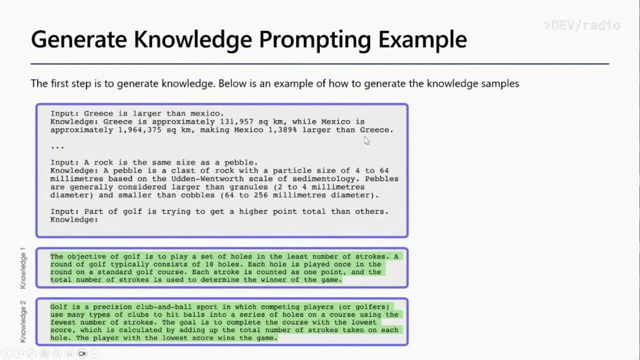 mexico one third to be larger than fifth. so that means what that means: mexico is larger than greece. second, i'm putting in another rock example. a rock is the same size of a pebble. knowledge. a pebble is a class of a rock with a particles with a 4 to 64- you know- millimeters. 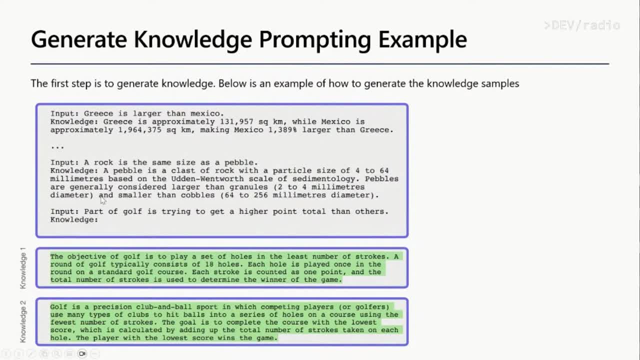 based on the ultra vision, all the things, blah, blah blah. then it's generate a knowledge. i would say this is the input and this is the knowledge. then again, i put an input and i'm asking to provide me the knowledge out of it. what is the input i provided? part of the glove is trying to 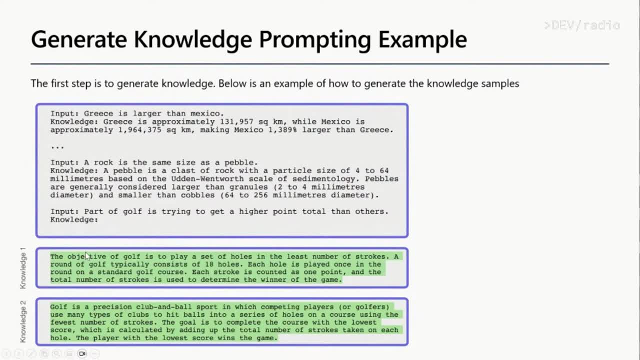 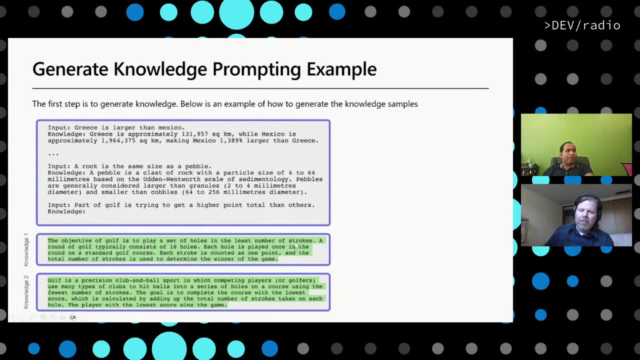 get higher point total than others. and then i'm getting a true knowledge from that. first of all, they say the objective of the golf is to play the set of holes in the least number of strokes. a round of golf typically consider the 18 holes. each hole is placed in the center of the golf and 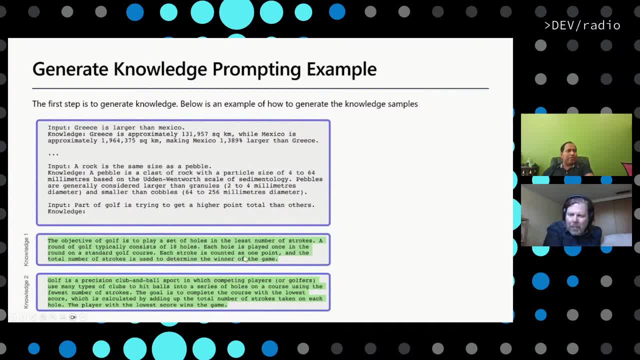 is once in the round of a standard golf course. each strokes is counted as one point and the total number of stroke used to determine the winner of the game. another knowledge has been generated: golf is a personalized club and ball sport in which competing players, or the golfers, as many. 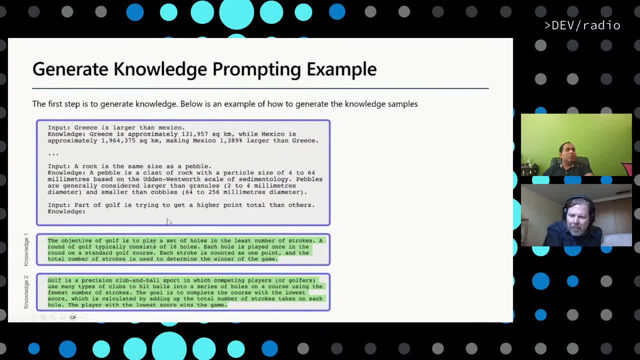 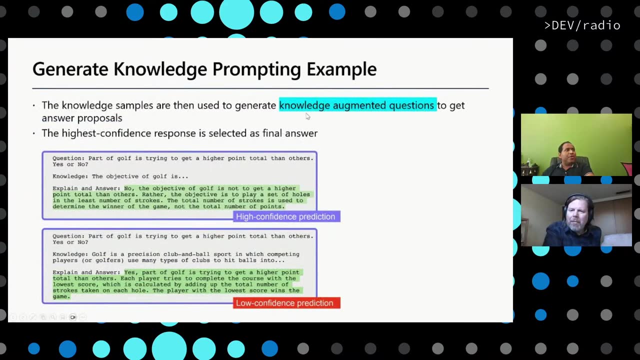 types to clubs. it was blah blah blah, right, so these are the two. knowledge is generated from that given input then. but next, then here is it comes then. what i did in this example is that the knowledge samples are then used to generate knowledge augmented questions to get the final answer, and then the highest confidence is taken for the final answer. 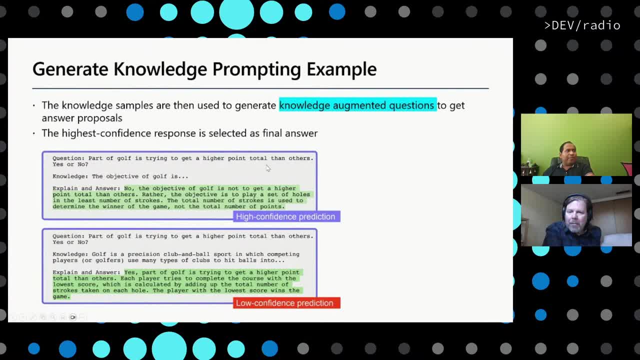 so means that we said part of the golf is trying to get the higher point total than the others. yes or no? then the knowledge which has already been generated before we feed on that and then give you the actual answer? no, the objective of the god is not to get the higher point total in. 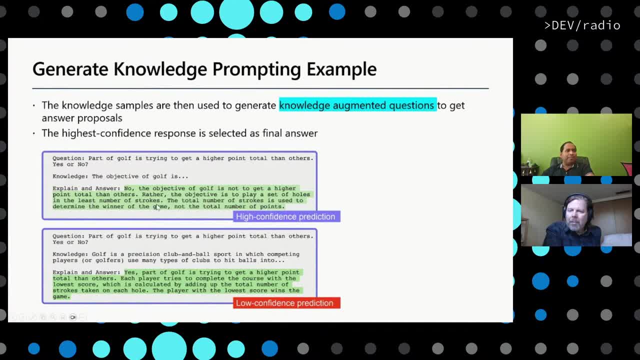 the others, rather, is object to play the higher point total in the others, rather, is object to play the set of holes in the least number of strokes. then the total number of strokes is used to determine the winner of the game. right, that's a high confidence. whereas the other one, the part 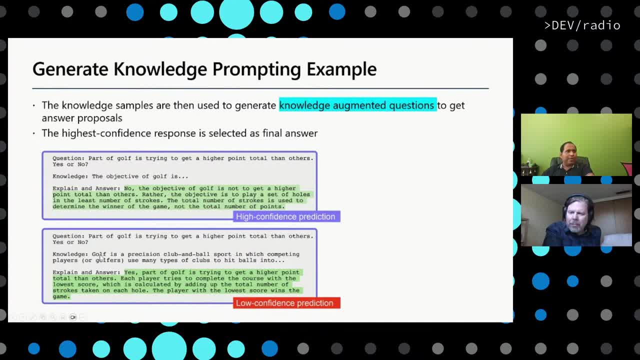 of the time to get the higher point. the same question i'm asking, yes or no? but i have two knowledge generated before then. i'm passing that knowledge. golf is a particular glove. i know the pressure and the precision club and ball sport game and all of that right. 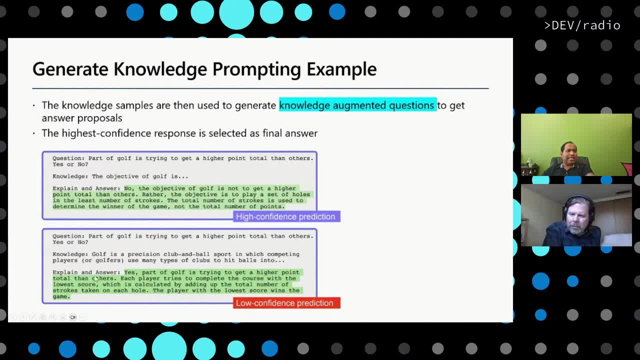 then i'm asking, based on that knowledge, the same question. then, saying the answer is yes, part of the golf is trying to get the higher point total than others. each player gets their compete with the course, like that. so both the questions and both the knowledge, i ask the same question both. 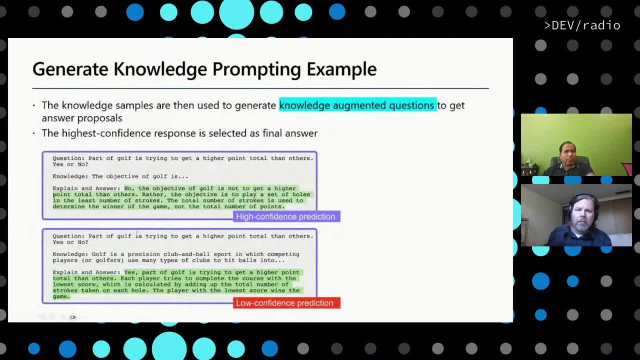 the generated knowledge and i get the answers out of it: once is yes, once is no, with the explanation right out of this- is give you the confidence which, because this one has a high confidence in some of the prediction, then this one, so it's chosen this one, right? that's called generate. 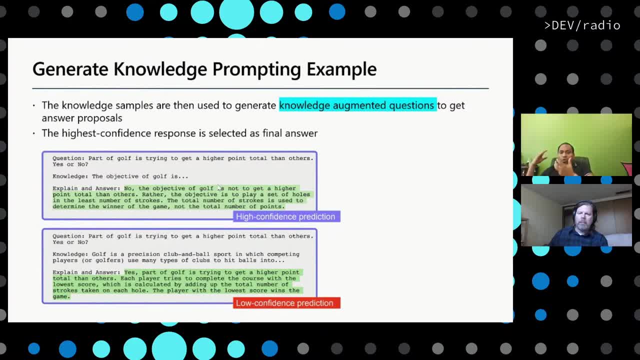 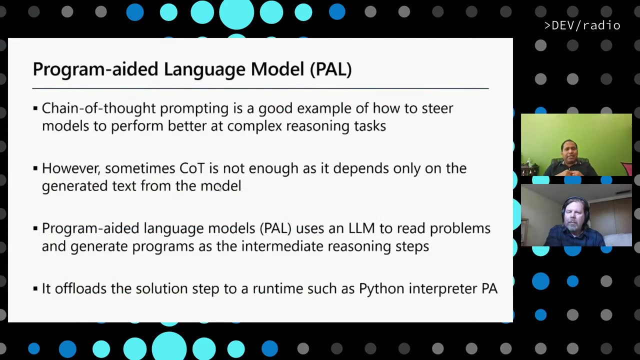 so you generate a knowledge from a given text. then you use those knowledge to actual question and see which one gives you the higher confidence for a prediction. that's another thing. next one is a program-aided language model which is called pal, which is a very important especially. 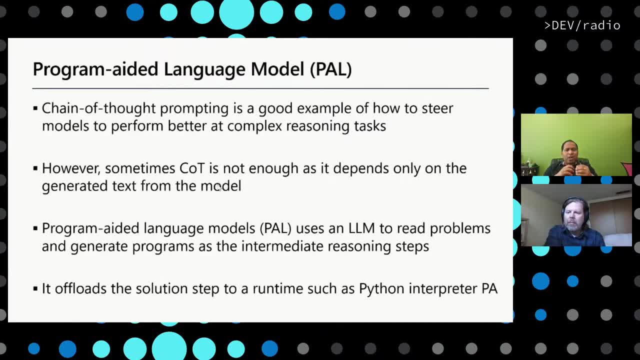 the reasoning kind of a concept where you have a lot of kind of a mathematical problems you need to show and to solve and in fact large language models tends to be more more on the right side than the ones which are on the right side a little bit, and so i think the 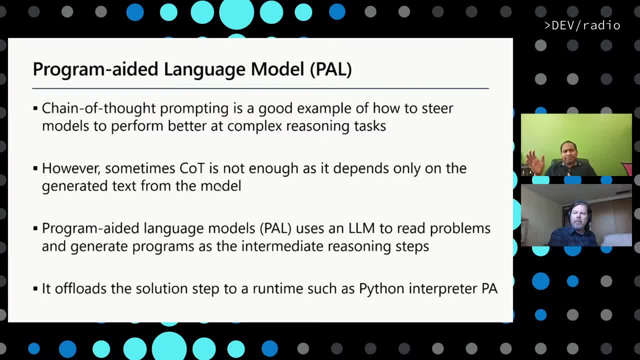 arrangements and the Everywhere models must be more. we just satisfied this program and claiming that gpt models can do a complex mathematical task as well, which was not there before, which is good, but pal is one of the. i believe they might have using some sort of pal technique behind the scene, which i don't know, but pal technique is basically it's same. 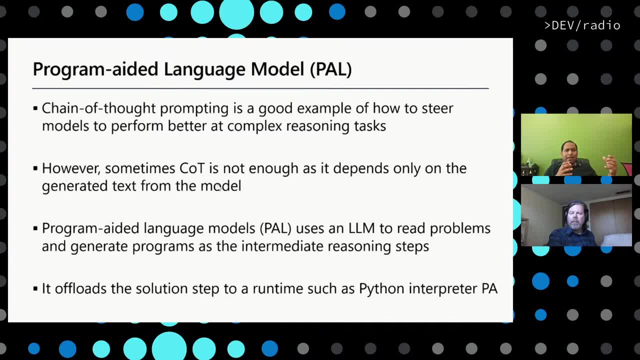 chain of thought, prompting and steer the models to perform a better reason over to give an output for a given task. but sometimes this is not enough because, especially when i say the mathematical problem, um it, it sometimes fails on that aspect right. so you need a separate tools which can 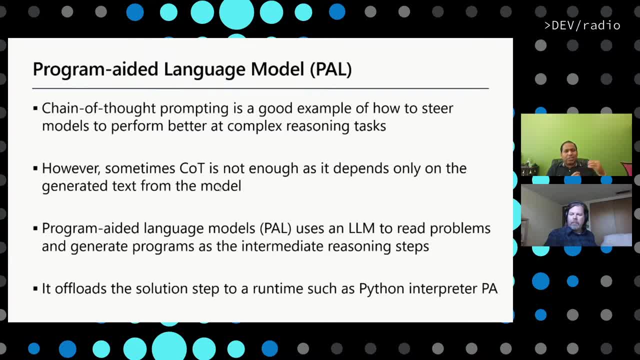 read your problem and give up actual reasoning, steps right behind the scene and it give you the actual results. right, and the pal could be a python interpreter, right. you can offload the solutions to a python interpreter tool and python interpreter will actually execute your statement or the actual problem, and give you the actual result, right. 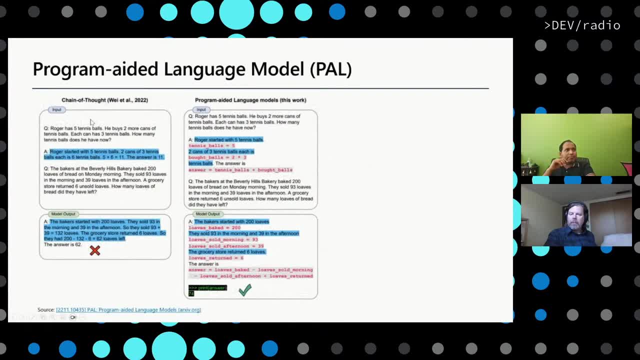 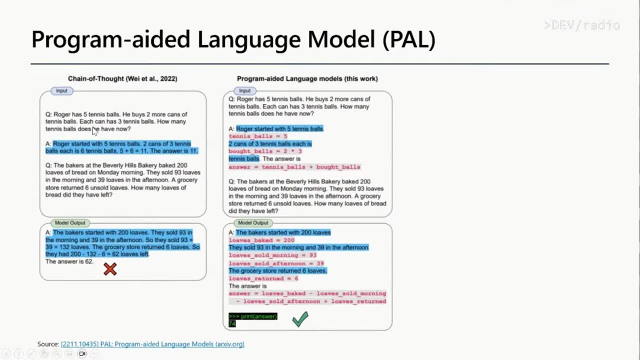 you how that looks like. for example: uh, here i said that rajan has five balls and five tennis balls. he buys two more cans of tennis ball. each can has three tennis ball. how many tennis ball does he have? now, right, even though, if i use kind of an um chain of thought, kind of an approach, you can do, 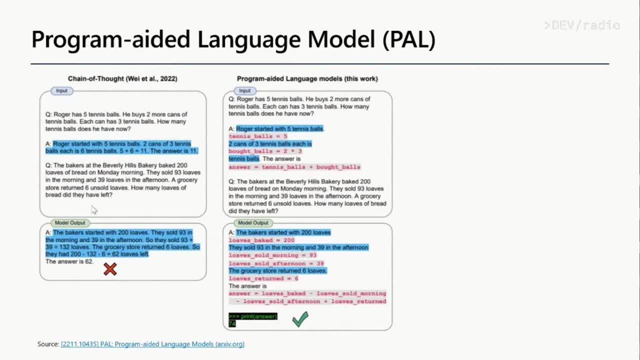 that i'm not saying in chain of thought. you'll not get the actual answer. you may get right, but here i'm talking about offloading that calculations to a different tools or a different hold together, a different kind of an um system which execute, typically execute, a literally execute and give you the 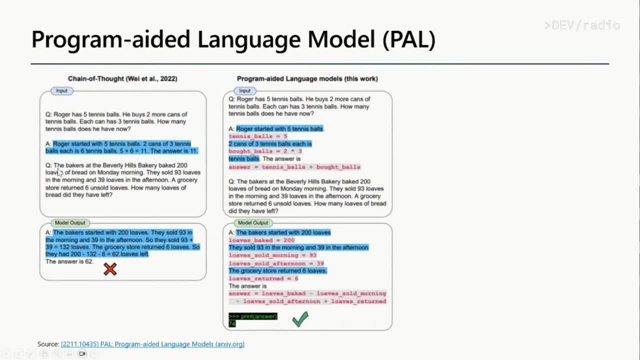 actual answer, right? so here then. um so, by the way, i'm sorry, this one is an input. i'm giving an answer for that and then i'm giving it another input and so i'll just keep on going. so in a typical chains a all in one. but here we keep on going, we keep on running. you need multiple so you don't have to run 10 Singapore business. what you do after wijayaryay is you need multiple new system. i'm not gonna write multiple new system by voice artist me anyld Seasonp. that's what hhj, hhj- I'm pence- are Ariel从. 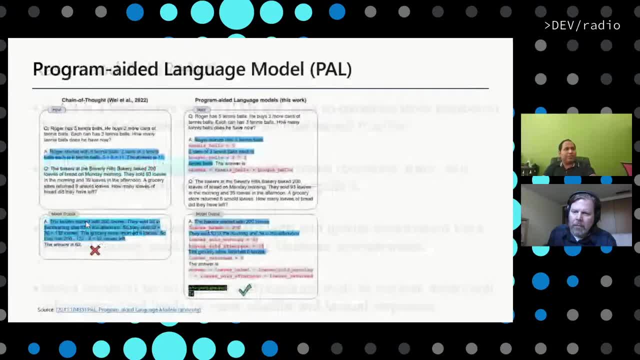 that which execute, typically execute, literally execute, and give you the actual saying, right. so here then, um, uh, so, by the way, i'm sorry, this one is an input. i'm gave an answer for that, and then i'm giving an another input and- And sorry, skip on me. 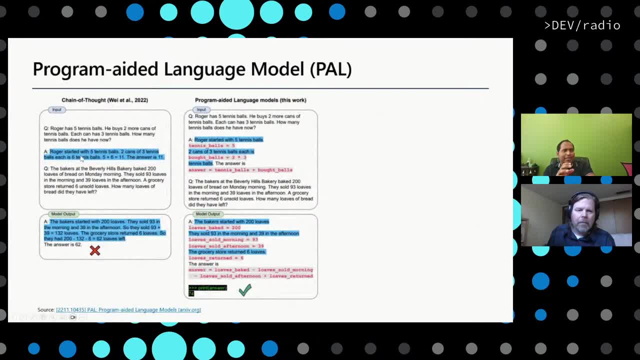 So in a typical chain of thought, I've given an input, I give an answer, I ask the question right And I'm trying to get the answer Here. the answer is 62. So you see that sometimes chain of thought fall off right. 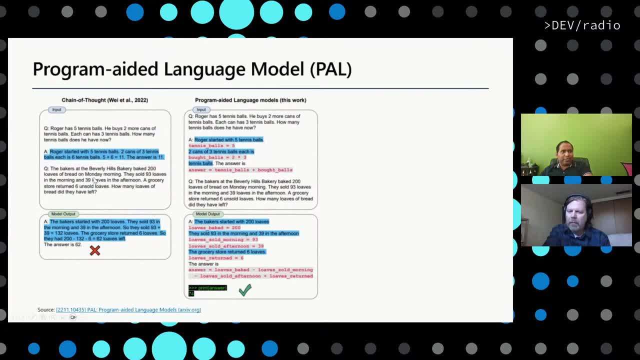 It didn't work well. The answer is not 62 in this case. specific to this example, right Now, if I do a PPAL approach, which is: you have five balls, he buys two more cans of tennis balls, which each can has three tennis balls. how many balls? 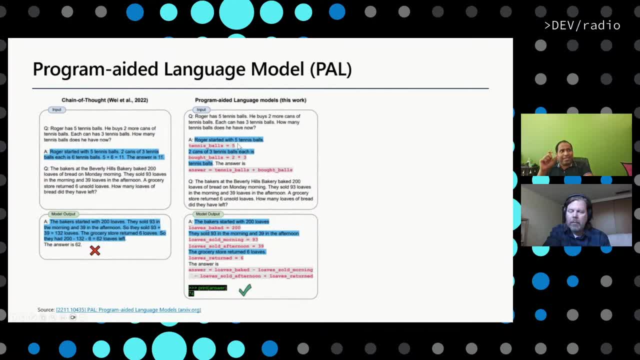 So Roger started with the five balls- tennis balls equals to five in the variable- Then he bought another three, which is two times three, and then get the actual answer. So this one, actually, this is happening behind the scene of Python interpreter, by the way. 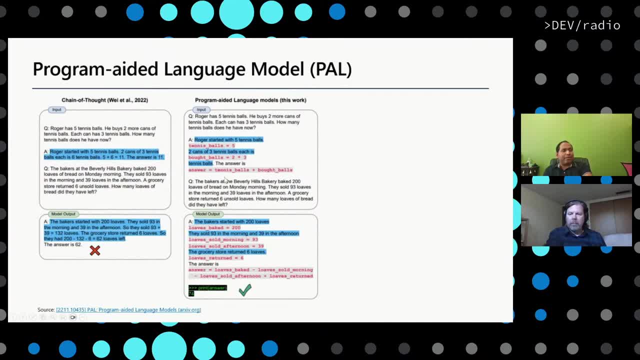 It is not happening by human, is coding that one And you will see the model output. you'll pretty understand who are the Python familiar. It'll give a sort of Pythonic way to give the answer. So, long story short, what I'm trying to message it from here. 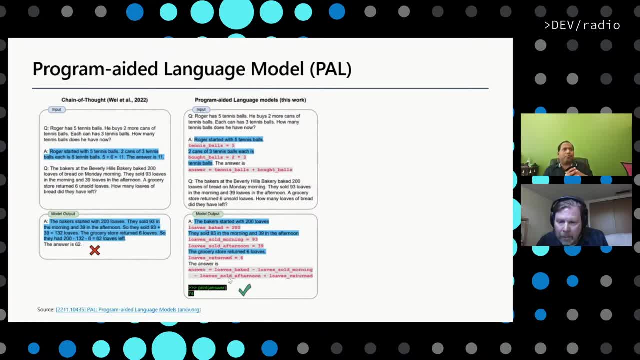 that a chain of thought reasoning is definitely a good approach. You can provide a chain of different steps which can come up with actual result. But sometimes, in a complex mathematical situation, the chain of thought might fall off, And here's the example: right. 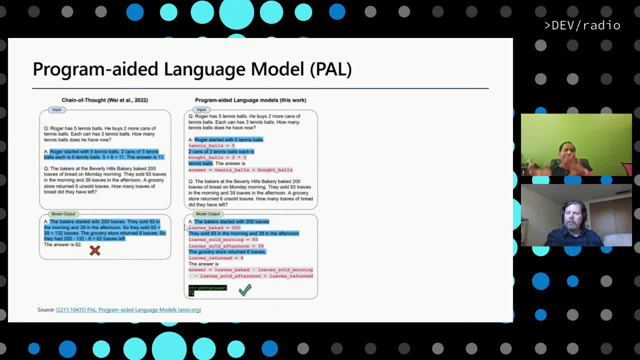 And that's where you use the PAL approach, where you are offloading the actual calculation to a Python interpreter. Python interpreter do the actual calculation and comes back to you to the actual result, And that's how it works. I hope it makes sense, right. 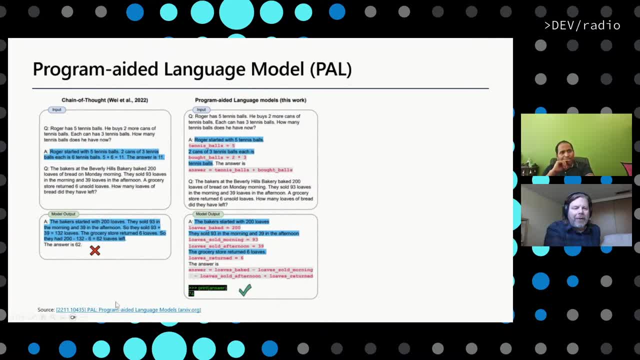 It does, It does. If I want to learn how to do that, do you have examples? Yeah, yeah, I'm going to go through some of the demos. Let me finish up the theory part. OK, just getting ahead of you here. 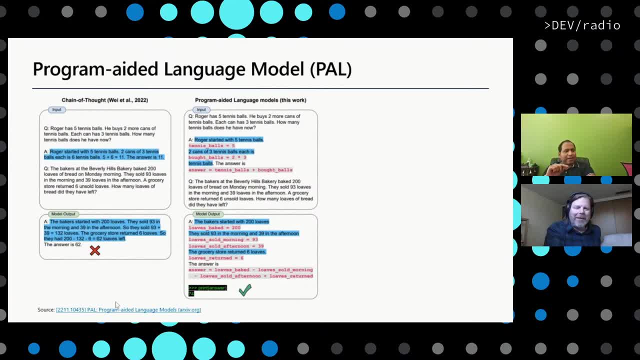 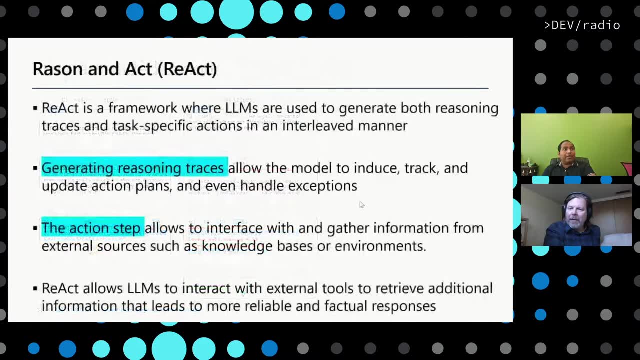 Yeah, Sure, Yeah. so here- and, by the way, this is the research paper I mentioned, which is basically talks about the PAL approach Now, reason and act. very important, And this is one of- I'll not say the best- favorite- 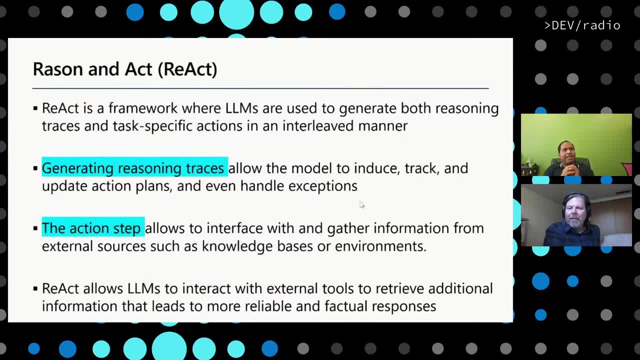 but one of my favorite: the framework, the REACT approach. right. So the REACT approach is a framework where large language model is generate both the reason and act on top of that reason, right in a very interval manner. not just one reason, one act. 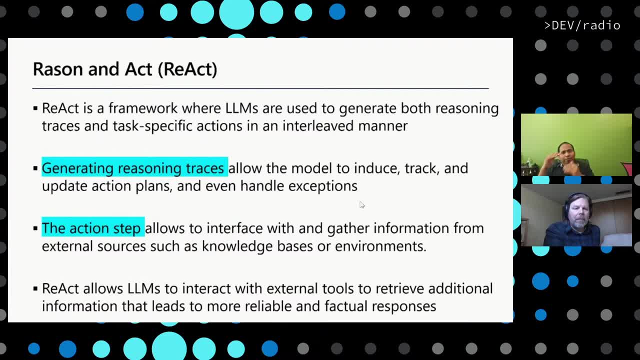 It will go to the iterative manner to come to the final conclusion. So first generate, Generating the reason traces that allow the model to induce some sort of plans of actions or what the models need to perform, the actual reason part. And on that which is called thought process, by the way, 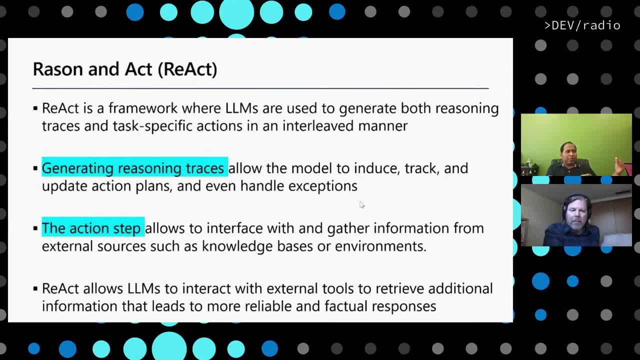 And then you take an accent on that thought process, which is the reason has been produced to come up to the actual result And REACT not necessarily has to be. it can extract some information from the website. Could be anything right. 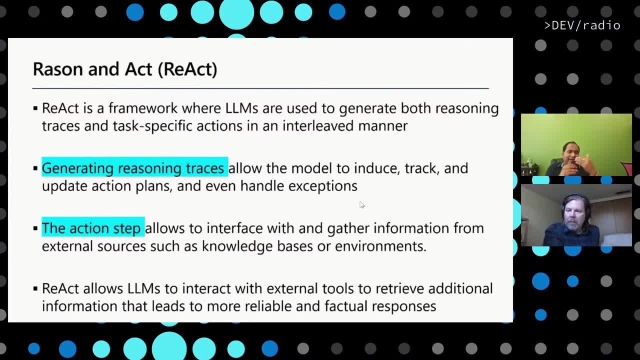 Or maybe from internal sources. With that reason and act will go along and then come up to the final result, And REACT allows more external tools to interact with. to come to the final response, And if you are familiar with the LanChain which 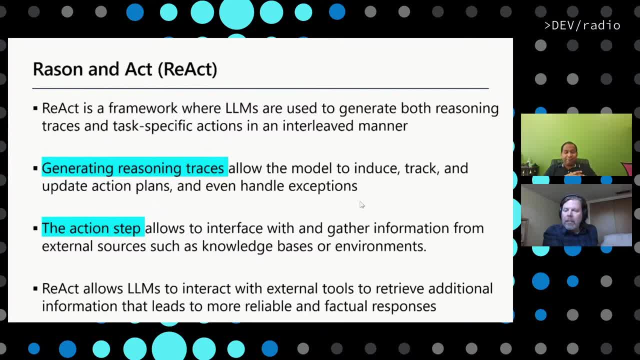 is a pretty, pretty good framework in the large language model and I'm a fan of it. they have implemented the REACT framework in their toolset, which will go to ask a question which is basically: REACT comes with some sort of agent concept. 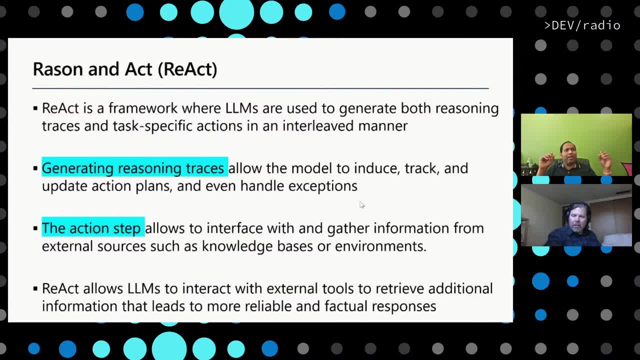 I'll not go deeper on the agent, But, in short, agent is: think about a program which is basically takes your input and it understands what's the next step. I need to perform right And how we need to perform it to understand that concept. 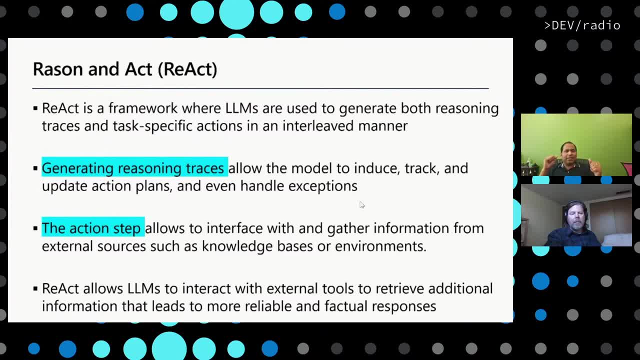 And accordingly perform it and give you back the large language model to LanChain. So I'll not go deeper on the agent topic. but REACT has been implemented, large language model in the LanChain and you can use their form as well. 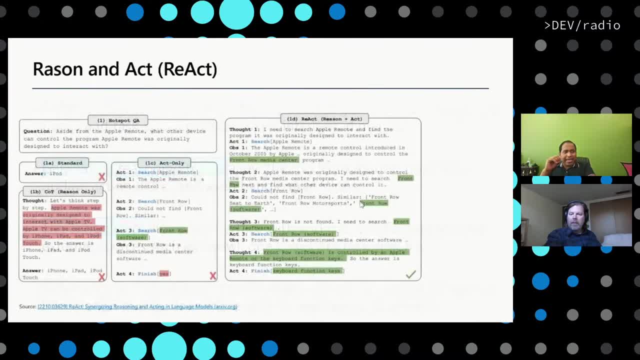 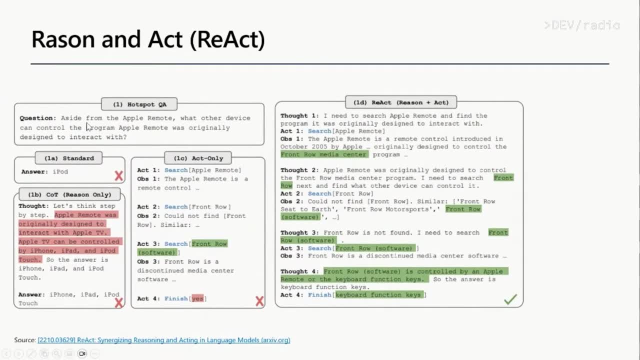 Now in the REACT. I'll give you an example here. And, by the way, this again came out of the science paper which I listed here, And this is the Hotspot QA data set. And here is saying that aside and in fact, 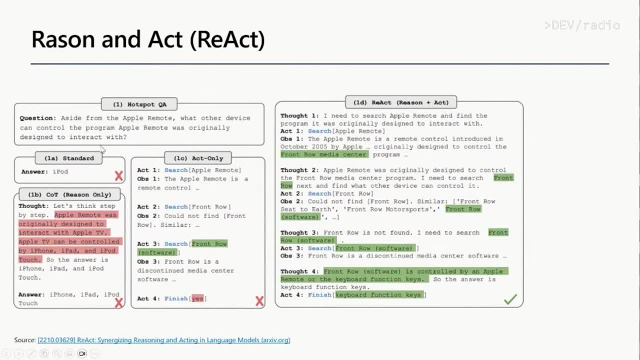 this one I've taken from this research paper, And in this research paper it says that, aside from Apple's remote, what other devices can control the program Apple remote was originally designed to interact with? That's my question If I go with the standard reason, not the REACT. 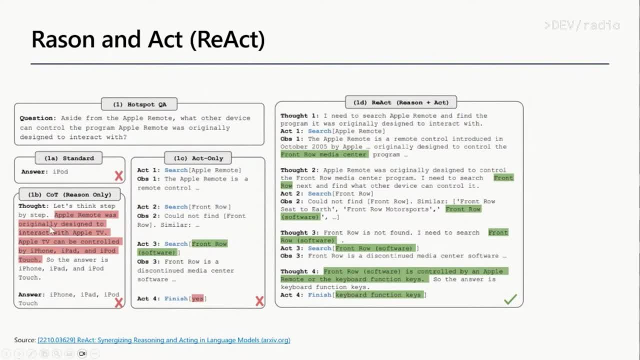 on the right side. Just don't focus on this right now. Just focus on this particular segment. This is the standard reason only kind of a chain of thought. So thought I say that let's think step by step. If I add that, what will happen? 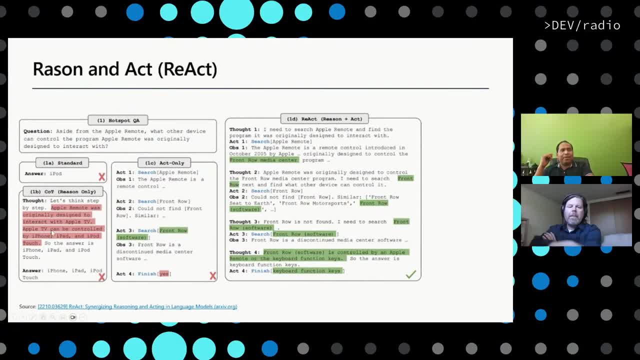 Apple remote was originally designed to interact with Apple TV. Apple TV can be controlled with the iPhone, iPad and iPod touch. So the answer is iPhone, iPad, iPod touch, right? This is wrong because this is just reasoning right. It is not taking an action on the reason. 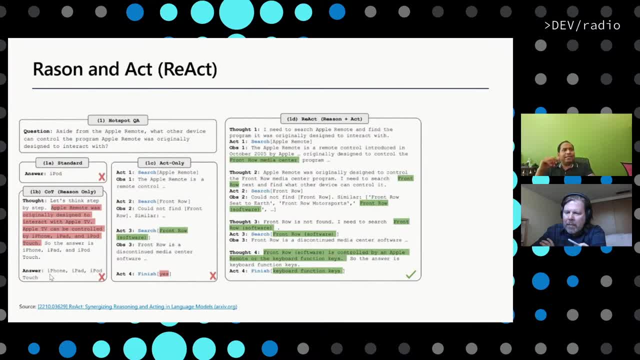 Whether I'm reasoning, is it correct? I don't know. I'm just taking a reason. That's a siloed reason. Now, if I just take a siloed act on the approach, I say OK, search. 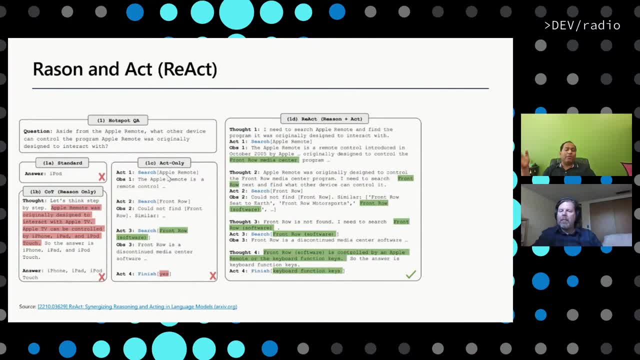 I'm searching and this search could be anything. As I said, REACT can work with the external sources And let's say I'm doing a Bing search, for example, as Apple remote. What I get? an observation. That's my actions. 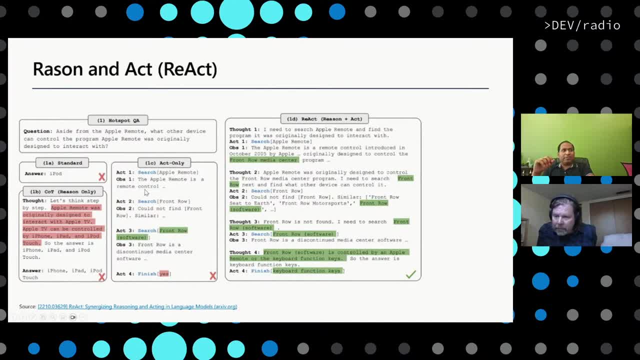 An observation is that Apple remote is a remote control. That's my observation. Then I do the again: search front row, because I did say that what other devices can programmers or engineers design? Then could we find front row or similar language? 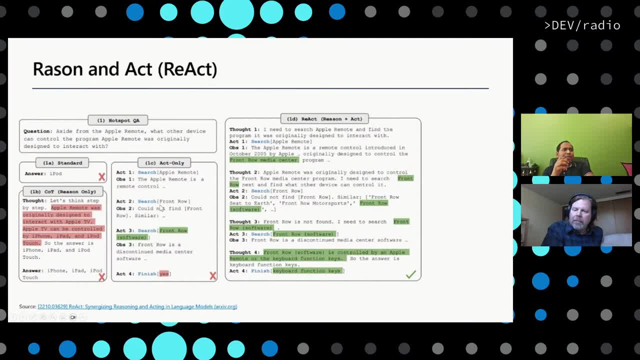 So what I'm trying to say. the second example: here it's multiple things. you can search through, right, And you can give the example So you can act based on the observations. right, You act, this one search and you get an observation. 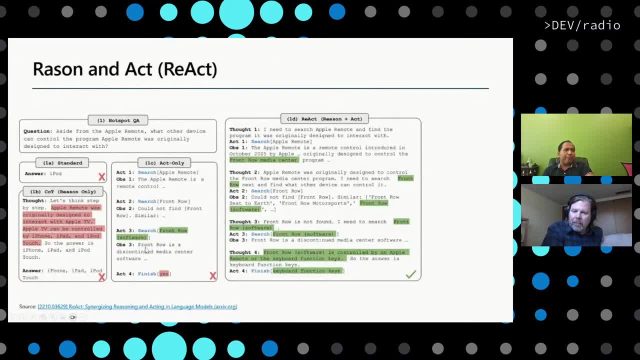 So you search something different, you get an observation, You ask something: front row software, front row software and this kind of media center- Then you finally finish it with a yes. So is that the answer? The answer is: the Apple remote is designed for interact with. 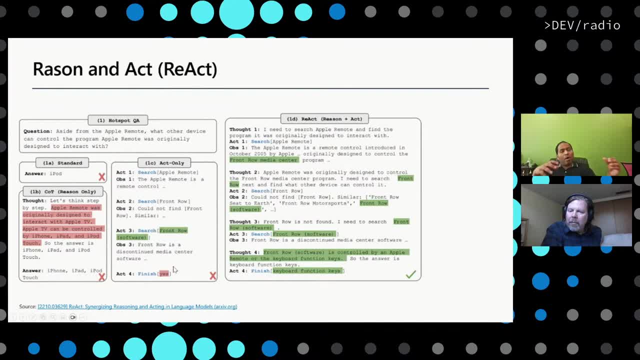 And the answer is yes, right, Which is also not quite correct. Now what the paper is saying, that we can combine this together. not only do have a siloed reason and the siloed act separately, let's combine this together and come as a react. 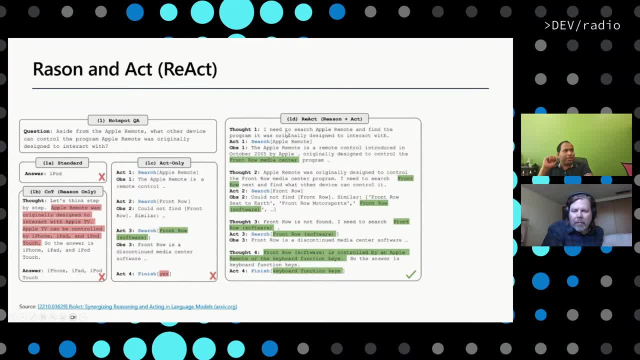 which is reason over act. So first I need to say that thought process, First I need to search Apple remote to find the program it was originally designed to interact with right And the action is it's going. maybe a Bing search. 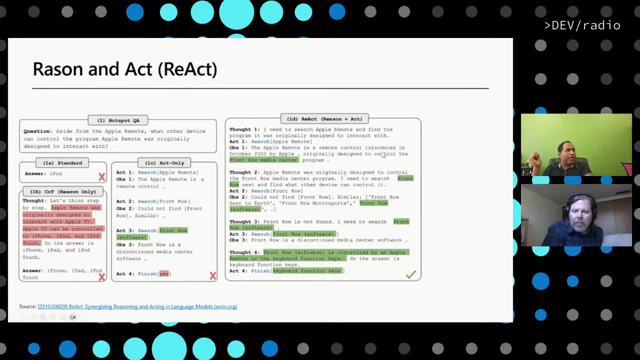 and it's coming out this observation: Apple remote was the remote control introduced in 2005,, originally designed to control the front row media center program, right. Then second thought process: go and it's a chain and it's not just somebody. you have to manually input it. 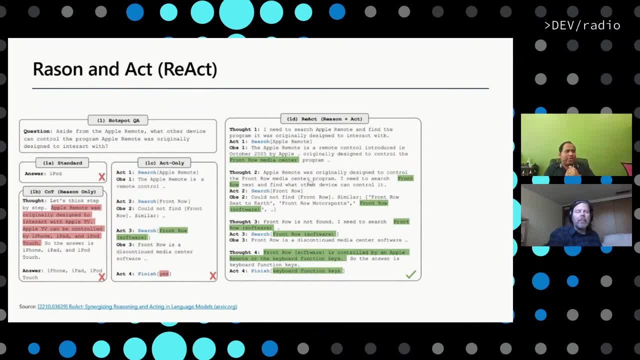 It's go to the second thought process And, by the way, this goes by the agent concept. by the way I was talking about Then, Apple remote was originally designed to control the front row media center. That's why it's coming in the first thought process. 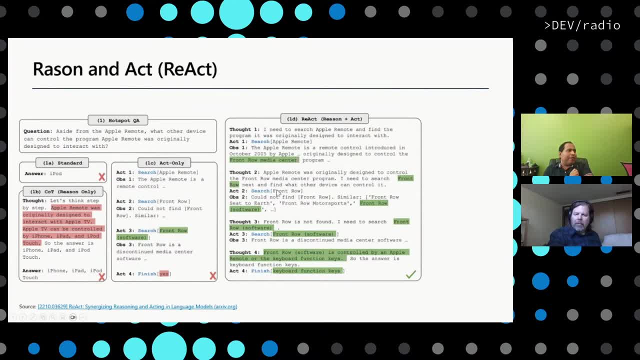 The second thought process goes on that right Front row, And again do the act on that. Then third observation: goes on that and keep on going And finally, in the final thought process, you can say, okay, front row software is controlled by Apple remote. 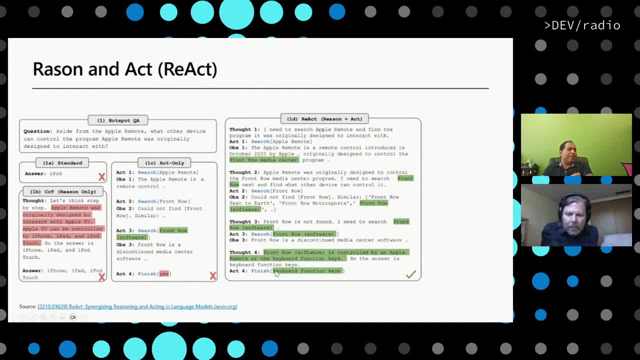 and the keyboard a function. So the answer is keyboard function, keys and the keyboard function. That's the final answer. So it goes to a multiple thought process, the observation which is basically your from the thought process, You are taking an accent on that. 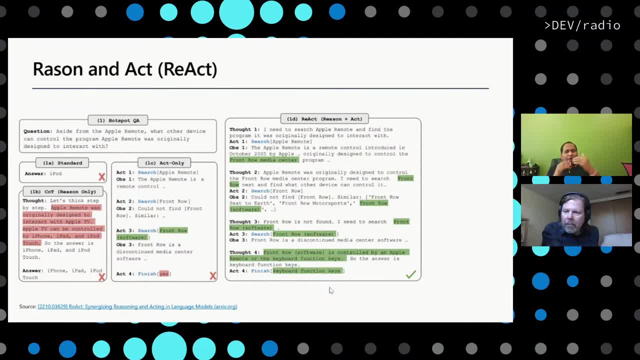 Again you go to the observation, thought process and action. So it's keep on iterating through that and give to a final conclusion, rather than silo to this one and that one That's called react. So it's basically the reason and you get a reason. 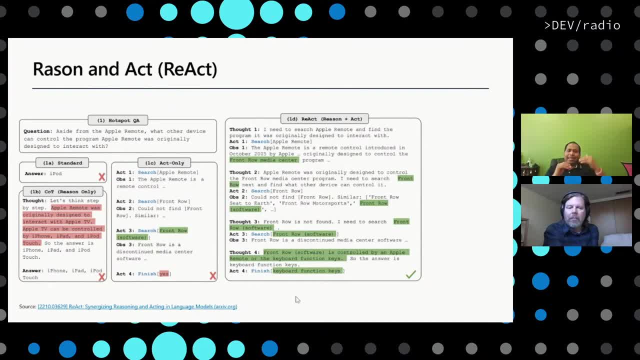 you observe the reason, you take an accent on that reason, Go again and again, and again, and then you conclude to a final conclusions. right, That's what it's called react. Good example, good example. You had a lot in there, very concisely, actually. 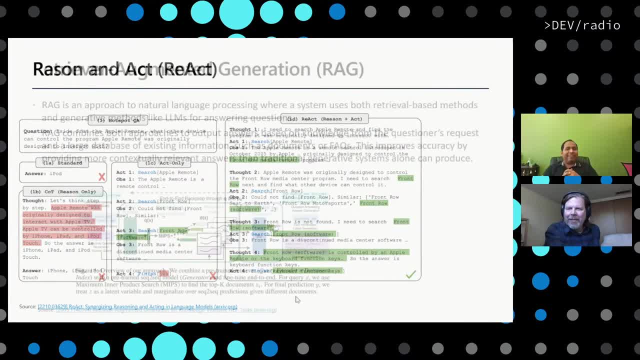 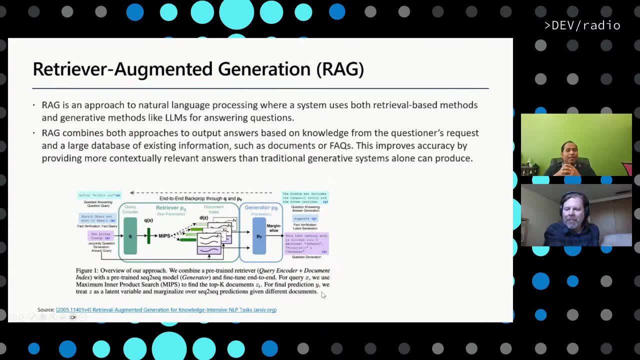 You did a lot of things And this is my favorite retriever- augmented generation, which is called Rack, which is also came out from this research paper And the reason I'm saying favorite, and I'll tell you a practical examples of the Rack. 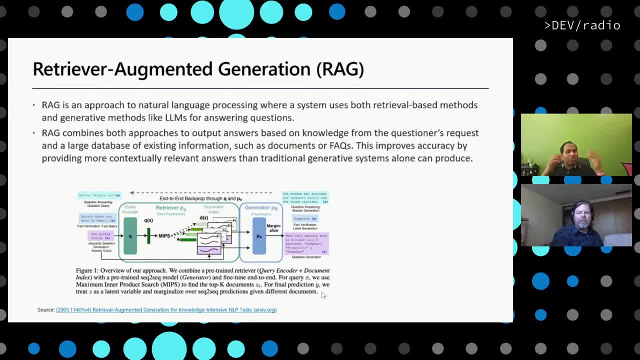 so that you will understand why it is favorite. And most of the enterprises have some common questions. Let's park that common question. Let's talk about the Rack, and I might think: why is this guy talking about without explaining Rack? Let's make this. 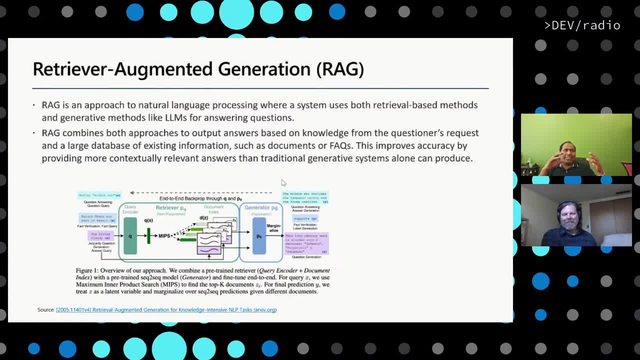 Okay, So Rack is an approach where the natural language systems, basically the process system, both uses a retriever based and a generator based method to give you the final answer, right? So what it does is basically- and again these things are taken from the research paper- 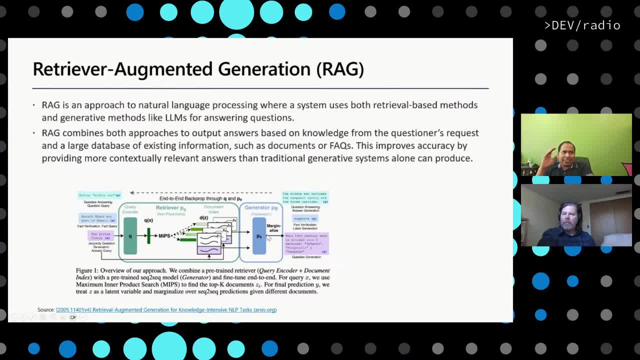 You have a two system sitting together: a retriever system and the generator systems. What this does is the generator system is basically generate- think about a knowledge right. It generate a knowledge and store somewhere right- Somewhere- We'll go more deeper- where it can be stored. 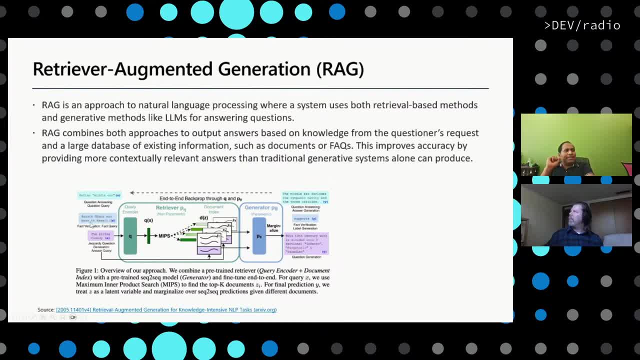 but somewhere it's stored right. And the retriever knowledge, which is basically the sorry retriever system, which basically you ask a question and that retriever knowledge, they said: okay, I have a question, I need to search that question from the retriever system. 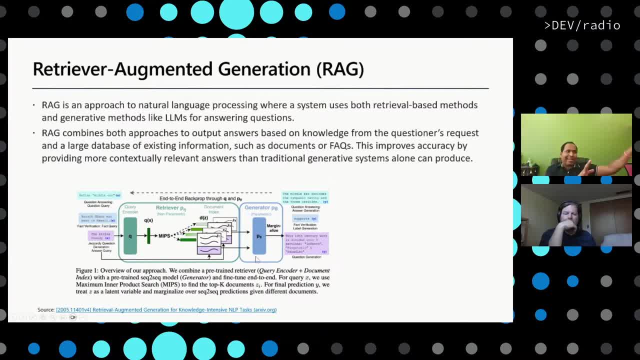 So it's from the database where generator has already created the source code. Then go to that source and give you the answer. right? So that's called Rack. You have two systems: One system generate the knowledge and other system based on the user input or the prompt. 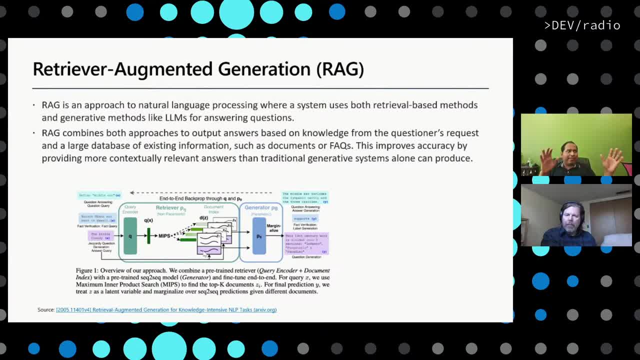 is trying to get the answer from the knowledge. That's called Rack right And it's pretty common, such as question answering, use cases, Sort of Even, in fact, In fact, some of summarization. I've seen that use case as well, but more typical use. 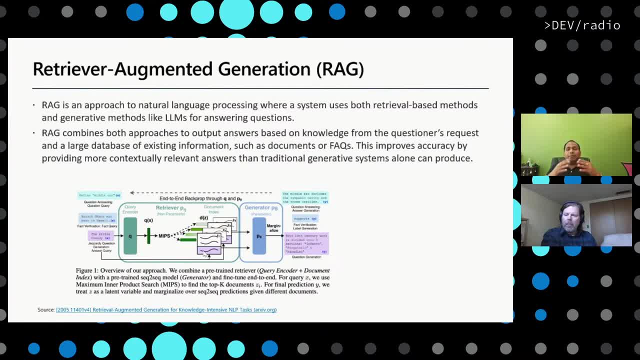 cases. question answer. In fact, which is true, and I'm serving HLS customer and in fact all my HLS customer use case are question answering from their corporate documents. So they don't want- and they have a lot of confusion- that hey, chat, GPT has been trained. 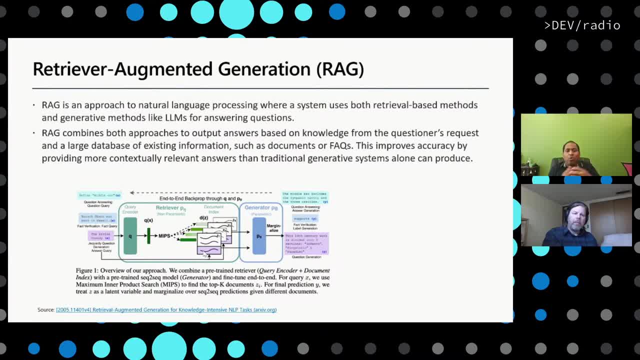 on the public data set, and if I provide my own data, is it going to be trained- the models by my own data? No, HLS, and I specifically- does not use customer data to train the models. We do not do that. So then, how I can use my own data to question and answer? 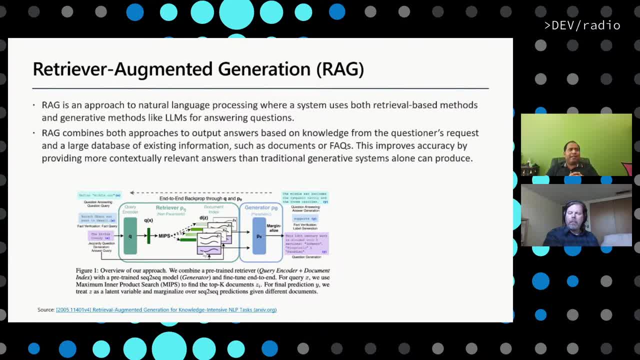 What is the mechanism for that? If you don't use train the data, should I have to do the fine tuning? Should it means that I will take the base models from you and I provide my own data to fine tune it? No, 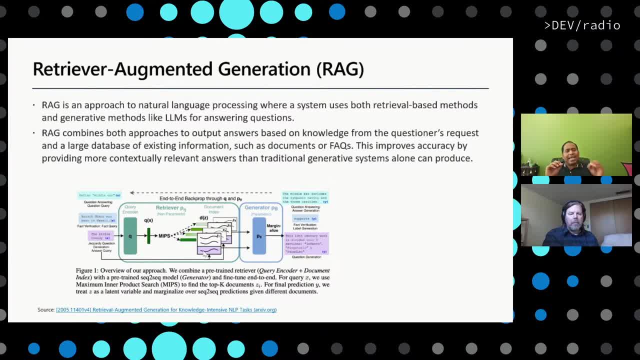 Fine tuning. we do not recommend to use it unless it is really really, really important. It is really super needed And I have not personally found any of my customer is doing fine tuning yet right Now. you might be questioning: okay, what is the difference in fine tuning and the rack? 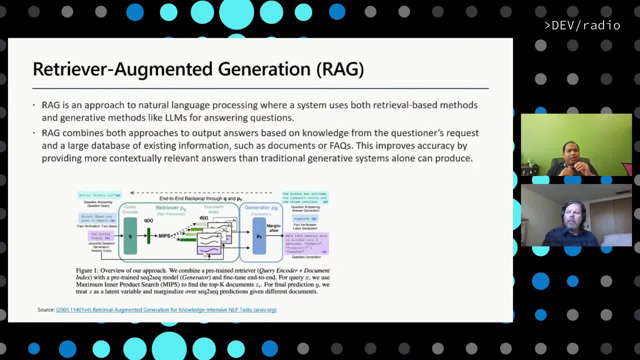 right, If I don't have to do the fine tuning, why do the rack So the fine tuning is? think about. I'll give you an analogy. right, Let's say you went to a school from grade one to grade 12, you studied math, physics. 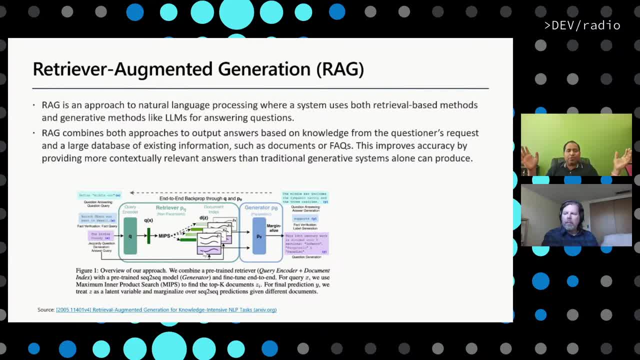 chemistry, biology, all of the different things right. So you are knowing many things. That is typical pre-trained model, which is a base model, came out of genitory open AI. It has many things right. Then you go to a college and you basically give me one second just some background noise. 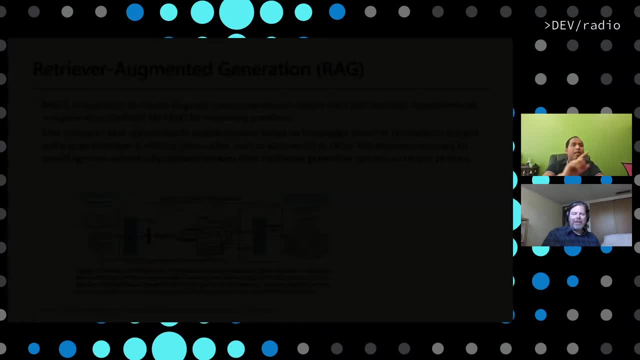 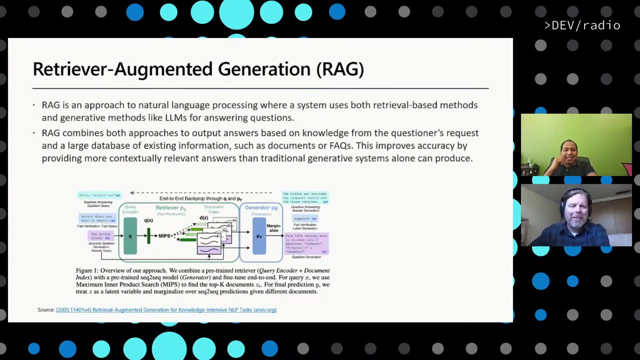 Just a second, Okay. Okay, I'm asking my daughter to skip silence, okay, Sorry about that. Okay. So what I was talking about, yeah. so after you've done the grade one to grade 12, you basically go through all the things and that's called pre-trained model. 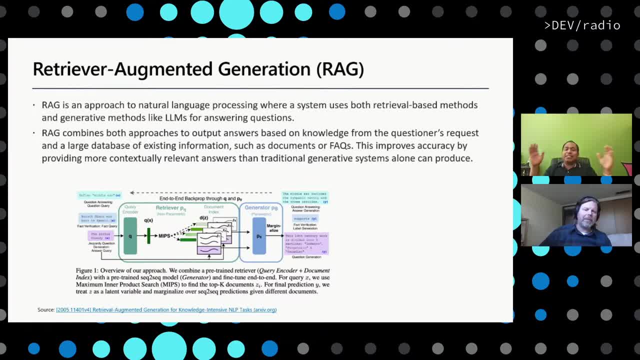 Then you went to a college and you studied, let's say, electrical engineering for four years, right? So this four years, you are specialized only to electrical engineering, even though you know the fundamentals of all of the things: science, biology, math and physics, all that. 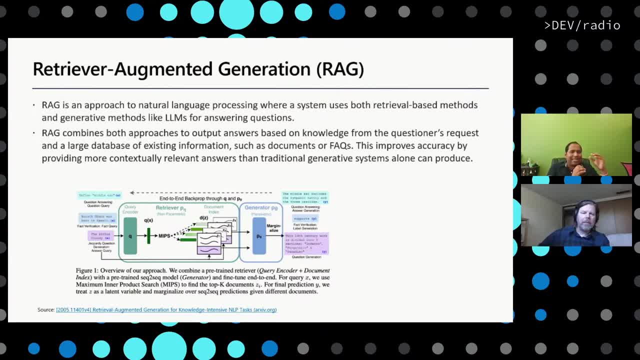 But the four years you only do electrical engineering- That is called fine tuning- means you are specialized to do only electrical engineering, nothing else, right? So in your term, if you want to do a sentiment analysis from your textual document, then 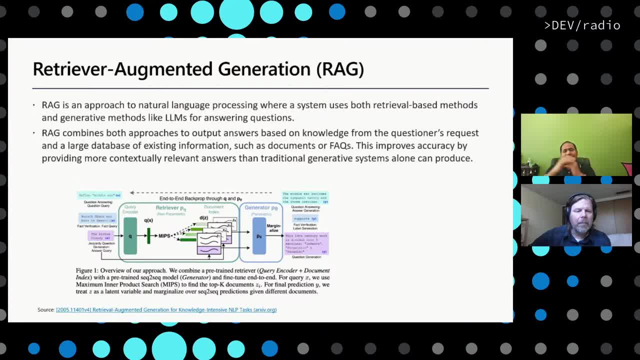 you can fine tune your model and provide lots and lots and lots of information, Lots and lots and lots of examples of your actual- you know the sentiment like text, sentiment, text sentiment like that right And that example. so you can feed into a large language model to fine tune it and there's. 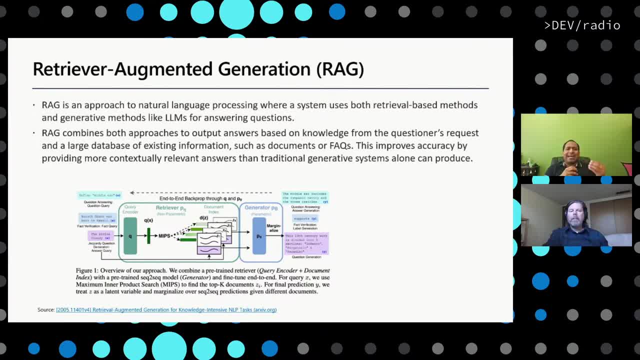 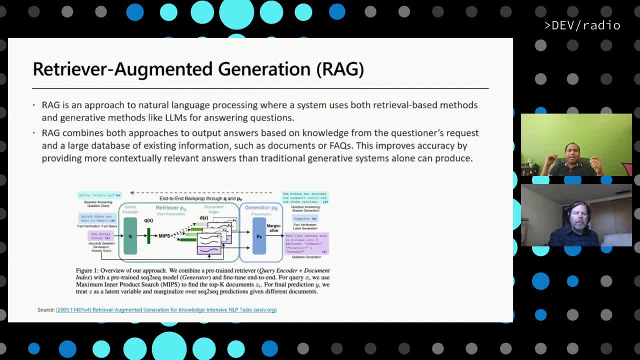 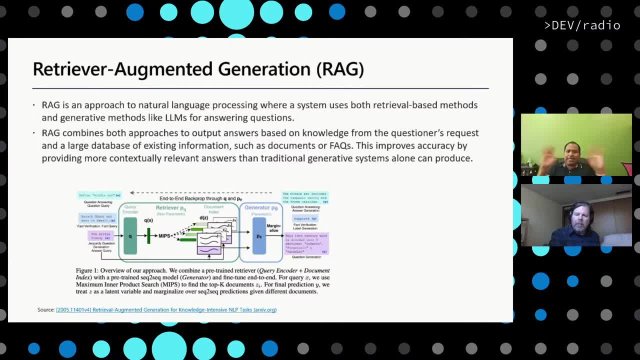 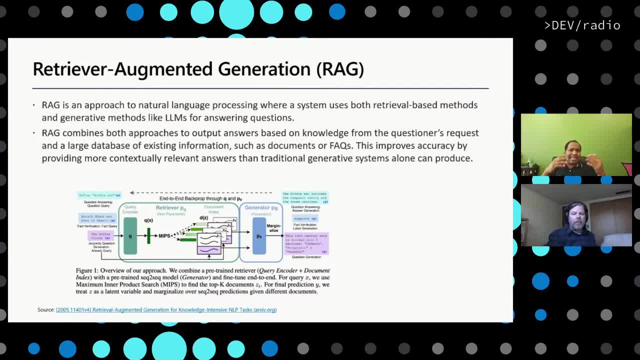 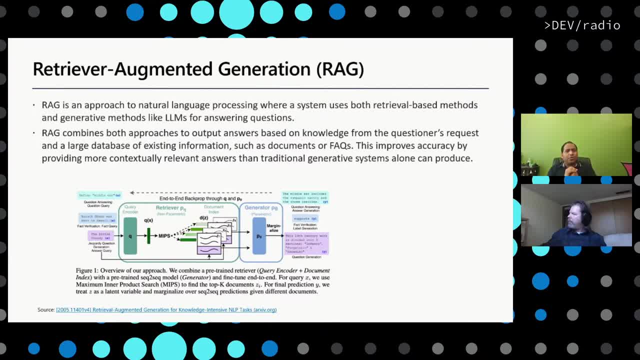 So it's very hard to tell where the answer source from, whether it is source from your fine tuned data or is it source from the actual model, internal pre-trained data. You don't know that. It's very hard to cite it that way, And that's where the rag comes into the picture, which is called retriever. augmented generation means that you have a source of document. You don't go with the fine tuning, You store it with some sort of database. You ask a question, give back the answer, Right. 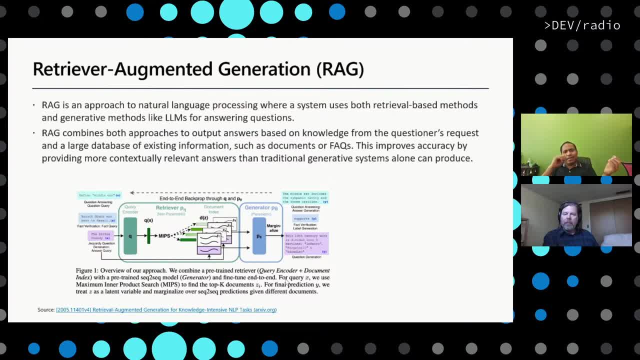 And that way It is. basically, if I take the same analogy of the electrical engineering, after four years of electric engineering you went to a job and in the job, every day you are learning new things. It's not just: you know four years of electrical engineering things. you learn Every day you are learning new things, new tips, new techniques. You cannot do every time fine tuning, It's not possible And it is not appropriate, not logical. And that's where that's where it's used. 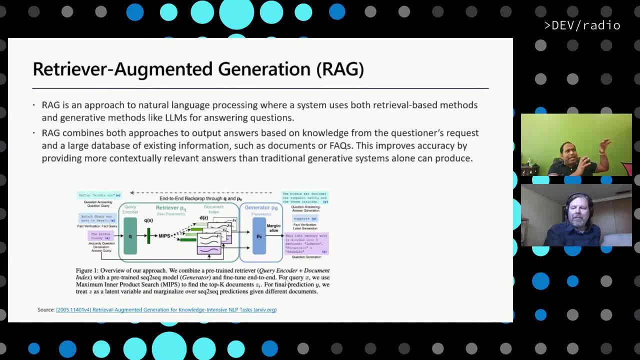 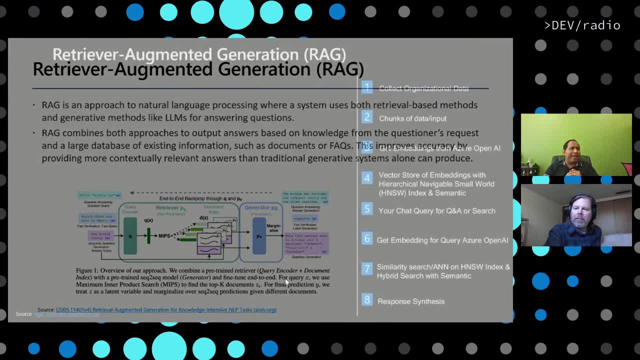 The uh, you basically all This knowledge you are generating you put towards some sort of knowledge base and you retrieve as and when required And in practically. if I ask how that in Azure, open AI? think about this step right. 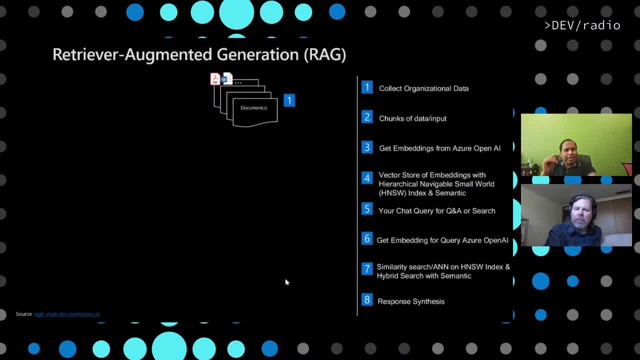 First of all, you have a lot of internal corpus documents. You have that one and then you chunk it up. Why it is chunking? Why I'm chunking this up? Chunk means a smaller version of this tech. The reason I'm chunking is two reasons. 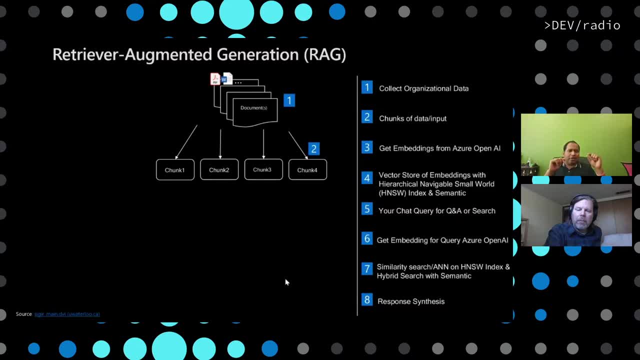 First reason: every large language model has some sort of token limit. For example, GPT 3.5 has 4096 tokens. GPT 4 comes with a two flavor. One is the 8k token and 32k token. 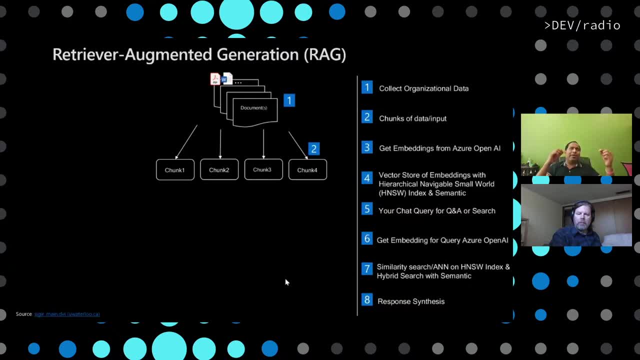 Right now, what is this token? I told you before tokens is. think about it. could be one word, could be one token- It's a numeric representation. or could be one word, multiple token. Now, if I ask you, um, for example, uh, I want to generate the knowledge of those documents. end of the day. 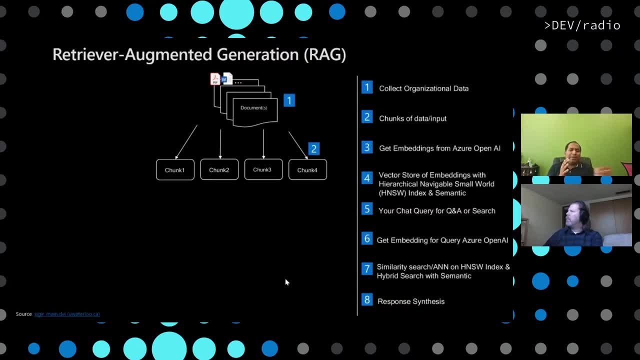 I need to get the uh uh numeric representations of the data. That's how I need to do, But I cannot feed the hundreds and thousands of pages into a single API call because there is a context issues right, I cannot go beyond certain code. 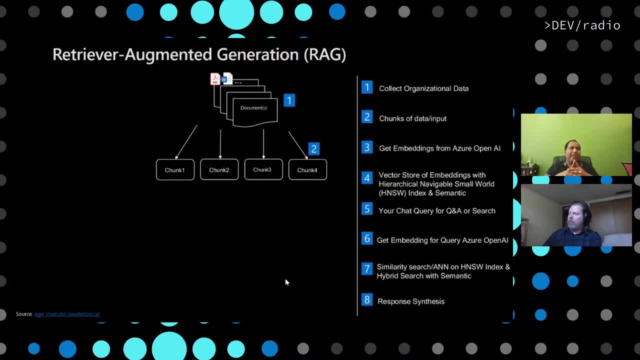 That's okay, Let's. that's the reason you need to do the job. And second reason, which my favorite, is that if I ask you that, Hey, you need to go for open book exam, And if I give you a hundred page of pages of book, no, uh, think about no, index, nothing that. uh, if I ask you a question from that, what are you going to do? 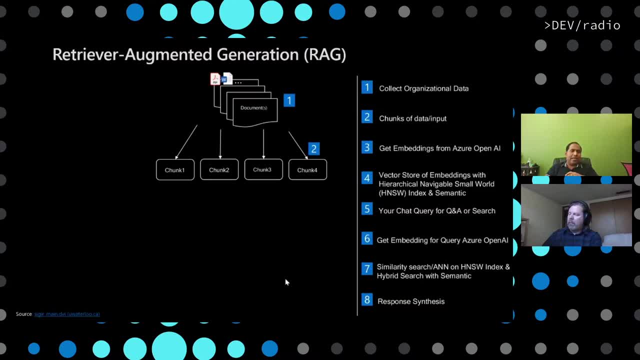 You have to search Almost all the pages to give you the right answer, right, Which is not efficient. However, if I give you uh one page from that hundred page and ask you a question, it's very easy because you are searching the question of: uh sorry, searching the answer of that question from that page only. 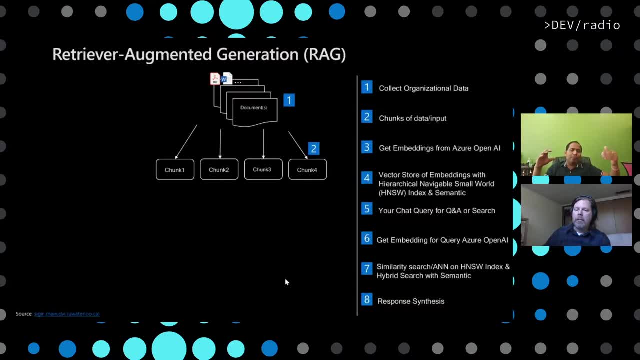 Right. So chunking it makes first of all removing that token limitations issue And second thing is much more efficient to give a very contextual answer from that given question, because you know I need to give an answer from that job. 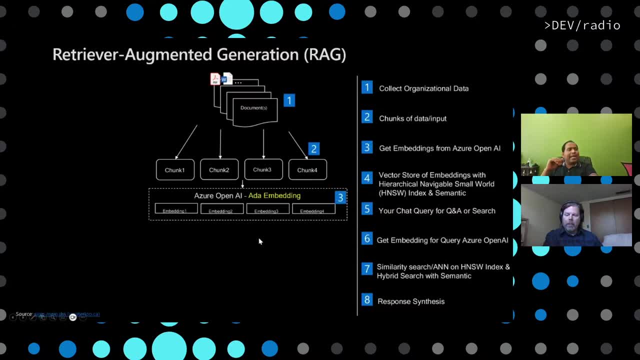 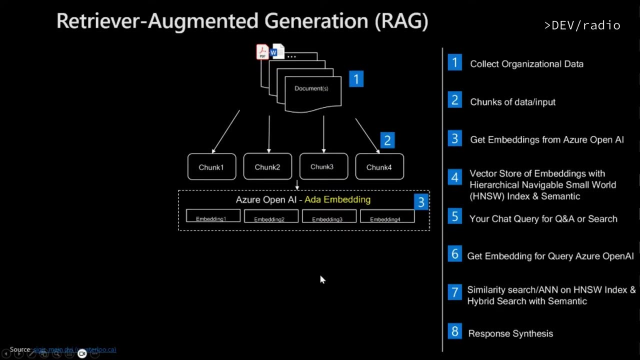 So that's the reason you do the chunking right, And then, um, you use some sort of open AI embedding models, which is called RDI embedding. What is everything embedding is? think about uh numerical dense representations of your text to uh end dimensional vector space. 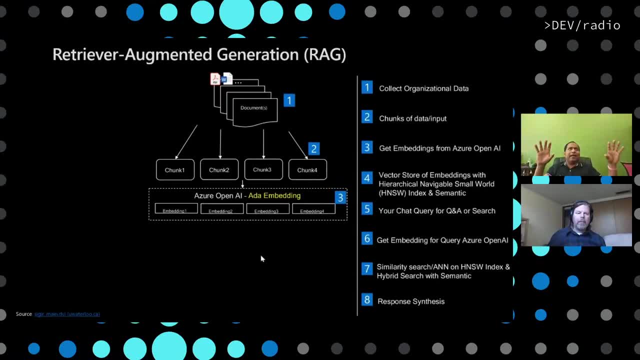 I know it's a very mouthful, but that is that. that means that, um, you create some sort of numerical representations and that representation you plot to a vector space. That's it. That's it, dense representation, by the way. 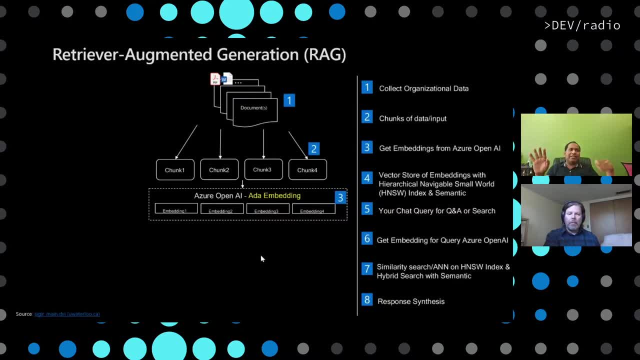 Right, Um, why? why I say the dense representation? because there is an another uh vector called sparse vector, right, So, dense vectors, sparse vector. I'll not go that deep on that, but there is a sparse vector which is lot of zero values can be exist in the sparse vector. 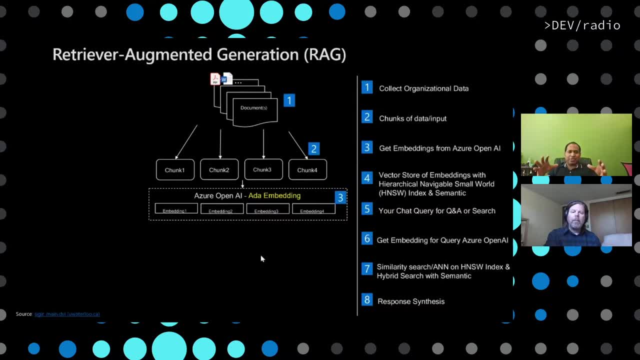 And dense vector is. a lot of non-zero values can be exist on the vector That's called dense vector And the dense vector is more. think about a contextually, Uh, semantically, you know, correct, uh, context can be produced by the dense vector, right. 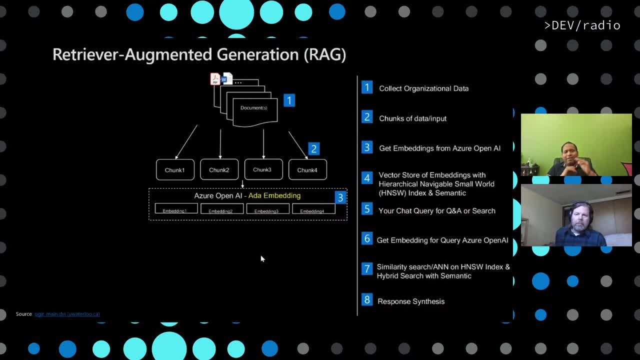 Um, there is a use case where you need sparse vector. We'll we'll go maybe in a later talk session on that, but in short, you created a dense vector using an RDI embedding model And then you store that into a vector database. 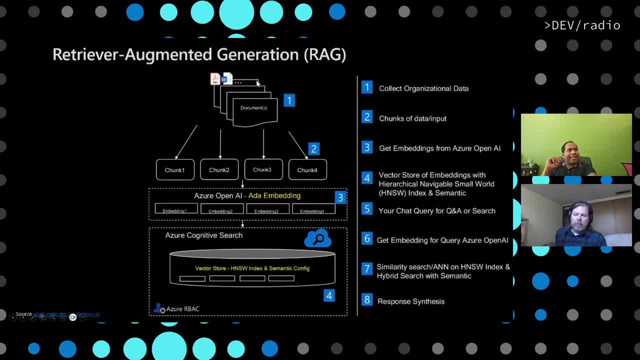 In that case, Azure cognitive search, you store that, embedding This whole piece which I just talked about in a rag approach That is called generator. This system is generated, You are generating the knowledge from this corporate and you are storing somewhere which is Azure cognitive search, right. 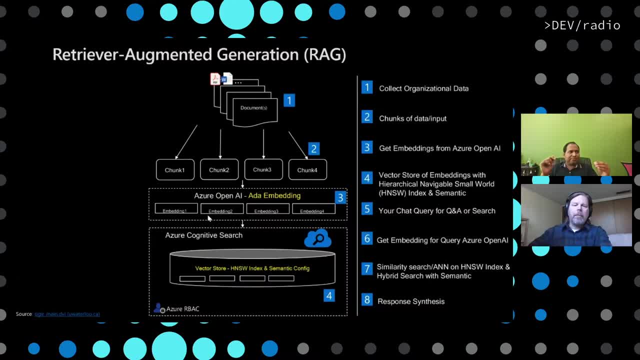 I hope it's clear up to that which is generator, Is it okay, Matt? Okay, They had myself on mute, Sorry, Yes, Okay, Great, Great. So that's called generator piece. Now we're going to talk about the retrieval. 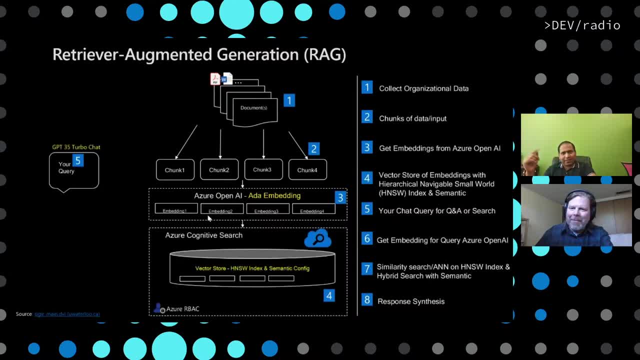 Right, We talked upside now here. Now you ask a question. let's say, in this case, 53.5,. this goes to the same embedding model, because you need to get the same sort of numerical representation. And then you search from your generated knowledge using a cosine similarity, right? 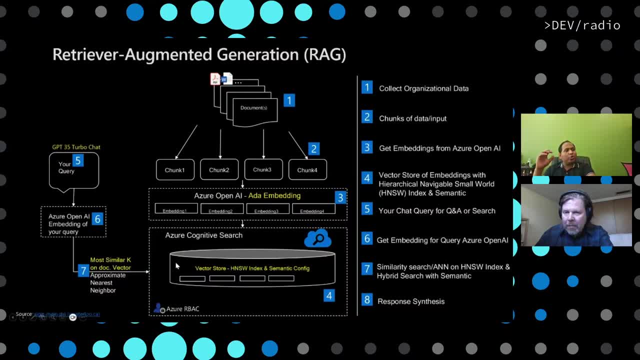 And you return back that actual contextual chunk which can suffice this answer, that contextual chunk, then feedback to an open AI completion And then you search from the same endpoint and generate back to the answer. So this piece is a retrieval, that is a practical implementation of that generator sitting. retriever sitting. 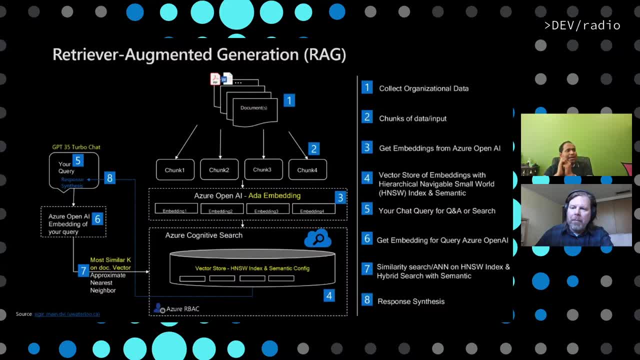 You get the answer. The best thing is there is: um, you get a citation. means that now if you ask that model to ask a question, it can cite a answer, because now it has a different chunk right. It can say that for this question. 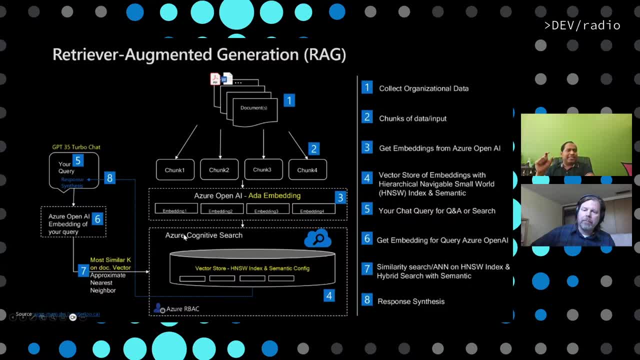 Maybe pdf number one, pdf number two and pdf number three. three is basically citing the answer and i'm gonna give you a demo on that so they'll better understand. so with that rag metro you can- basically you are grounding your model to answer the questions for your own data, even though open. 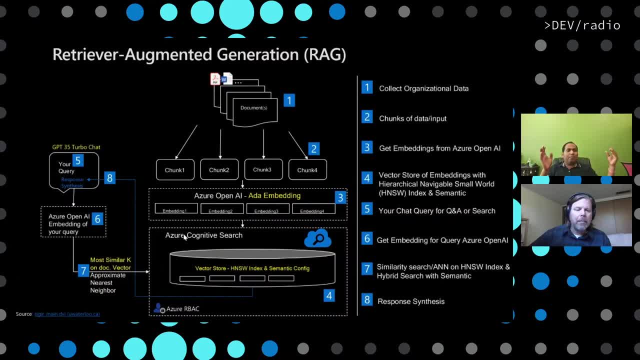 the rgbt model has been trained on the you know billions of corpus and open data and all of that, but it is not known about your data and that's where you can ground the model to generate the answer from that, and this is a very fantastic approach to ground the model and generate the. 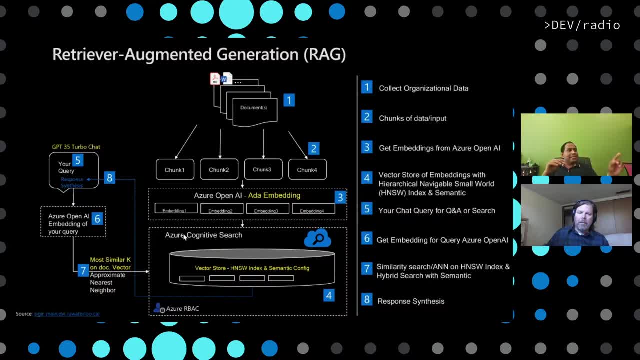 answer from your data rather than fine tune. this is very common things, and all of my customers are using the rat rag approach to generate the question answering from their own internal corpus document. right now let me give you a quick demo on the rack right so that you better understand. 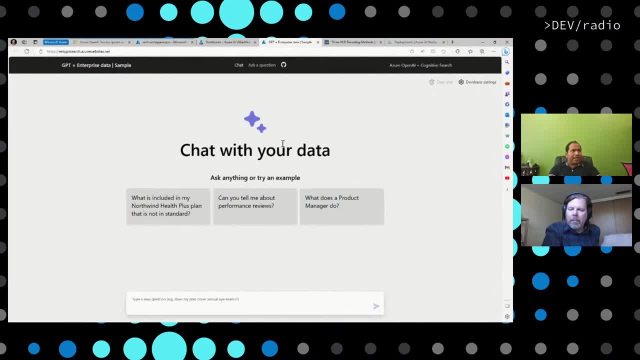 for example, in this one it's called chat on your data. it's an enterprise, uh, data here, uh, behind the scene. i have already generated the knowledge base, which is the generator part means that i have a set of different documents which have gone through a chunking method. use the numerical representation of the 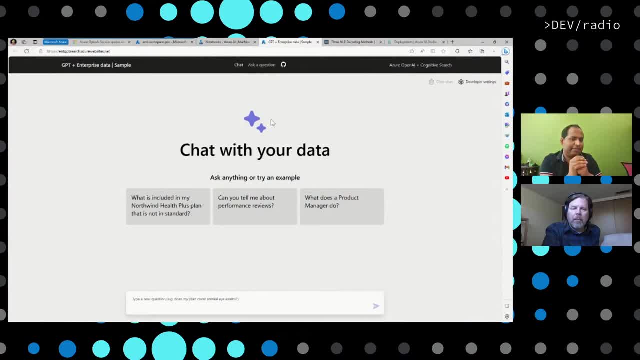 chunk and then store into a cognitive search vector database, right, i'm sorry, the cognitive search in this case. i haven't used vector devil, but if you want you can use that one. and then i asked a question: right, what is included in northwind health plan? that is not standard. 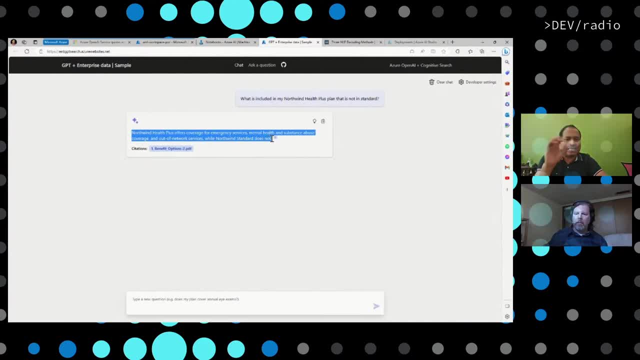 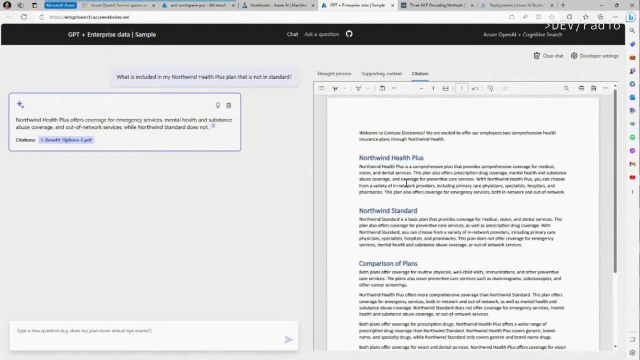 right, you see that it gives me very precise answer. that is a retriever piece, right, and it's cited. this as well. it's cited. okay, this is the actual pdf document has been used to source this answer. so, as a responsible ai or um principle of responsible. 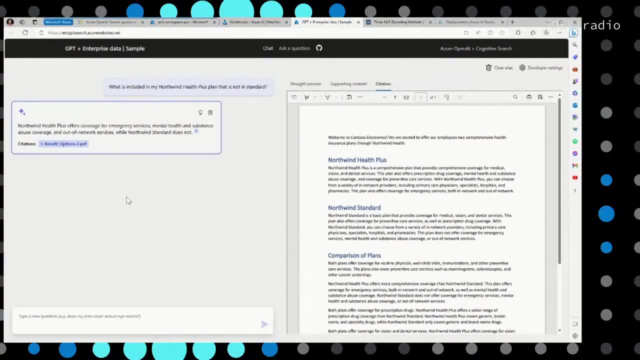 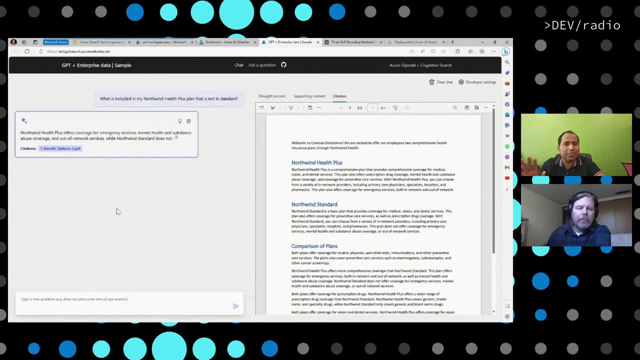 ai is. you always need to show your you know the where the answer is sourced from. you need to provide that. all right, if you use the fine tuning approach, you're not able to provide that citation. that is not possible because at that point all the weights and all the parameters are infused. 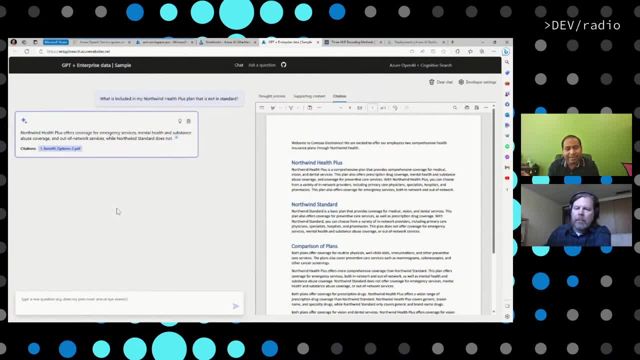 altogether. so you cannot tell that where it comes from, whether it comes from a pre-trained data which comes from the fine-tuned data. no, you cannot do that. i mean, as for my knowledge, you cannot, but maybe in the future. then something came up and this is the way you can do that. but as for my knowledge, today you cannot do that and that's. 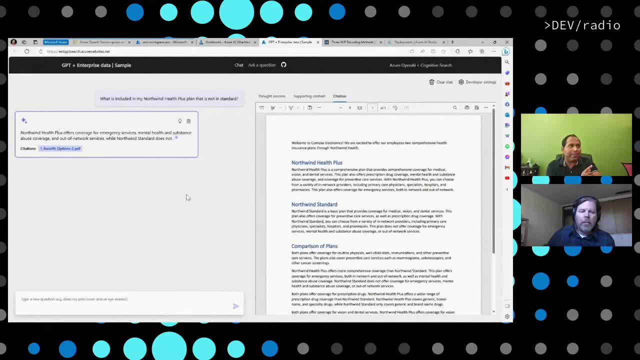 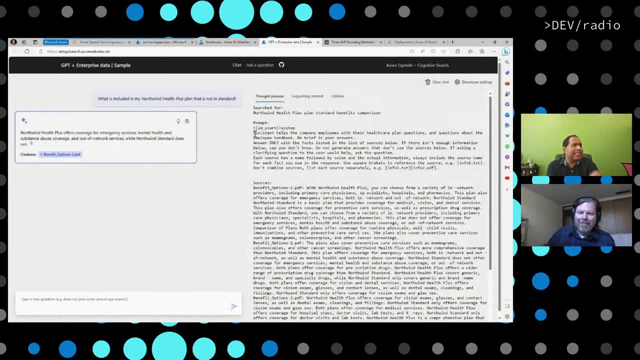 why the rag approach is much more better because you can cite it where it is coming from. that's number one. now, it also gives some sort of thought process. i'll not go deep on that, uh, and say that, okay, this is actually your meta prompt, is your system prompt, and that these are the source chunks. 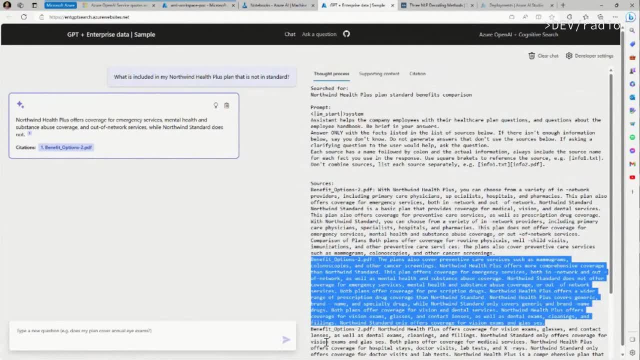 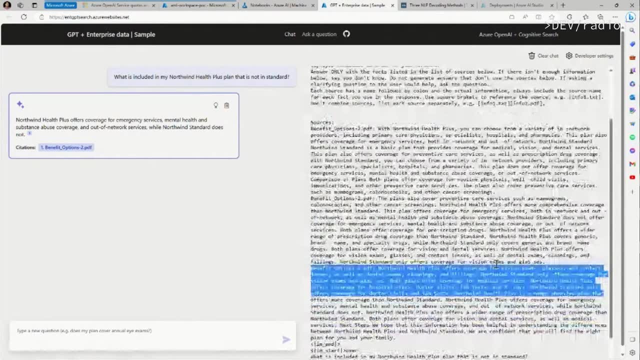 one. there is a second chat and this is the third chunk and that's where it's coming from right and in this chunk is feeding to the actual. you know this chance comes out of the. your cognitive search, feed, backup and open eye gives back the actual answer. 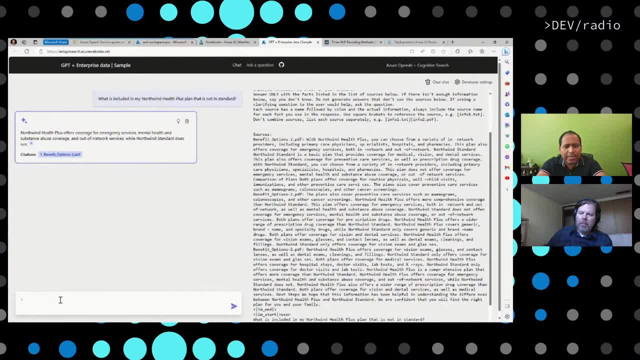 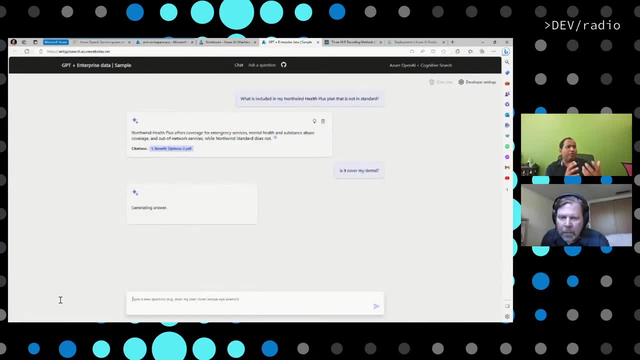 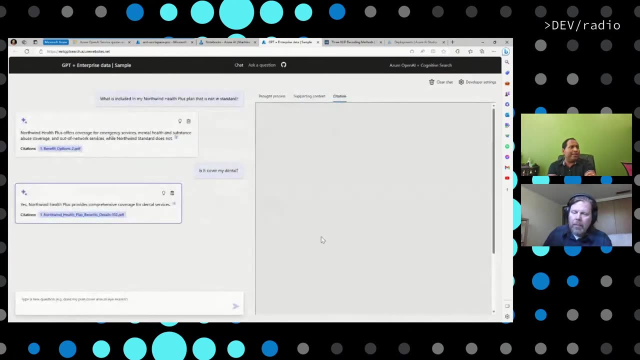 now if i ask a very follow-up question: uh, is it, is it cover my dental, right? so it's a pure conversation and that can say: yes, not real plans provide that dental. now you see that it's giving me all together a different source of documents, right? you see, the previous source of document was: 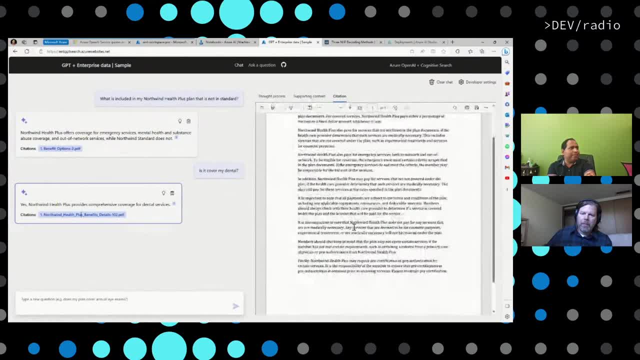 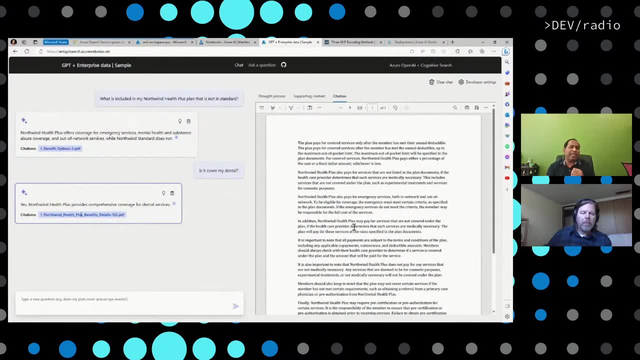 different. now this question, if i ask, is: give me a total different, different document. so this kind of a luxury and flexibility you will have if you use a rag approach and if you chat your own data. so that's what i want to say about the rag and i'm gonna quickly switch my uh terminal to a 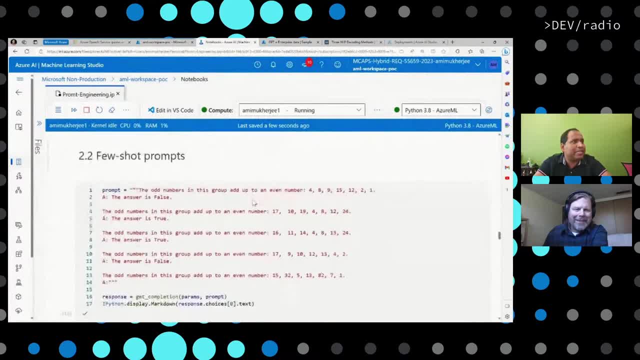 demo, because i promise i'm gonna give you a couple of demos on the different techniques which i've talked about. but before i go to the different techniques, on that i hope is it clear about the rack, why it is important, why people sometimes think that you know, fine tuning is. 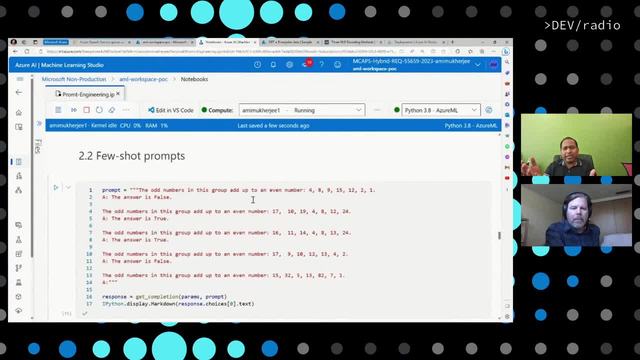 the best approach to go and where you may not need fine tuning at the first time. rather, you can use this approach to come up to your own reason. is that? does that make sense? yeah, it makes a lot of sense and it's. it's pretty clear why you would use it and it's. 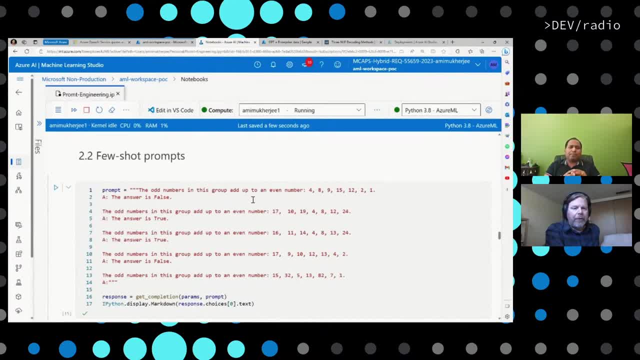 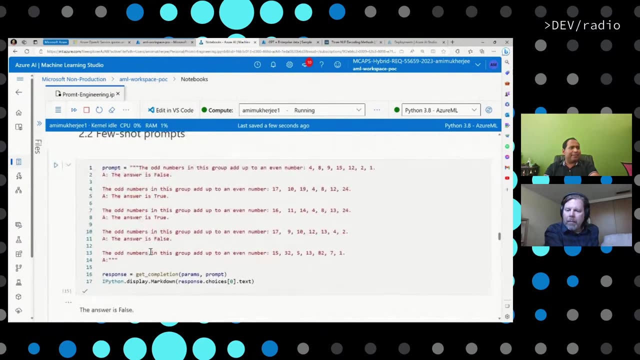 um more valuable than than fine tuning in practical cases. yeah, yeah, great, yeah, awesome. so we talked about the other techniques in the before slides, so a couple of quick, you know demos on that. so, for example, here the same example which i provide, right, and if i ask that in fact all 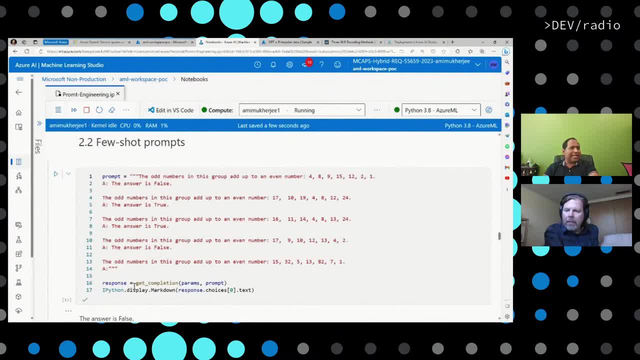 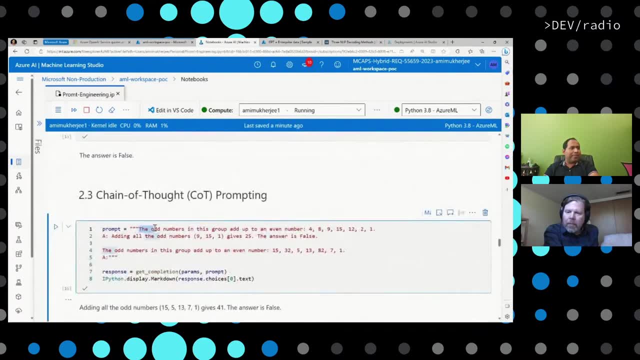 the things i ran before. um, if i run that one, it tells me this answer is false. right same thing, uh, in a channel of thought, right, i have the um, the prompt, right, and in that case that, uh, all of this group at the event number. if i ask that question, uh, which is, which is basically um, give me that the answer is: 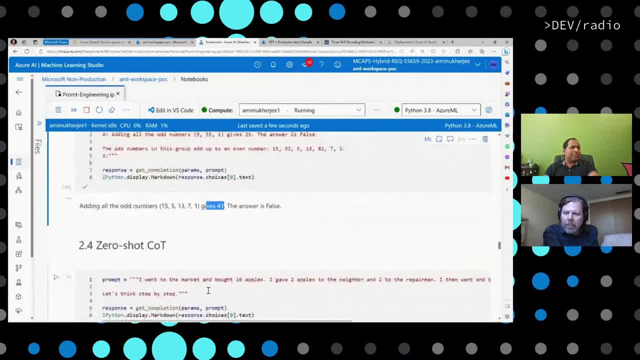 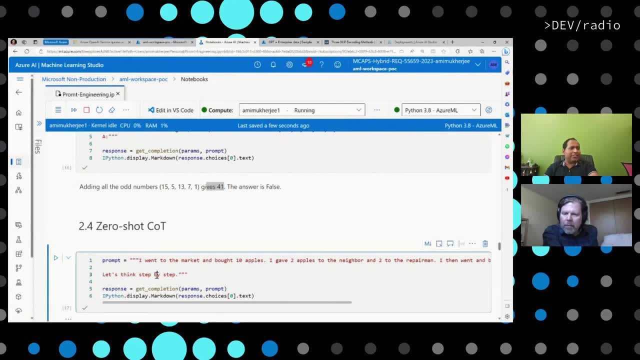 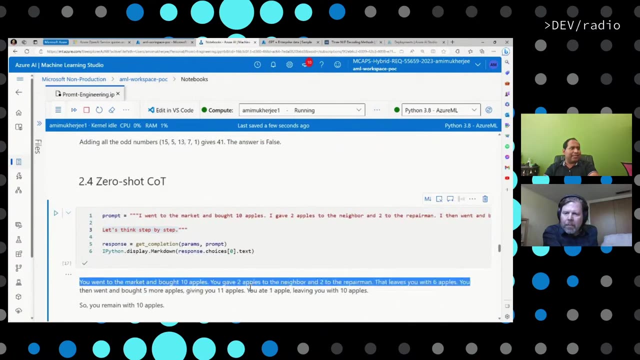 false, which is giving the 41 right. this chain of thought now zero sort cot. when i'm adding a less thing step by step, i go to the same example and i added a, added just a step here. let's think step by step. and once i get that one, it gives me a very precise uh thinking, step behind the scene and give. 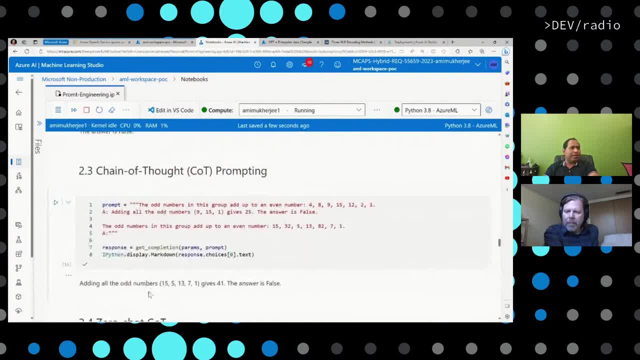 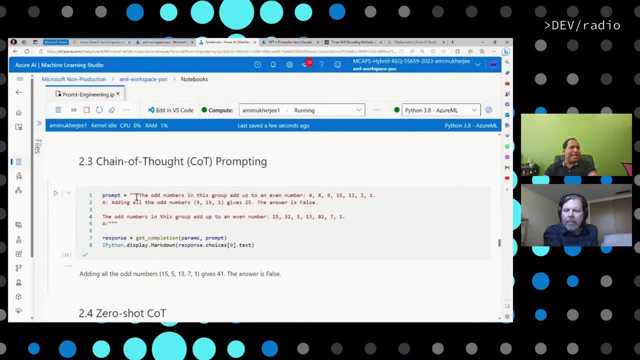 me the actual answer, when, in this case, regular chain of thought, it does not provide me um any sort of- you know, exam detail explanations, but i do provide an example, right, in this case, this one, my actual question, this is my actual answer, right, i put an example and then i'm asking: 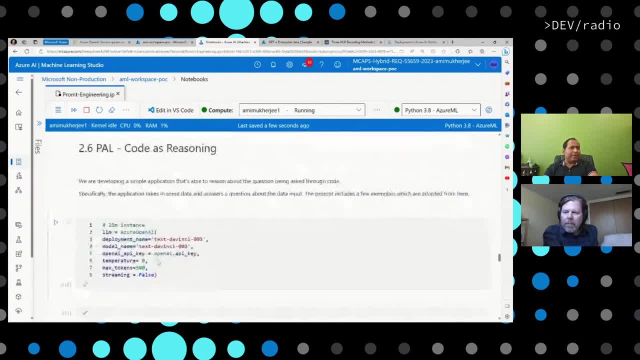 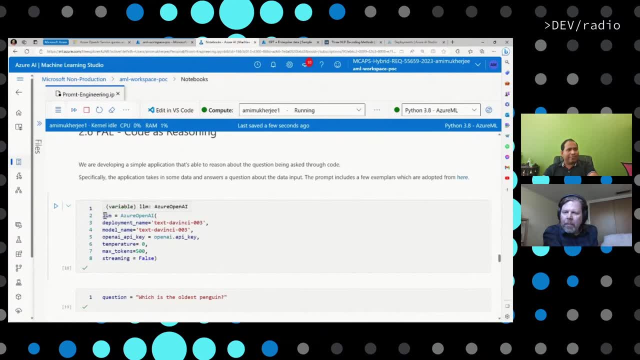 the question, i'm giving the answer. that's, uh, that's kind of a channel of thought, right. so i thought now, pal, which is, which is i thought you might be interested to see, that one, this one is, i'll provide that define, a large language model, uh, the define that you know the instance of it. 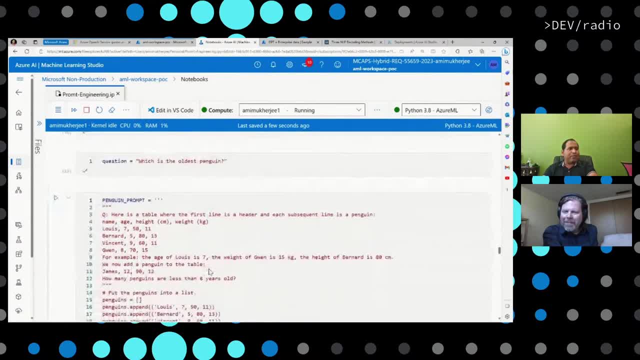 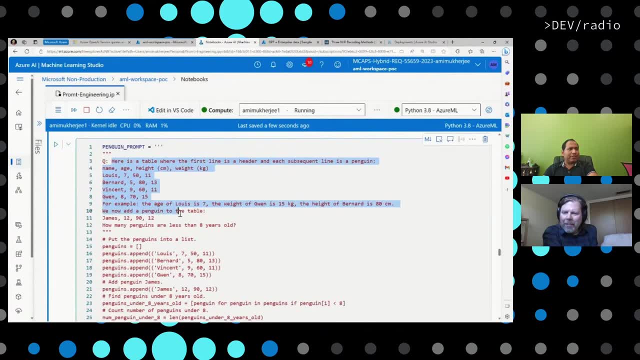 and then i ask you which is the oldest penguin right? and the penguin prompt is: is pretty much like this right. i provided a detailed question on that. i'm sorry you're saying something, man. no, no, no, keep going, keep going, i'm just following you. yeah, then, how many penguins are less than eight? 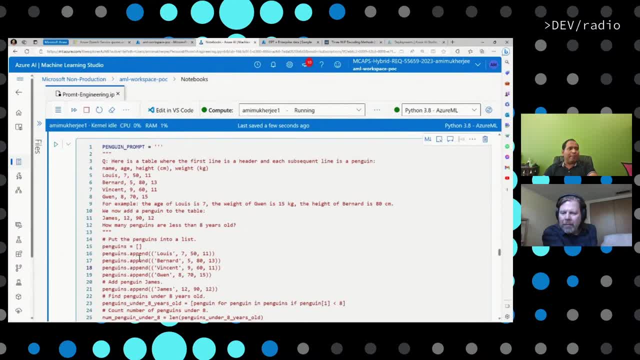 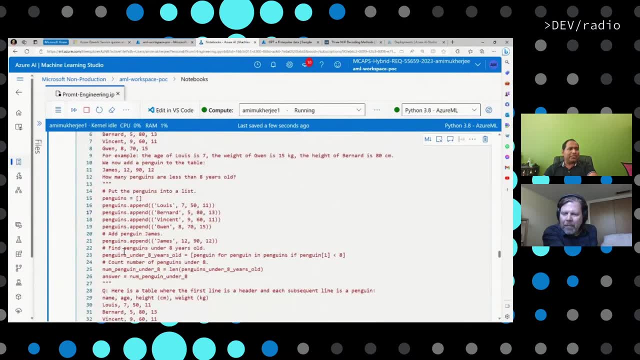 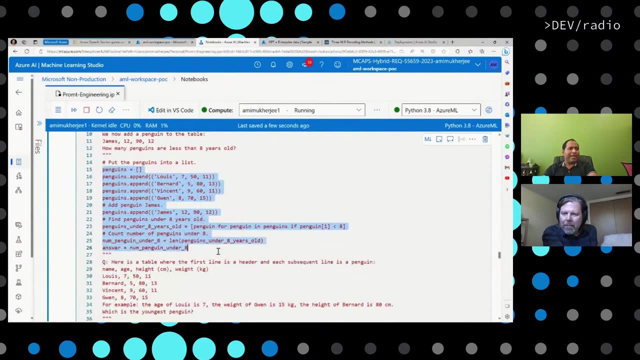 four, then put that in a pythonic, you know format. so i put in the python list here and then append all of the penguins details then and i append the another one, the james, and give the file answer. so this pythonic interprter which i'm providing here, it can be used to come up to the actual, actual. there's many, many examples. 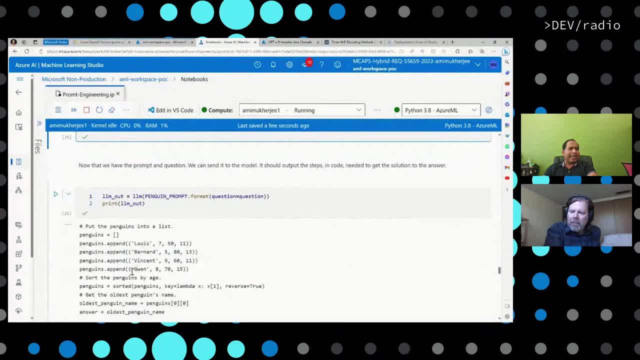 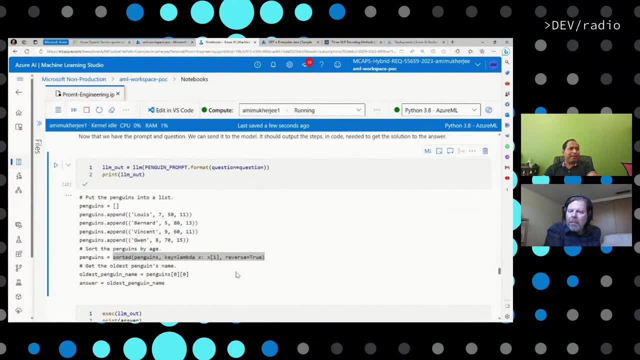 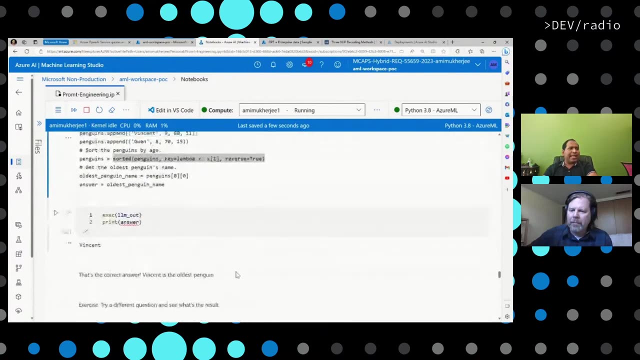 then i come to the actualism right. so when i run through that it goes to that actual, you'll see examples. it used the pythonic- you know nature insert of Lambda functions it uses to come to actual conclusions. right now you might be thinking that, hey, how do I do this python? 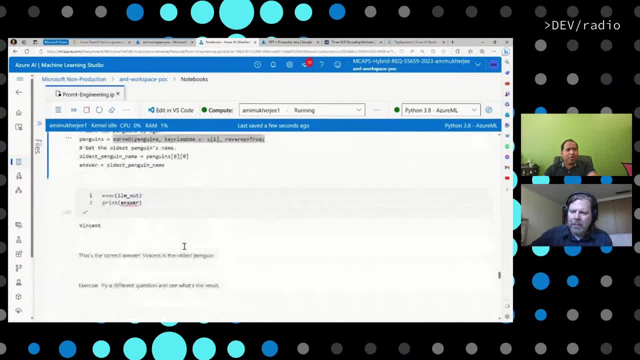 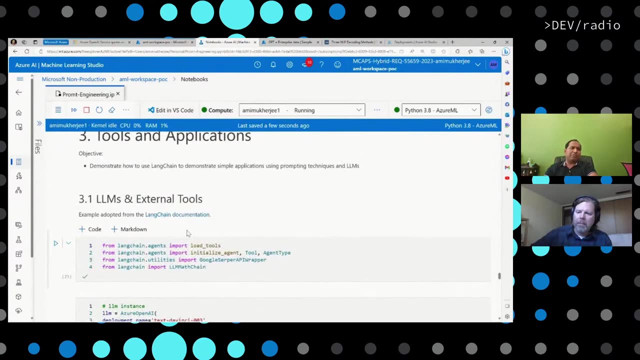 equals. should I have to write my python code? and all of that not necessarily always, because there are some tools are available which is called langchain, and langchain has the python repple, the tools which you can use to do the offload, the calculation to the repple, and they 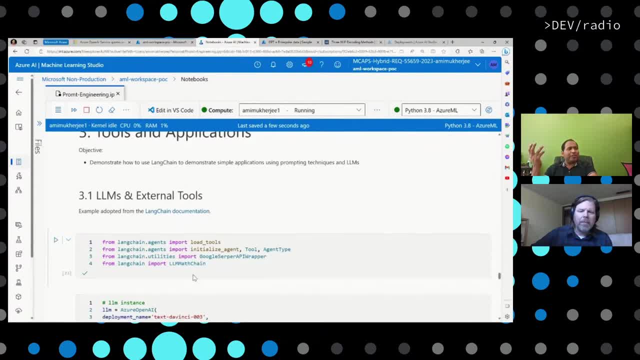 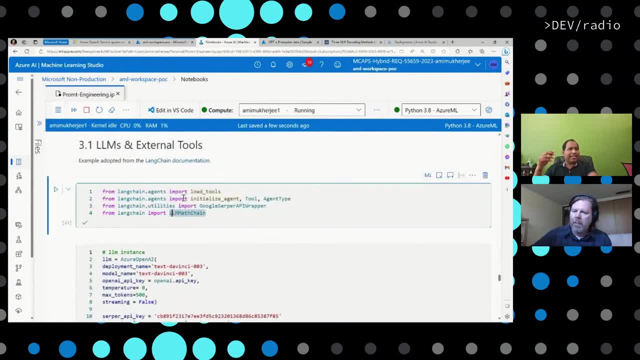 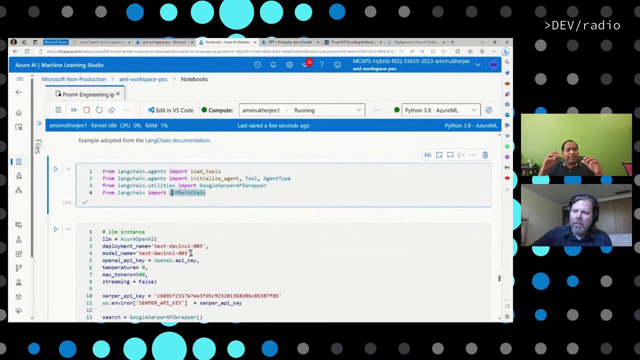 can use from there. I also talk about the external knowledge generations and all that, for example. in this case, right you, I use a langchain here and I said that I'm going to use an agent here and I'm going to use some sort of tools here. right, and, by the way, in a rag approach also. 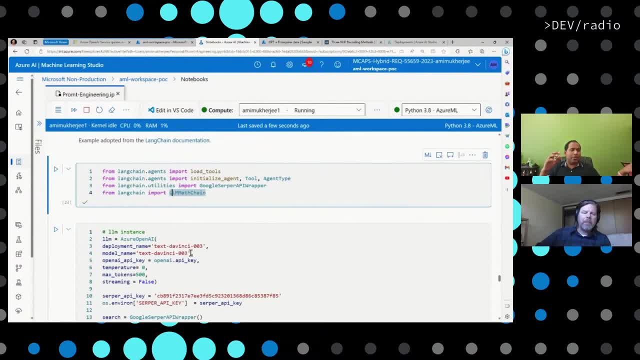 it not necessarily always has to. data has to come from your knowledge store. it can come from external sources as well. so, as you know, the OpenAI GPT model has been trained on the public data till, I believe, September 2021, right. so it doesn't have any any knowledge after beyond that cut. 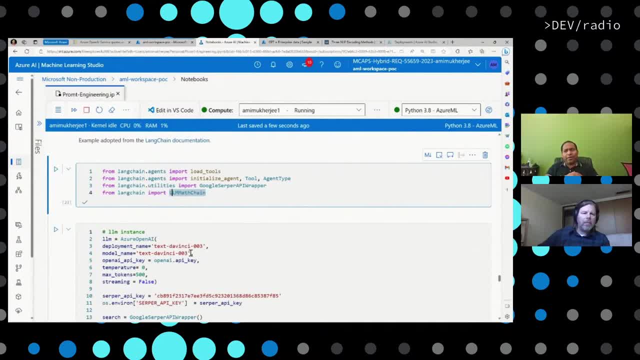 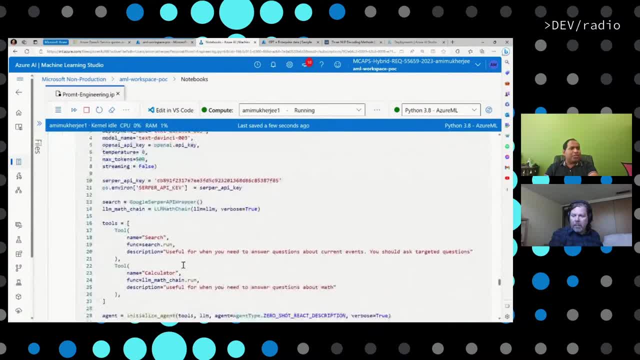 and that's where it's going to be, and that's where it's going to be and that's where it's going to be. so, for example, in this case I have defined two tools- one is a search tool and one is a calculator tool- and I'm telling that this search tool is responsible if I ask very targeted, uh question. 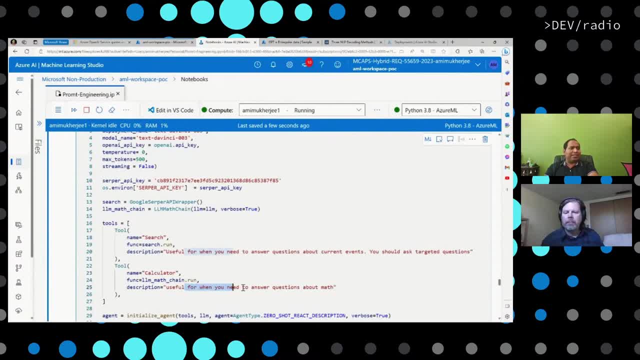 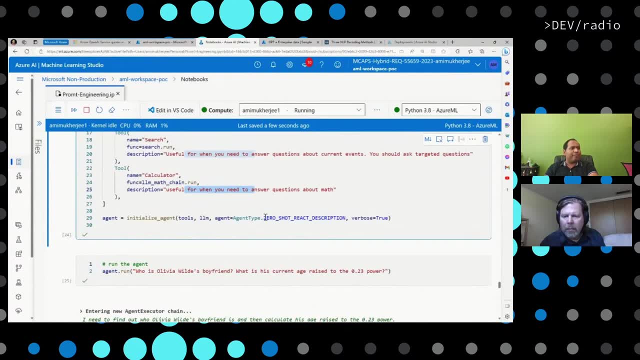 on the current events and this tool will be responsible for some sort of math related question. right then, I use a geosort react. that's what's talking about, the react. so in the agent you define the react from a launching. and then I'm asking who is Olivia's boyfriend and what is his current age? 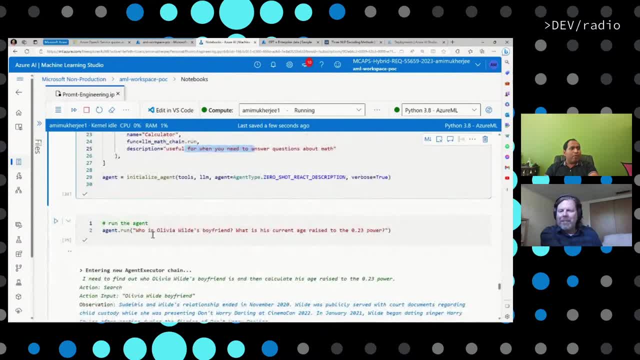 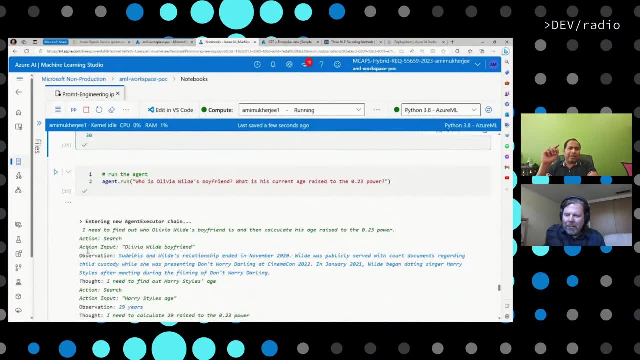 raised uh to the 0.23 power, right. so now Olivia's wills the boyfriend first. what it does is, if you see, that is action and that's all uh reason over. um, react is uh reason over observation. the act, right reason and act is coming here. so first input is: first they need to find Olivia's boyfriend. but 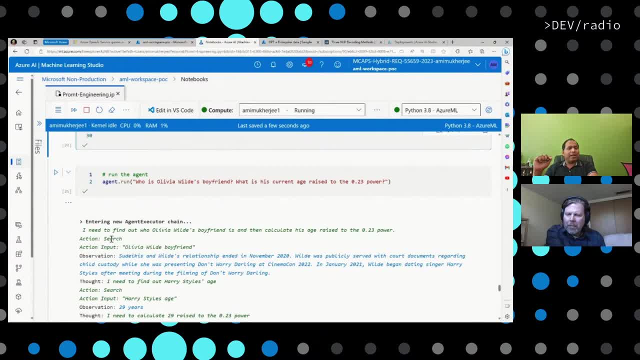 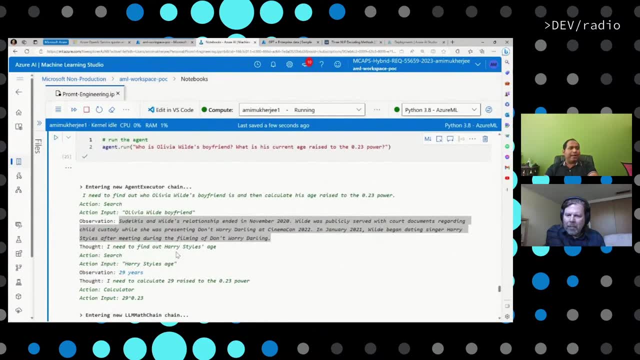 that the action is taking. it is searching from the internet. it's not going to the the pre-trained data and the observation is comes from us, from internet. is this one? then he said, okay, then I need to find uh this particular guy's, uh the Harry's age. right, then again you go for a search and it's. 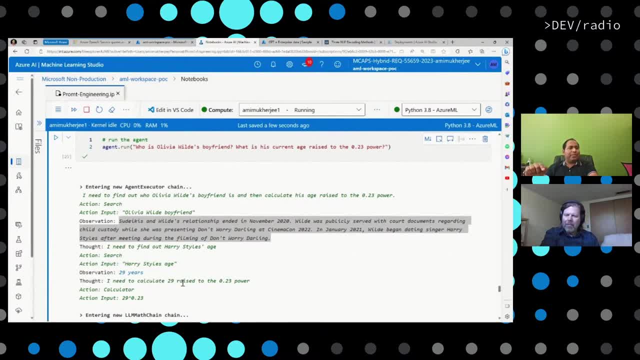 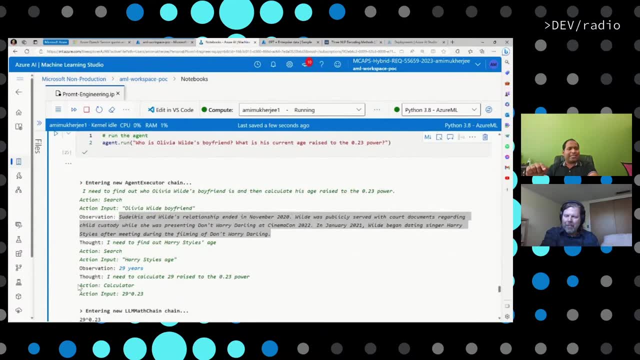 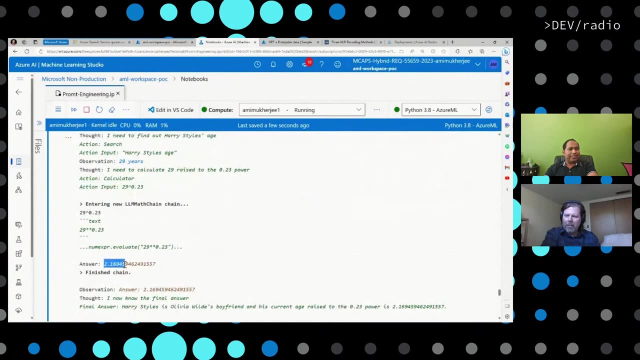 come the Harry's age is 29 years, then you need to calculate the 20 and to basically increase that age to some 0.23 power. right, then use a different action that's called calculator and then use that action to raise that and it's coming up to the final conclusion that this is my final answer. 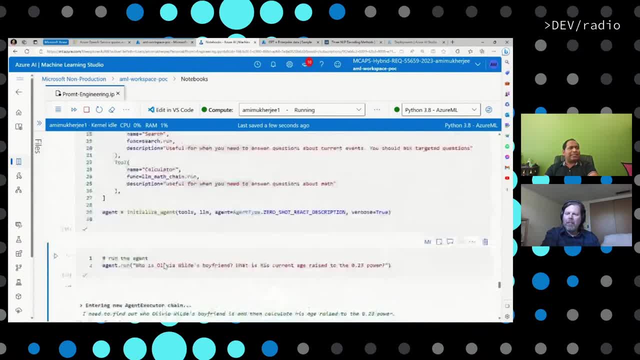 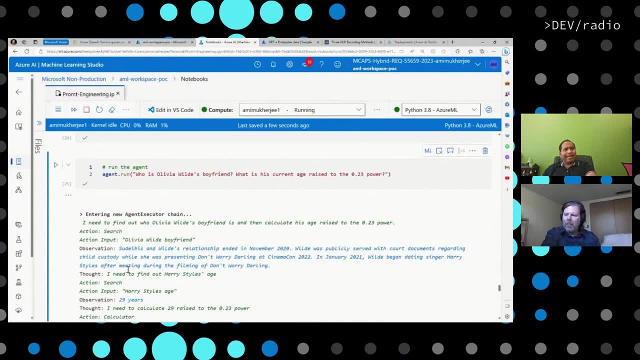 so you see that in a one example I just asked this uh question and behind the scene it goes. a react kind of an approach goes over at search. you can get the result and when you do the search it's basically use rag by the way at the same time. right, because 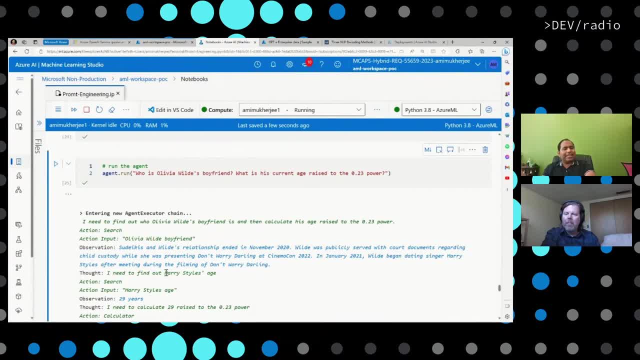 you're feeding that information from our different sources. then you search- okay, this is the observation I got. next thought is: find the age of the harry and get the find the age of the harry, the another search and then, okay, now I got the final age. then you got to that. the another tool which I use, the calculator, then you, you который car, you go, and then you're, you're there when you get to step 1 of the question: what is making a point x, tok, or it is characteristic, and kra vieler, whatever you're doing. and then you are finding to know, you know not that. 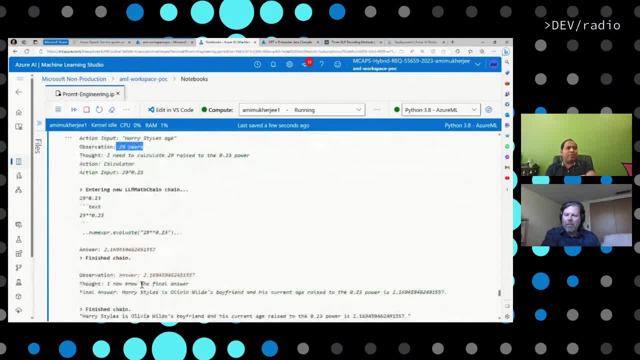 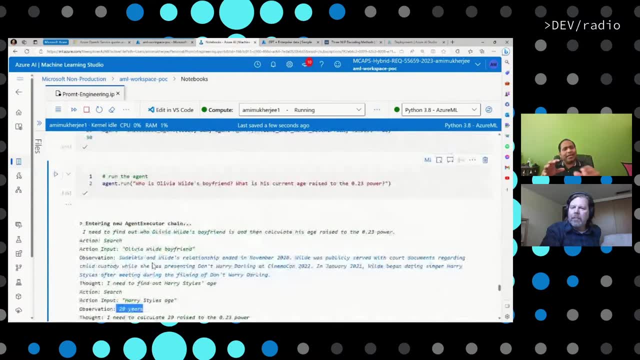 or this is the result. what is happening to this calculation is whether it is more likely the calculator to, to you know, do some map and give you the final results. right, that's, that's pretty much. it's called um react, uh with agent, uh with the rack, everything all combined together, right? 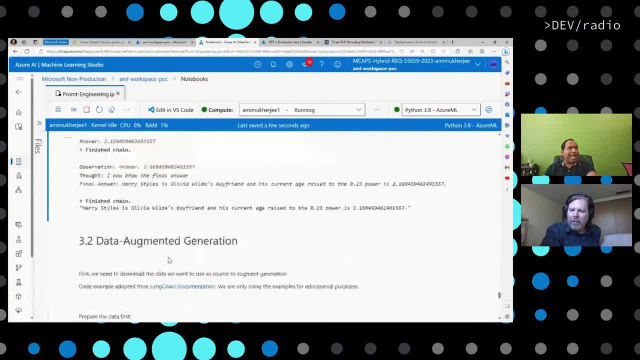 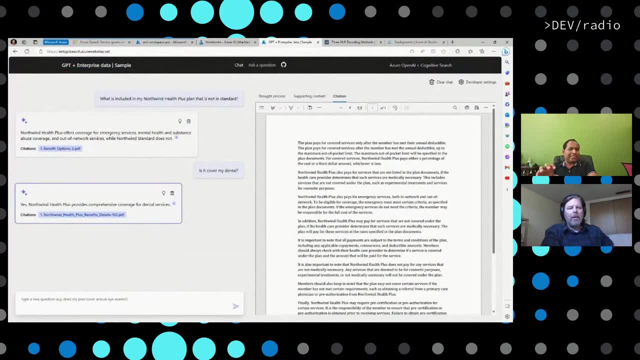 and um this one i already demonstrated before, which is called actual rack, which is this example, to citate the data. that's pretty much i have for the demo. i hope this makes sense. if not, reach out to me. i can go give you more detailed explanation on that. um so long story short to write a. 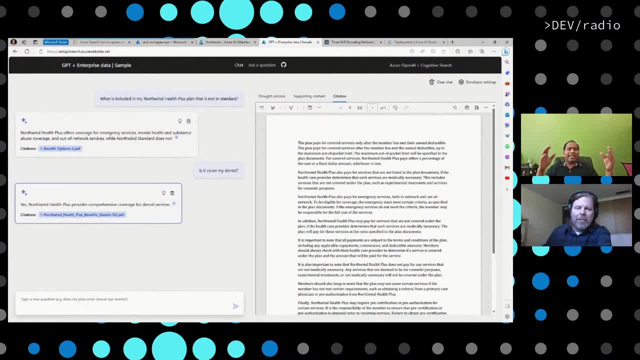 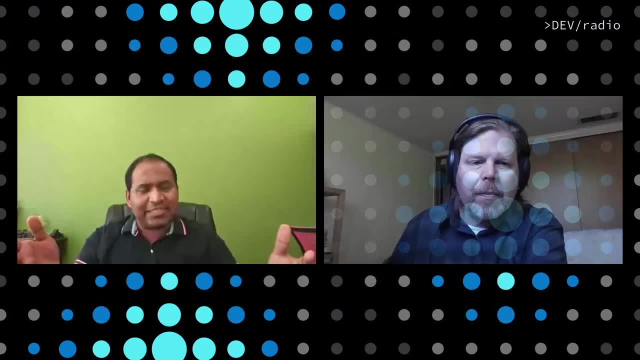 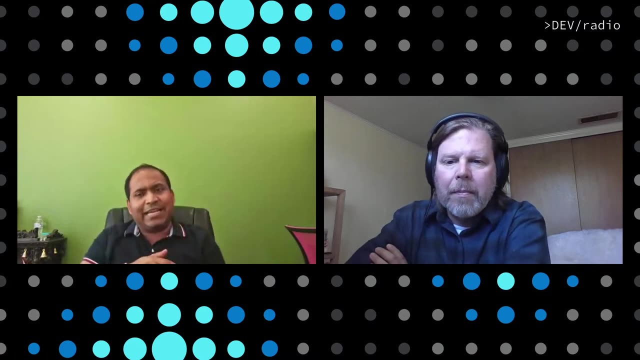 prompt, better prompt. there are. the different tips and techniques are there. these are not all, but these are some of that which is very popular and most of the customer are using these techniques to write a better prompt. that's one right and, with all of these approaches and tactics, i'm sure you 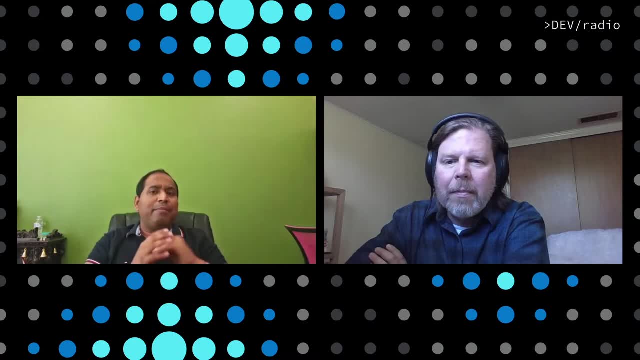 able to write a better prompting in your applications. but remember one thing: as we write the better prompt, you also need to think about prompt safety. right, there are a lot of uh like: uh, prompt injection jail breaking, right, um, the prompt leaking. there are different uh the prompt related the safety features unity. 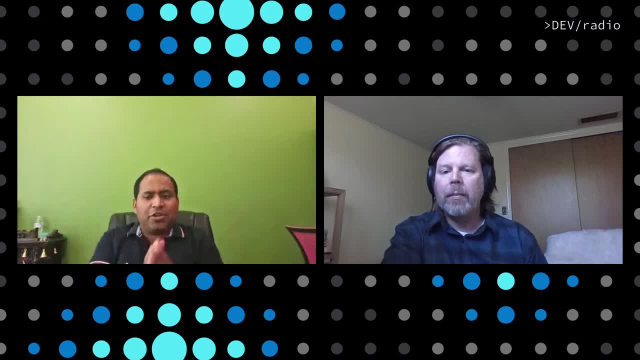 employ which can save your prompt right, which is not part of the topic today, which might be i'm going to record a other session on the prompt safety. you need to think about that as well. right, how it can safeguard your prompt prompt engine is a definitely one of the aspects. but prompt. 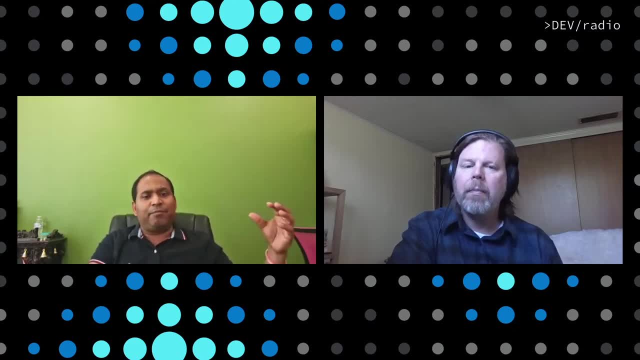 safety. at the same time is very important for the enterprises to safeguard the prompt so that somebody cannot hijack that prompt to inject some their own prompt. or somebody should not steal the meta prompt, which is actually the system prompt, and inject something different. right? so all these things you need to think about before you think about how to build a large 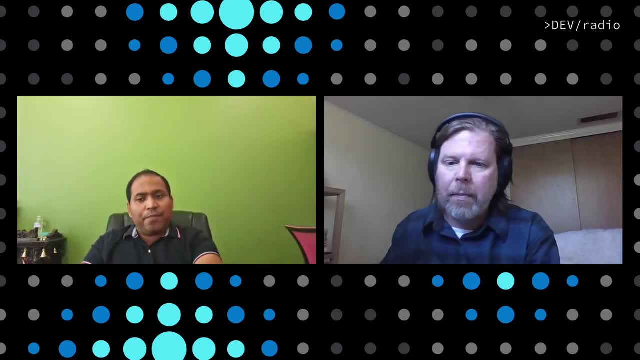 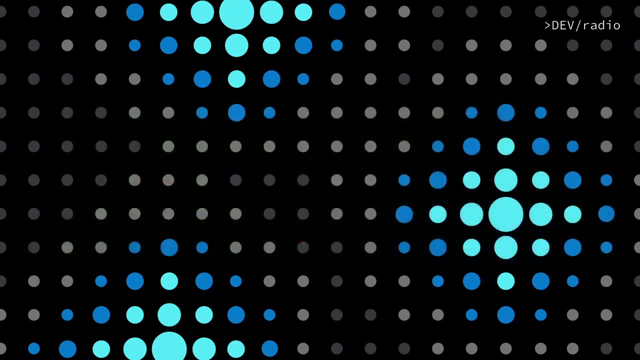 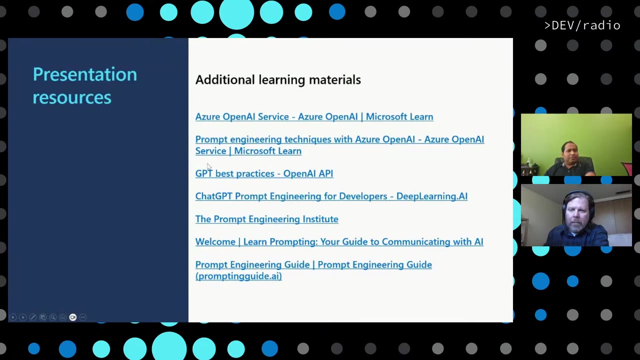 language model applications and get you to a production. so that's all i have and i'm gonna leave with a couple of, you know, additional slides here, which, uh, which basically talks about, uh, the learning materials for you and what are the best you know, the, the prompting techniques. 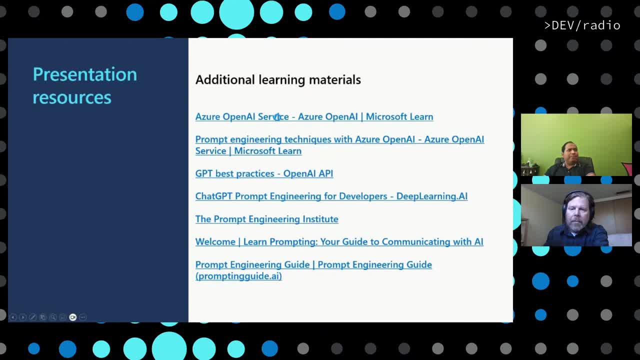 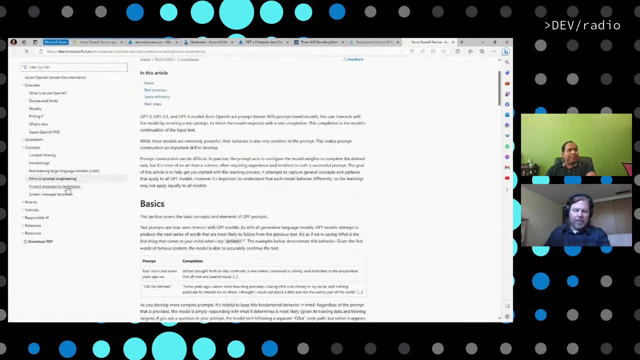 like we do have in microsoft. if you click on that link, it will be reached outside to uh uh page, which talks about the prompt engineering and the different prompt teaching techniques and all of that. this is a really good one. uh, in fact, open ai also came out. 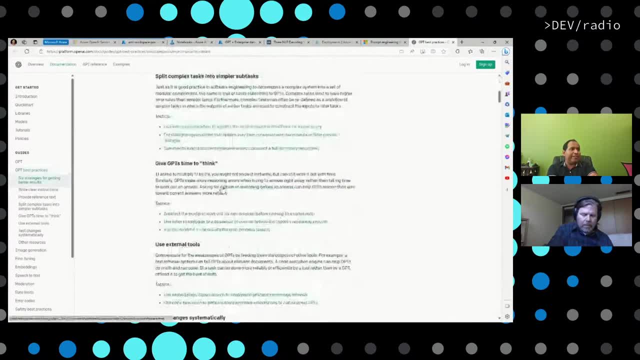 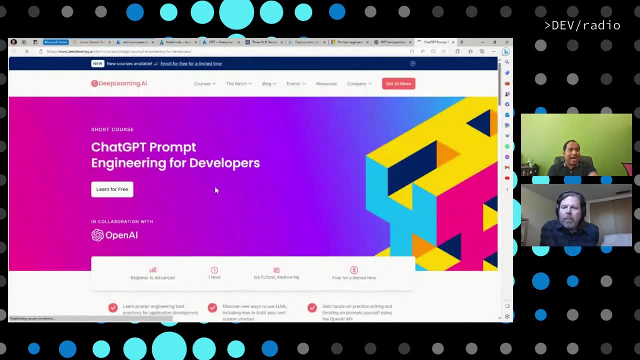 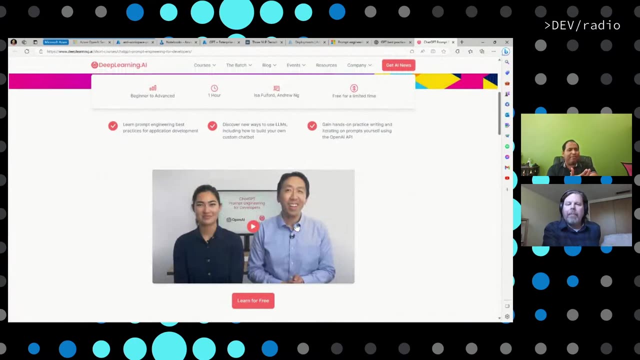 of- uh- i think it's pretty new- the best practices for prompt engineering. you can employ that one as well. um, third one is a prompt engineering for developers: deeplearningai. i highly recommend this is a the course, the deep learning ai taught by the android, who everybody knows. it is a part. 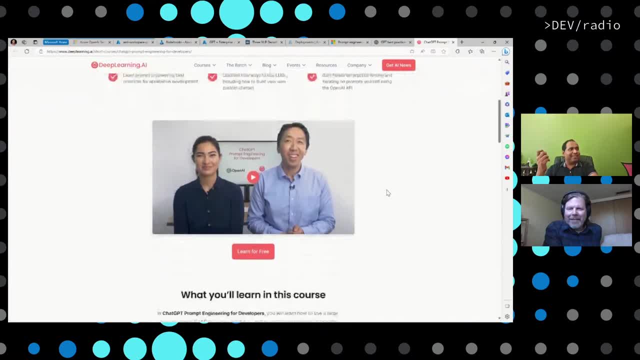 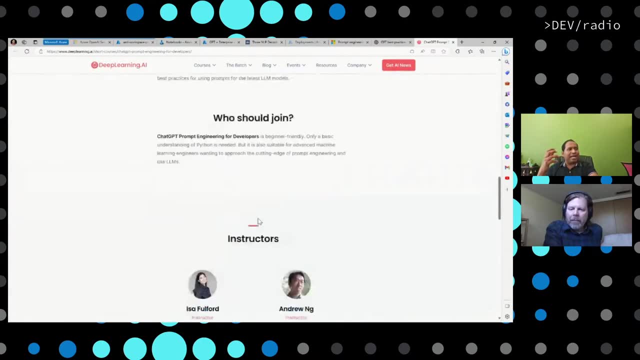 of you know the, the, the deep learning and the machine learning, and it also open ai um version. i think our name is isha, so isha and andrew has been talked to a different prompting technique. in fact, in my presentation, which i use, i use some of their techniques to present you. 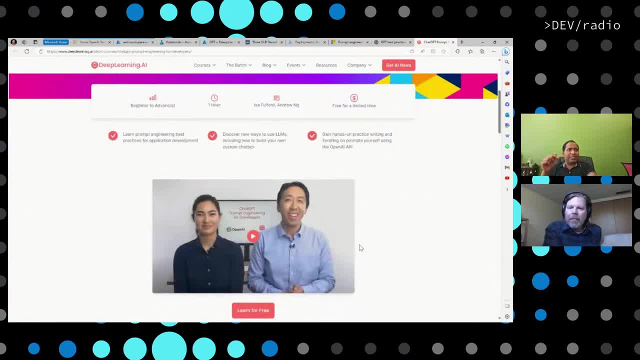 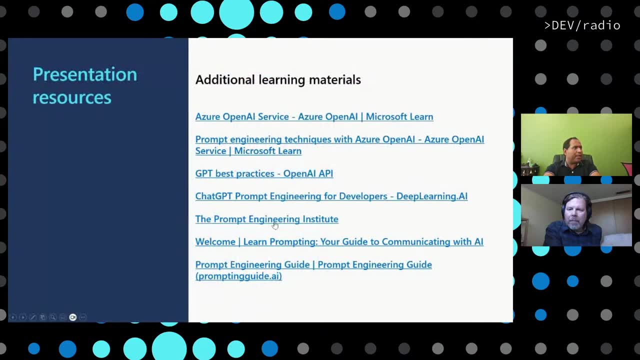 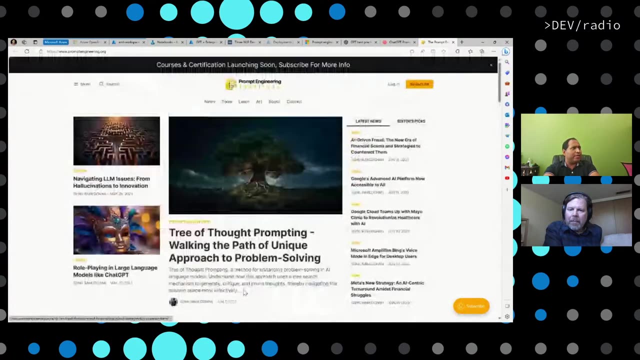 so that you can get the first hand what looks like. highly recommend that pretty valuable information on that as well. right um. third one is um. um is a prompt institution institute. this is also you can get some current details- what's going on in the world in terms of the prompt. 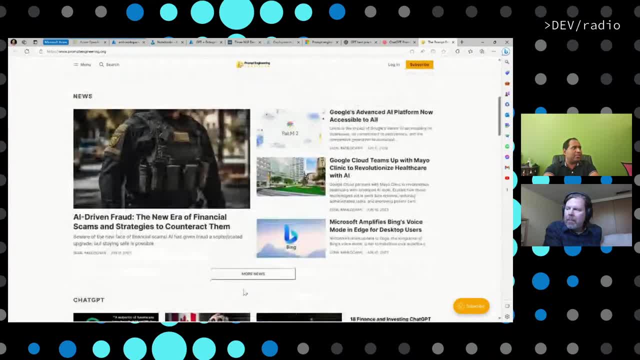 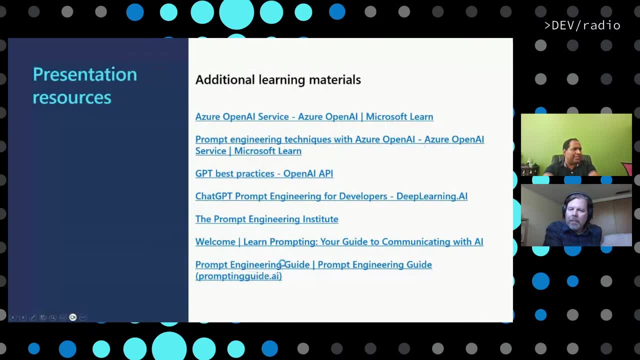 engineering, how the enterprises, as the industry is going, different tips and techniques. you can follow this. this one that's really helpful. um, you have another one, prompt engine guide. uh, that's also very important. you can get a lot of prompting technique. in fact, some of the examples which i 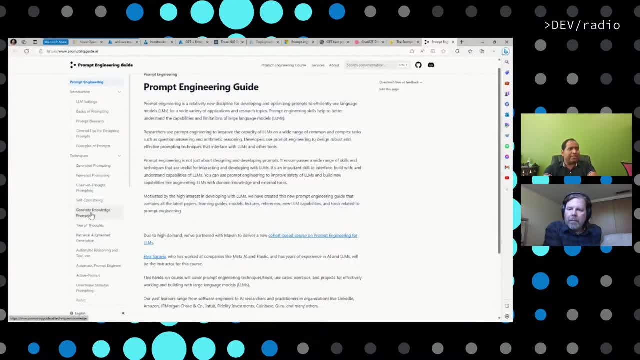 take it, i take it from here itself, which is called self-constraint generating power. knowledge tree of thoughts. it's pretty new, um, it's. it's basically talks about, uh, different thought process and give a given you know ecosystems. it basically gives you the final, final output, rather than just one chain of thought. 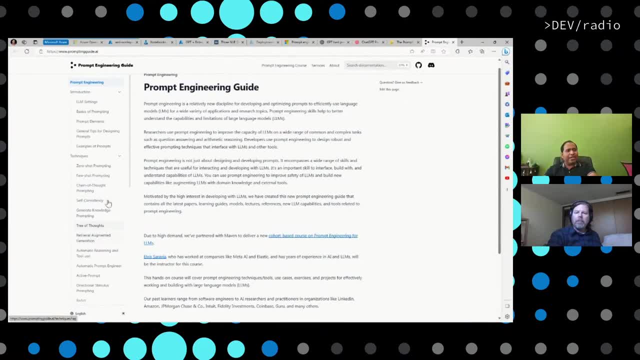 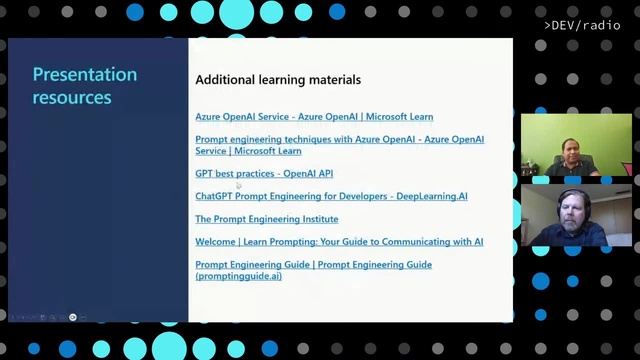 multiple trees of thoughts. it goes through and give you the final results. so there are different techniques. has been mentioned over there. you can go through that, um, and yeah, that's it. so, in fact, these are the learning methods i can recommend. let me know if you have any questions.